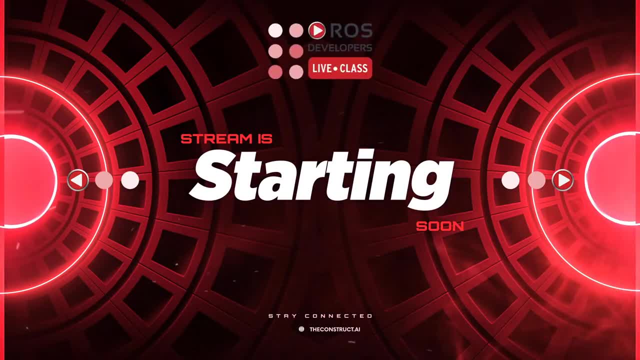 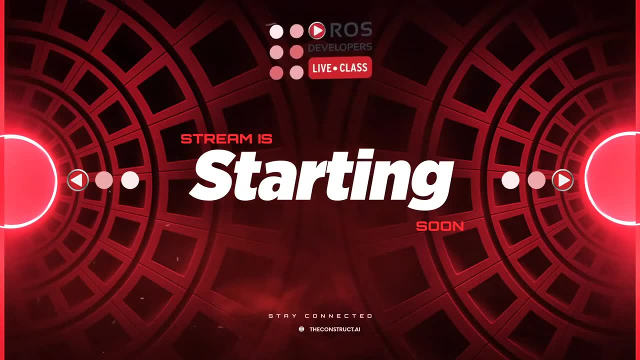 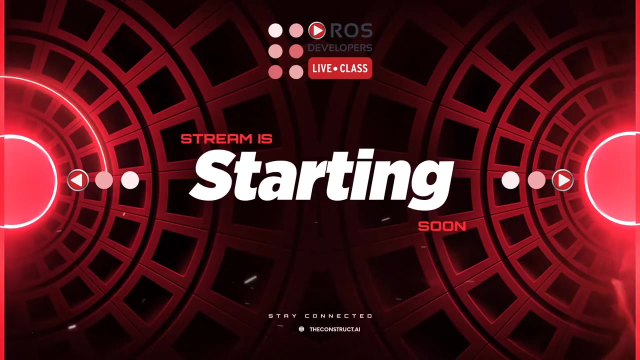 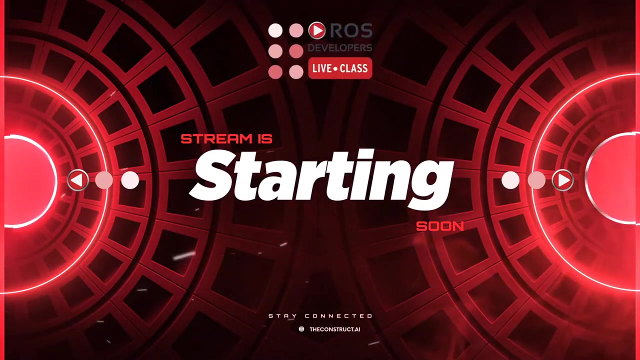 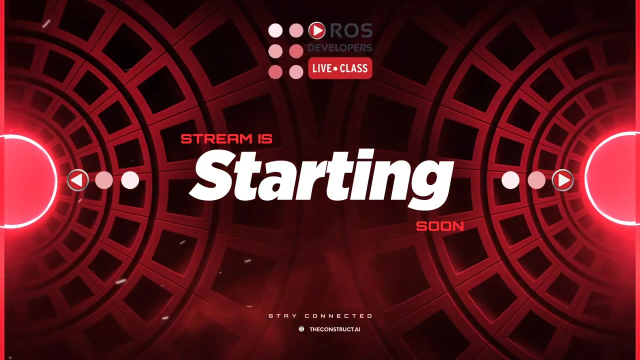 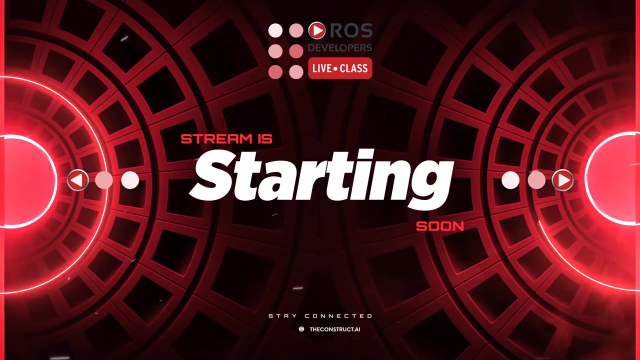 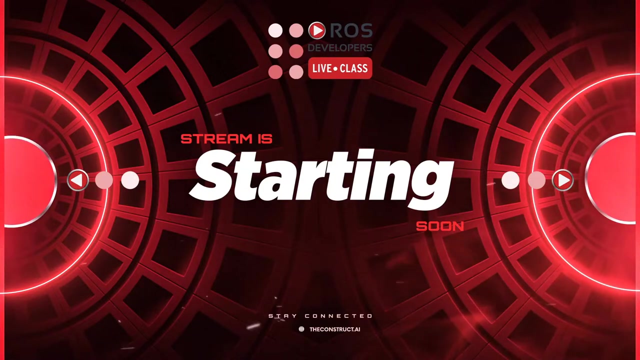 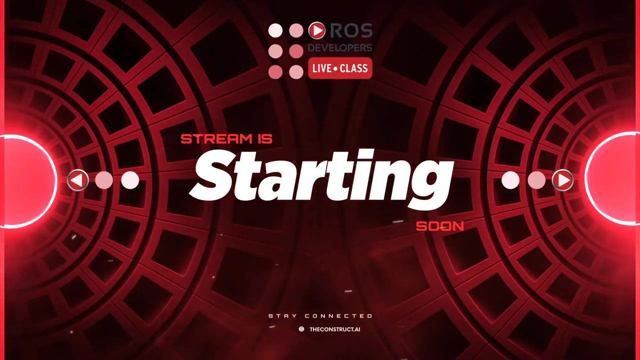 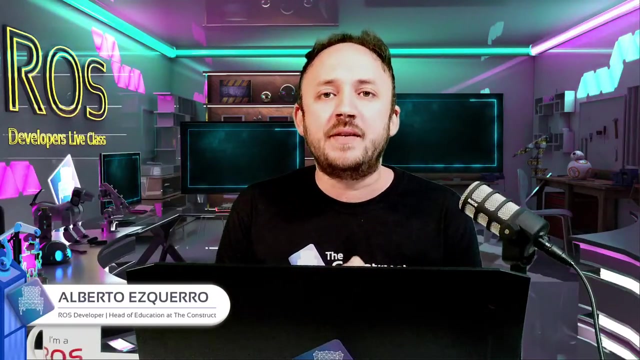 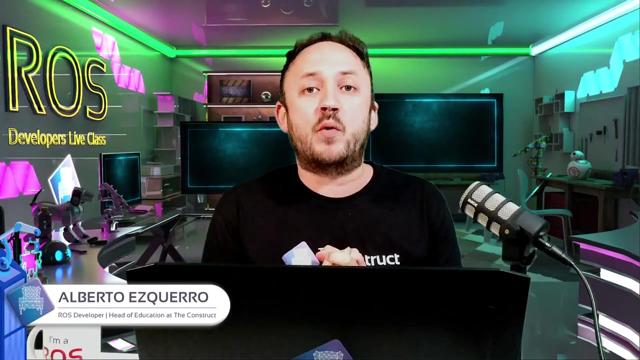 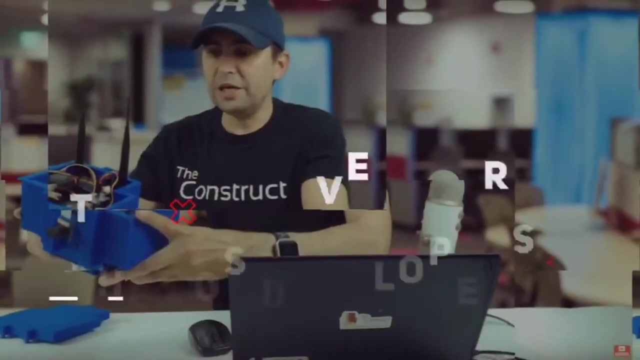 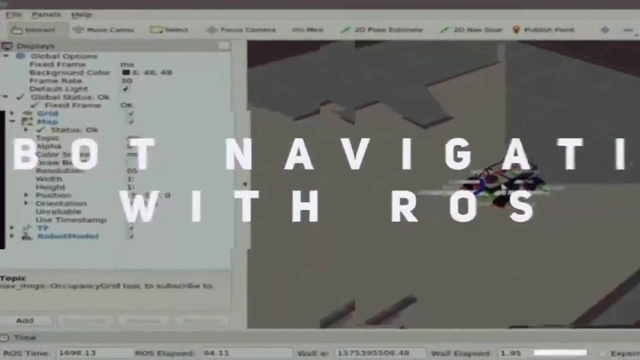 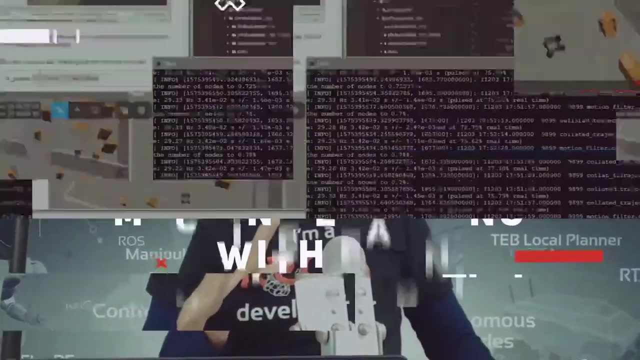 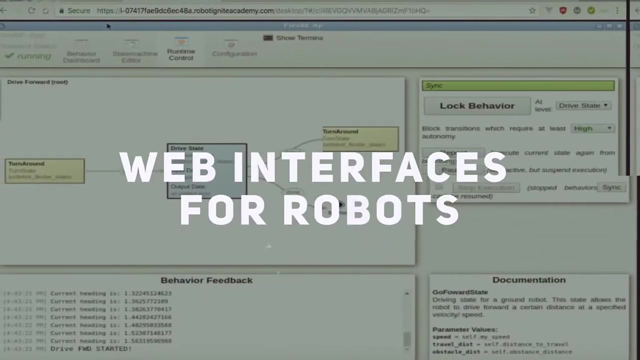 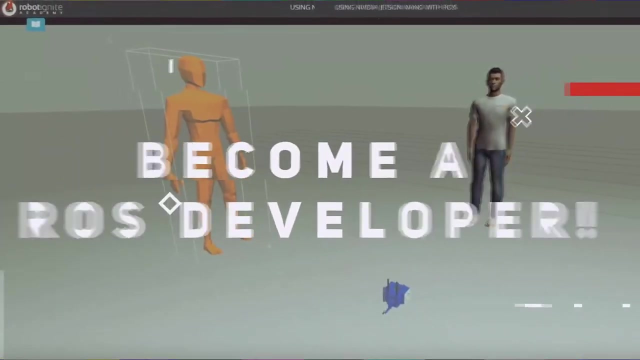 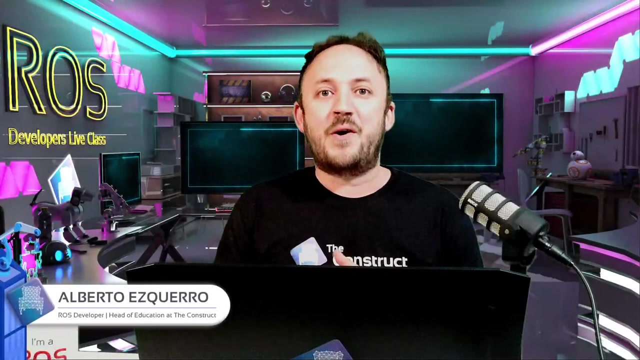 Thank you. Thank you Where we are going to be working with a robot manipulator, with a real robot manipulator, and performing some ROS manipulation with it. So let's go for it, All right. So hello there, ROS developers. 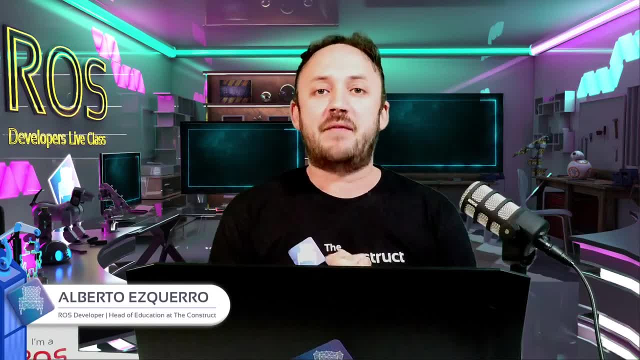 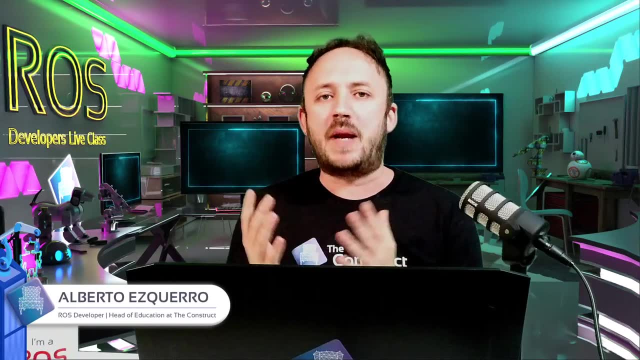 Welcome everybody to this new live class. As I have just said, today we are going to be working with a robot manipulator And we are going to be performing some trajectories with it, Some motion planning, And we are going to be working first with a simulation, with a simulated version of this manipulator. 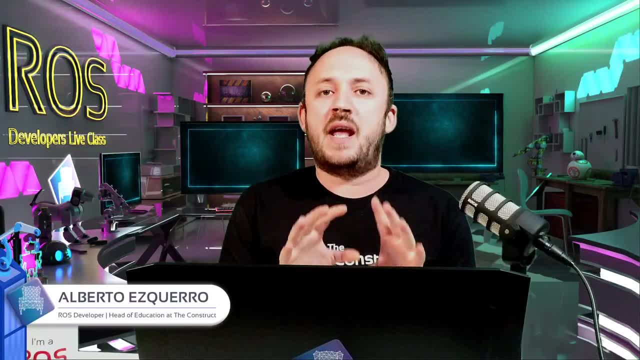 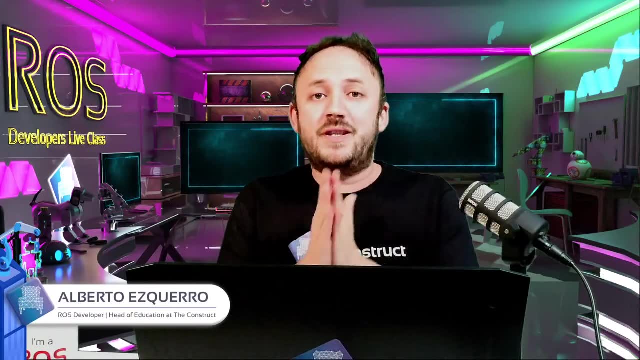 And then we are going to move the code we have executed in the simulation and we are going to execute it into a real robot. The same code. So this is the goal for today. Then let's not lose any more time and let's go for it. 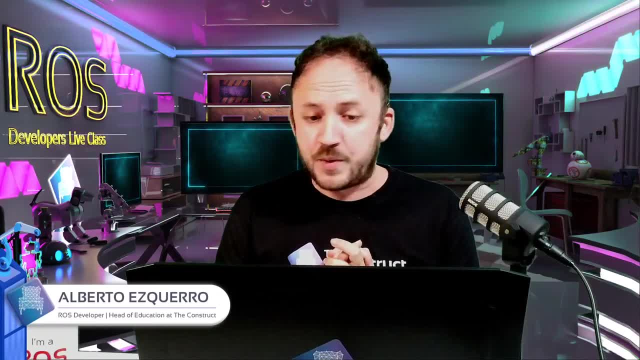 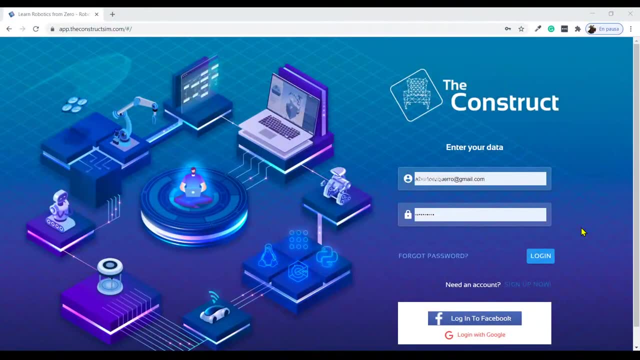 So I'm going to switch right now to my computer screen and I'm going to start the live class. So let me do it right now. There we go. So, as always, we are going to be working on the construct. 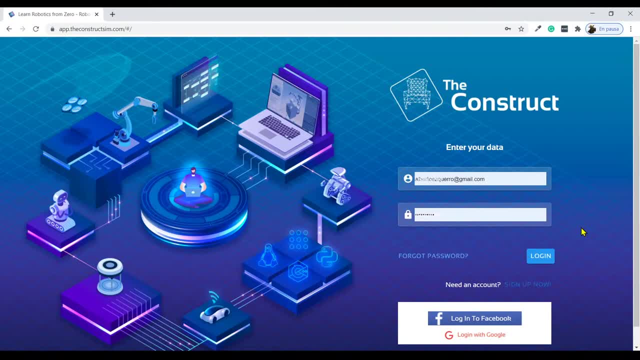 So all of you log in. The ones who already have an account For the new ones, just create a new account. It's completely free. It's going to take you just a few seconds, So go for it, Then we are going to log in. 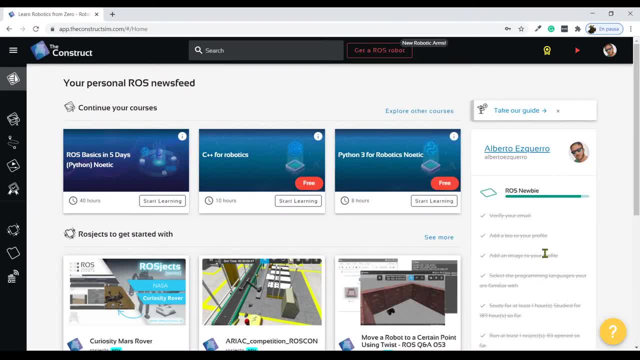 And now, in order to access the live class, today's live class, you are going to have to come here to the left menu. If you come, If you move your mouse here into the left, this left area, you are going to see this menu. 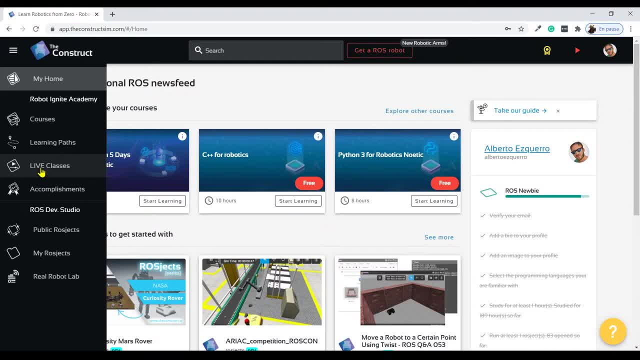 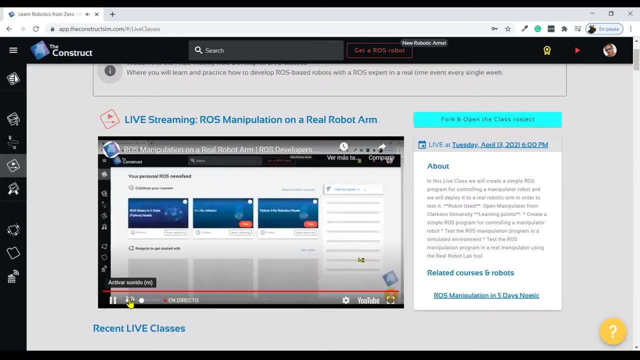 And we are going to come to the live classes option. You are going to click on this option and this is going to show us the current live class, This live class that we are currently streaming. So this is the actual, the current live stream. 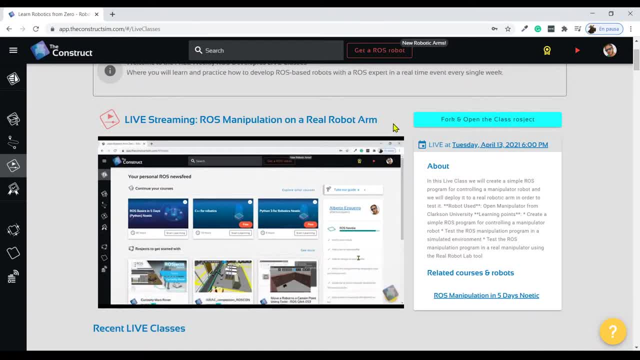 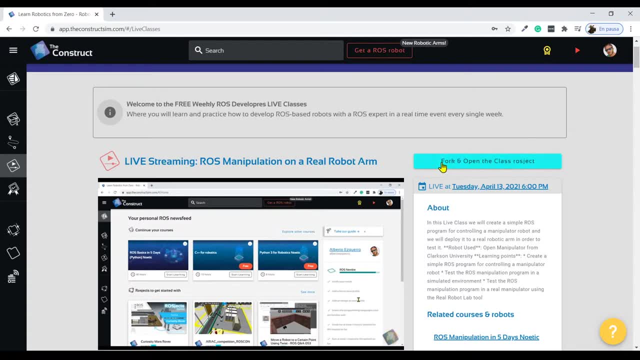 And then here you can see the video, And here in the upper right corner you are going to see this light blue button which says fork and open the class project. So everybody, you have to click on this link. This is going to automatically copy and open today's project. 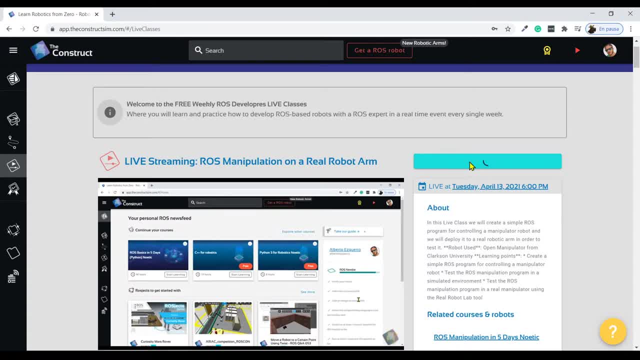 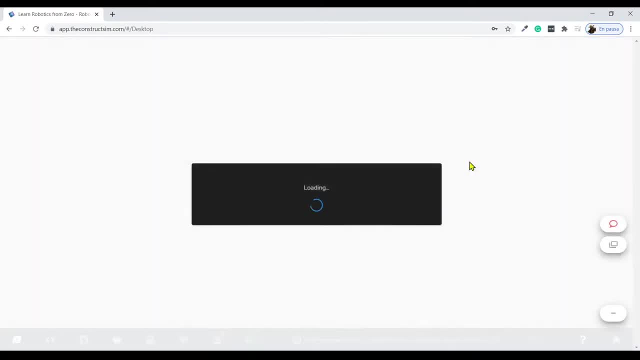 So let me do it myself. I'm going to click here on the button And this is going to automatically copy the project into my workspace, into my account, And it's going to automatically open, as you can see. Let me make sure. 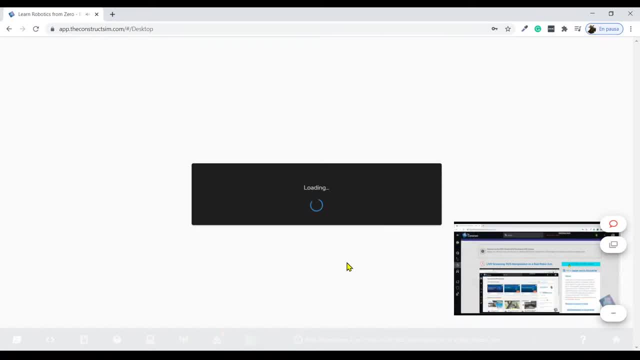 Let me make sure, Let me make sure. Let me minimize this also. And now we are in the main screen of our project, So we are going to. you are going to see, here, in the lower right corner, here you can see the live streaming. 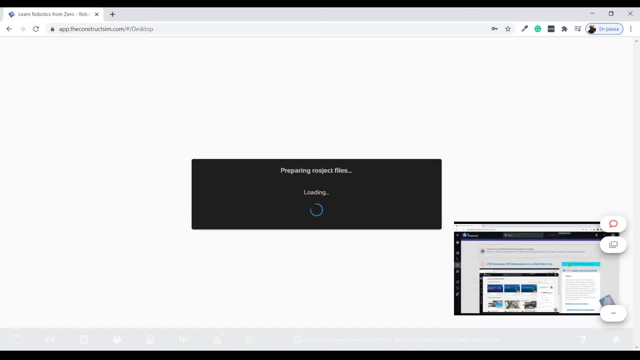 So you are going to be able to follow what I am doing here, And also you can activate the chat by clicking on this button, which I am going to do right now, to see what you are saying. I am here myself, though. 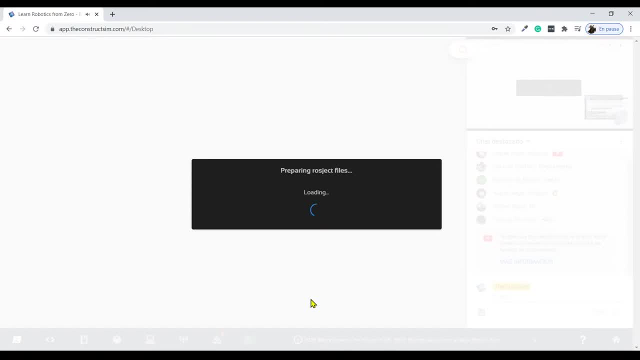 Now let me wait a second so that I can mute myself. So hello, hello. I can see there Miguel Engineering Nations. as always, William, Enjoya Thomas-Peyrushian. hello everybody. all right, so meanwhile my Roject is getting loaded. 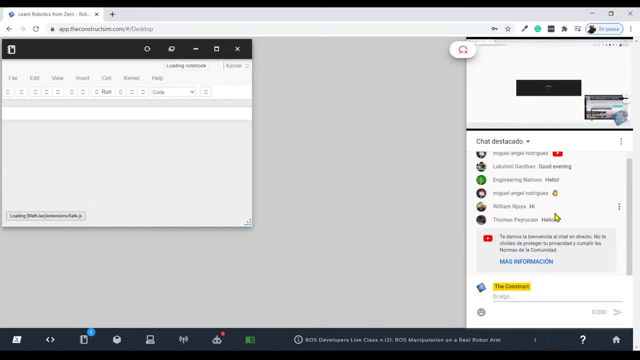 let me, there we go, let me mute this. let me know, by the way, in the chat here for a moment, if everything is fine. I suppose it is, because otherwise you would be here in the chat complaining about it. so I suppose that video is fine, audio is fine. you can hear me. 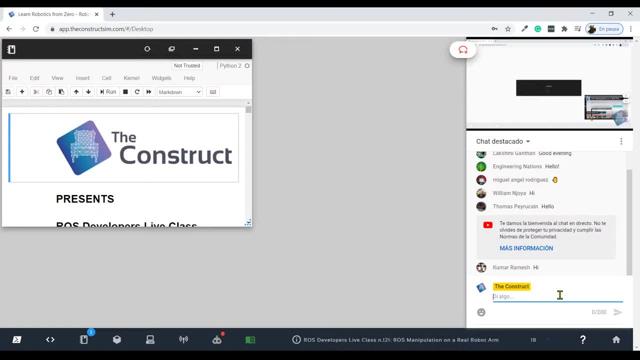 correctly. yeah, let me know here. give me some feedback here in the chat so that I can keep going. hello, hello Kumar, hello Adrián, Adrián Caderno, hello everybody having a hard time finding Roject. so it's engineering nations. what do you mean? 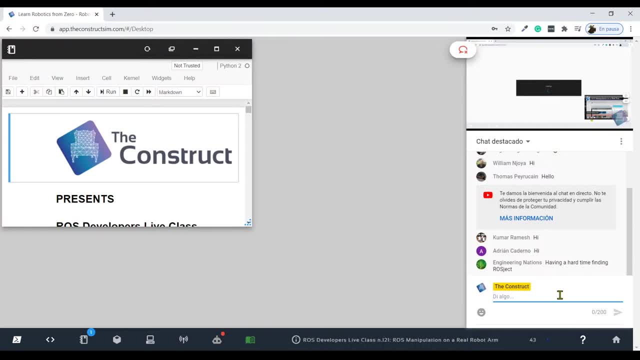 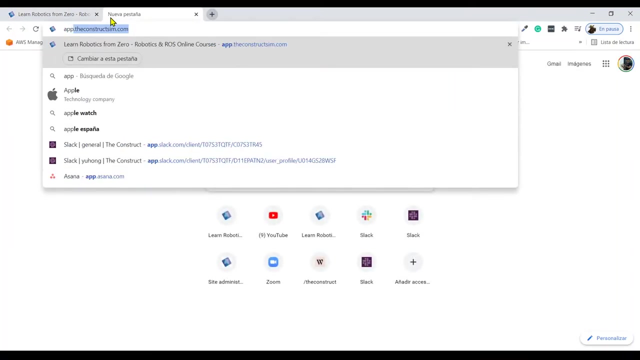 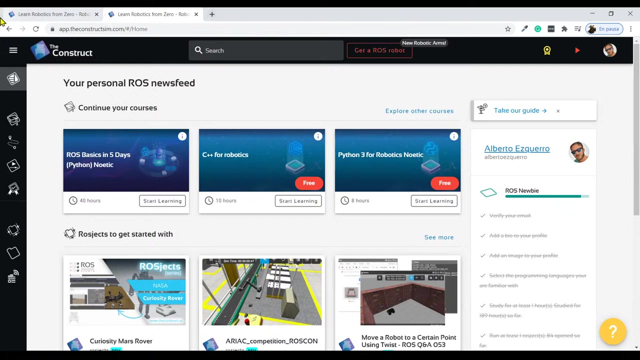 It's in the live classes, in the live classes button. hello everyone, it is fine, says Lucas. video and audio are fine, great, excellent, excellent. let me just remind it one more time, in case somebody has just arrived, so remember you have to log in into the Construct webpage. come here to the left menu. 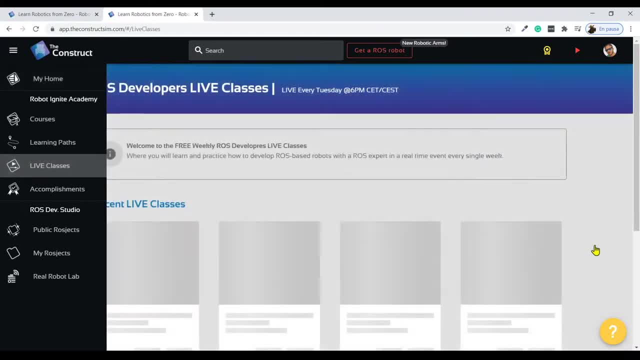 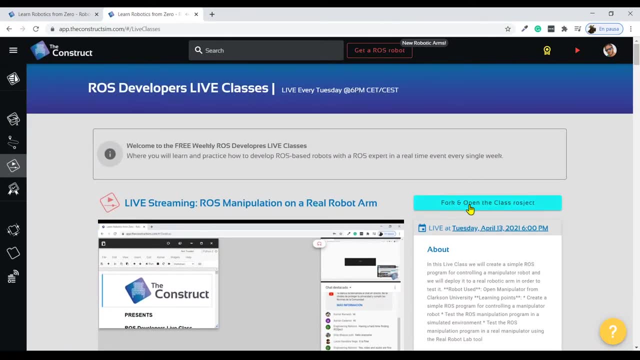 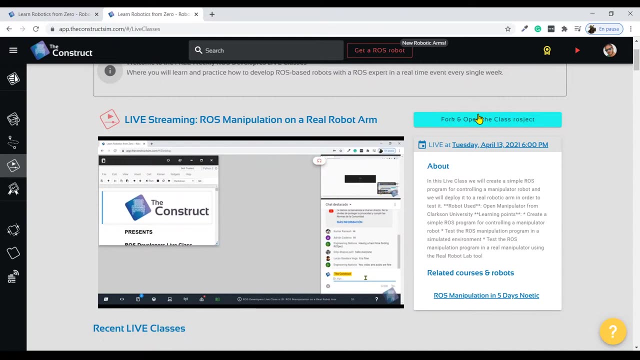 and click on the live classes. okay, and here you are going to see the current live stream, the current live class, and you need to click on this light blue button which is fork and open the class Roject. you click here and this is going to automatically copy and open the Roject for today's live class. all right, 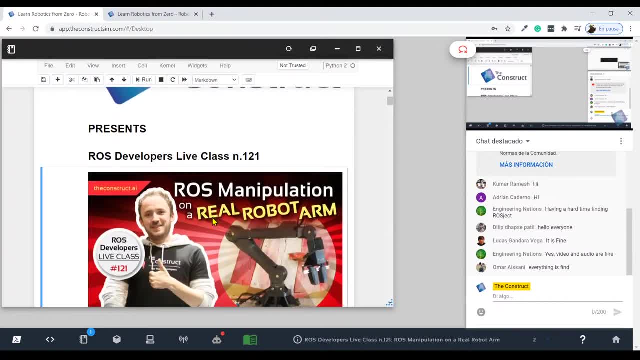 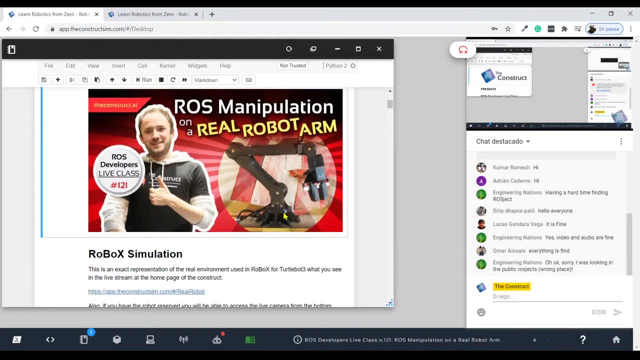 so let's go for it, let me let me. first of all, it is fine, everything is fine, okay, great. so let me just very quickly summarize what we are going to be doing today. so we are going to start first of all by starting our manipulator arm simulation. 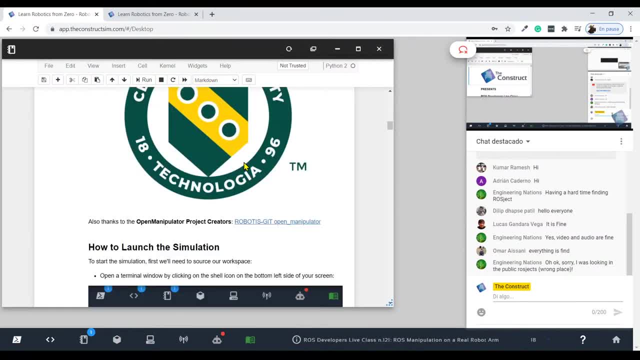 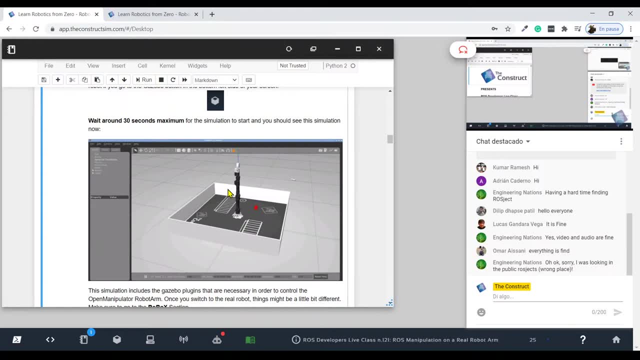 which you are going to see here. this is the real one, by the way down. here we are. you can see the simulated version. so we are going to start launching the Gazebo simulation of our manipulator robot, which is this one. 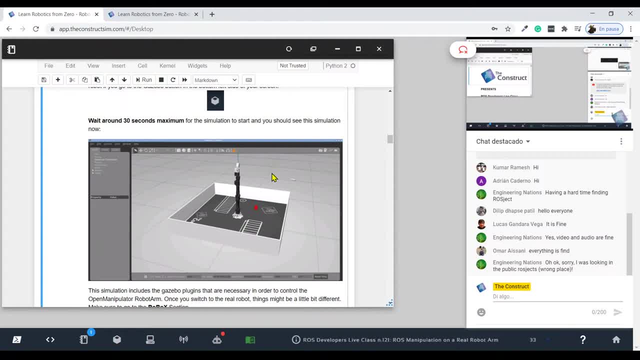 and then we are going to explain some things. I'm going to show you how to move and control the joints of the robot. then we are going to also launch an script in order to move the joints to random positions continuously. we are going to review a little bit this script. 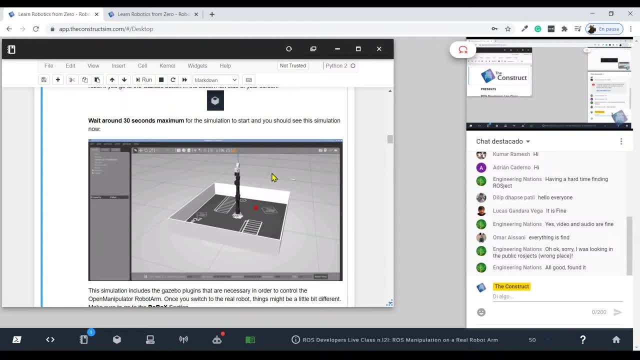 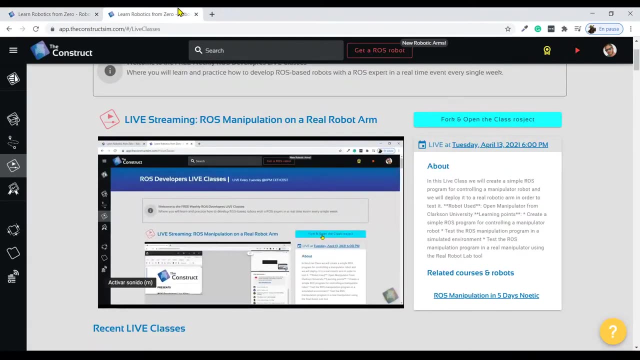 and what this script is doing. and then, once we have tested that everything works fine in the simulation, in the simulated environment, we are going to use the real robot lab in order to connect to the real version of this robot. so in previous live classes we have already 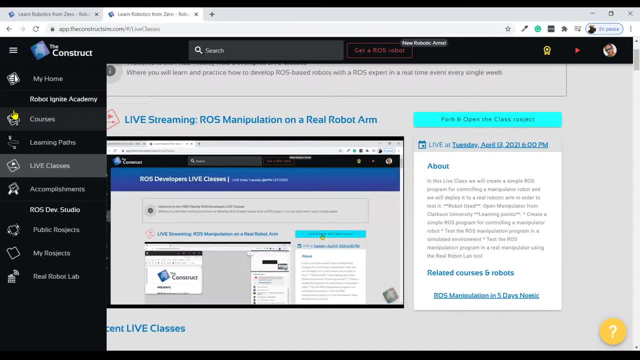 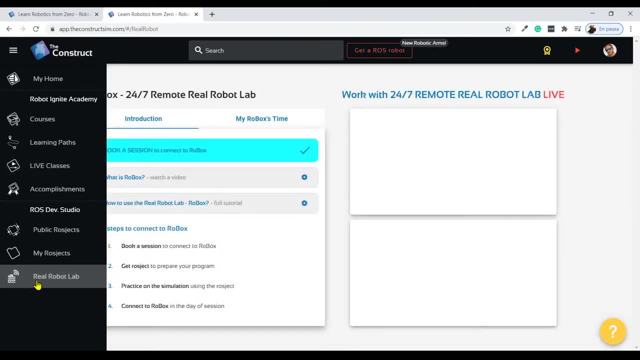 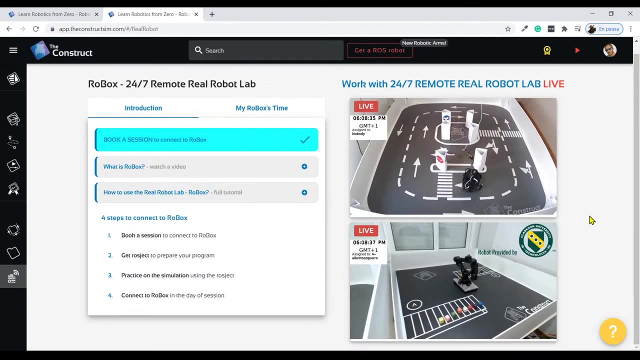 been working with the real robot lab. you can find this tool also here in the left menu, here the bottom one which says real robot lab. so here is where you can book sessions. in other tools work with real robots. Up here we can see the Tartalbot 3 robot which we have been working with. 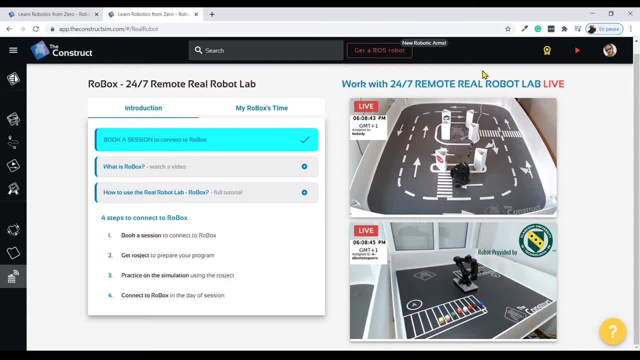 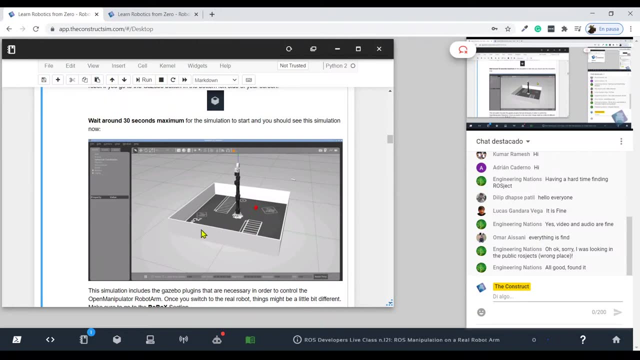 this robot in previous live classes already and you can see now here that we have a second robot, which is this one. This is the manipulator robot that we are going to be using today, that we are going to connect to today. As you can see, it's the same robot as the one we have in the simulation. 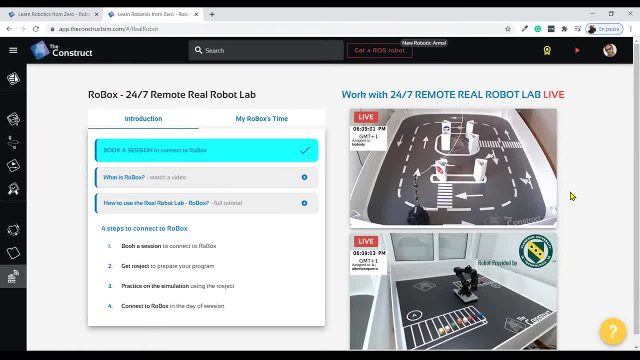 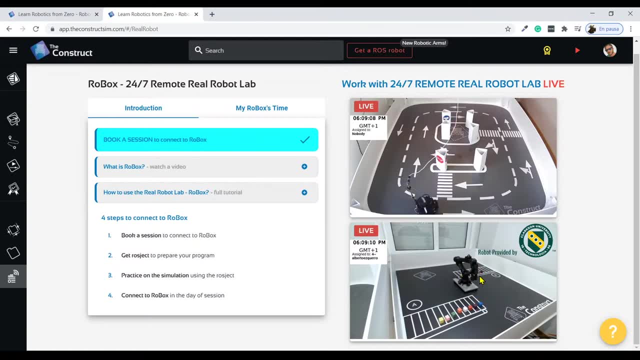 you will see it, and we are going to use the real robot lab tool in order to connect to this manipulator robot. I will show you later a little bit more, but basically here you can book sessions in order to connect to real robots. In this case we have the Tartalbot 3 robot in case. 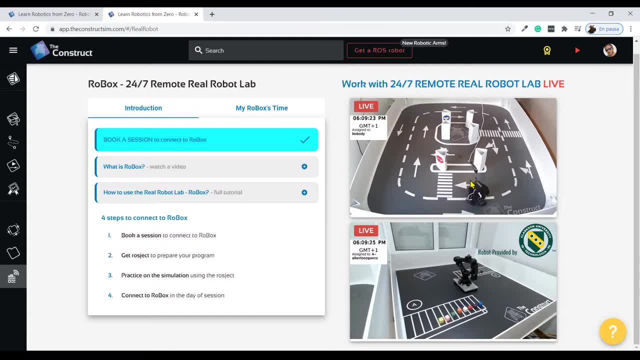 you want to test a mobile robot, for instance for- I don't know- for navigation, for testing navigation programs, etc. You can use the Tartalbot 3 robot, also many other things, and you have the option now to book a session in order to connect to the manipulator, in order to test, let's say, motion. 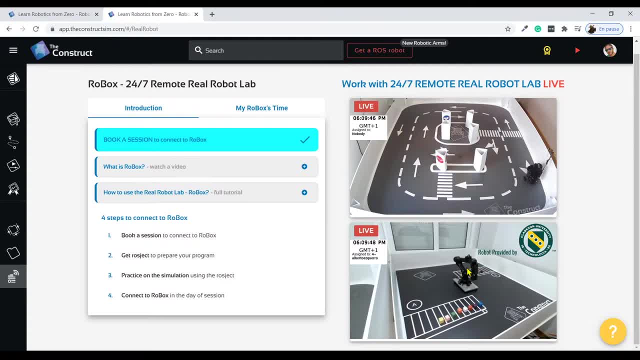 planning, you can use move it, etc. etc. All right then. not today, but starting from tomorrow, you are going to have the option to book one session for each one. Well, you are going to be able to book two sessions in total totally for free, All right, so normally, 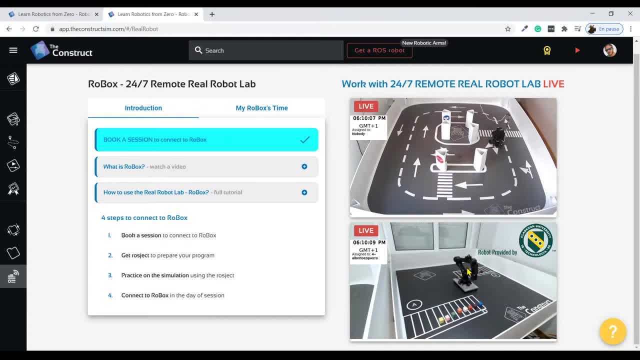 this option is only for subscribers or our clients, but starting from tomorrow and until the end of this week, you are going to have the option to book two sessions completely for free. You can choose to book two sessions for the Tartalbot 3 robot or two sessions for the manipulator or. 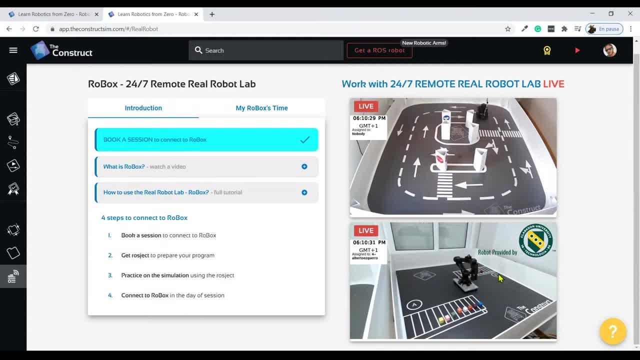 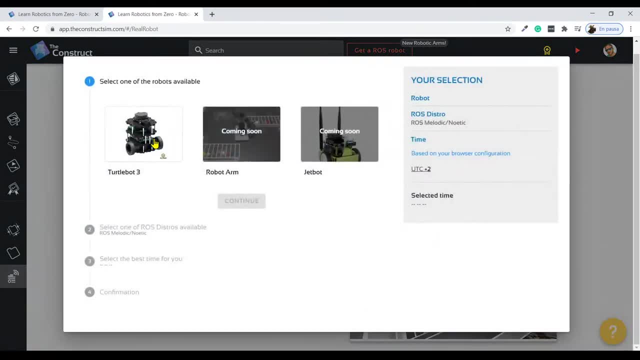 one for the Tartalbot And another one for the manipulator. All right, and it's as easy as following the instructions here selecting the robot. as you can see, right now we only have the Tartalbot 3 available, but, as I have just said, tomorrow we are going to activate the option in order to also be able to book a session. 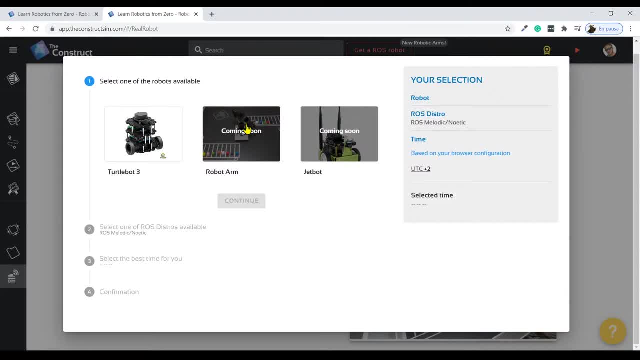 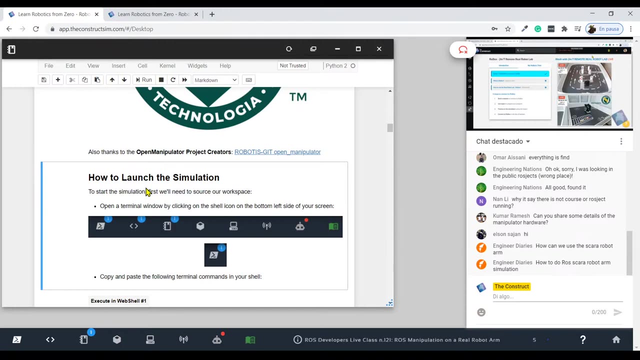 with the manipulator robot. All right, Okay, then, having explained all these and the plan for today, Today's life class, Let's go for it. So let me come back to my Russian. Let me ask you, all of you guys: have you already opened the project? Do you have it open it? 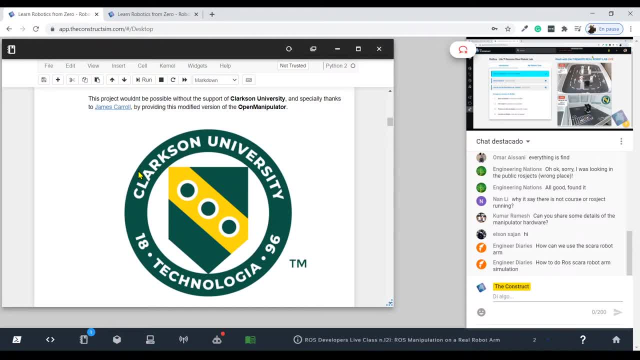 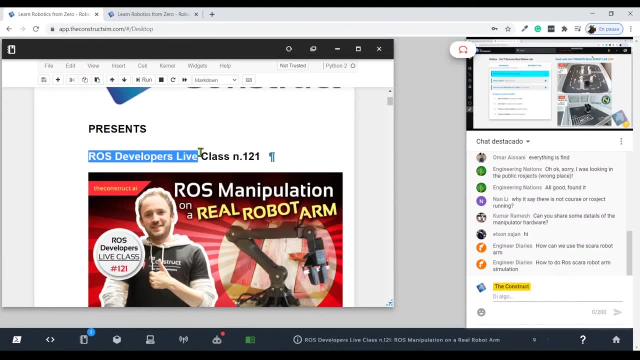 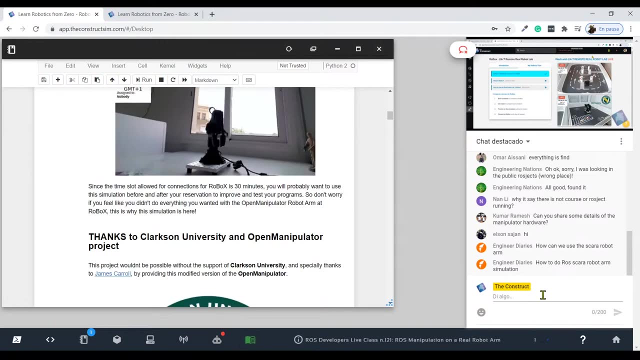 Like I have it Here. Yes, It has loaded properly. You have here the proper notebook. Notebook has to say: Mount developer's life, class One hundred and twenty one. Everything is fine with rosette, So Can we start working? I would like to wait for everybody, or almost everybody, to be here at the same point as I am. 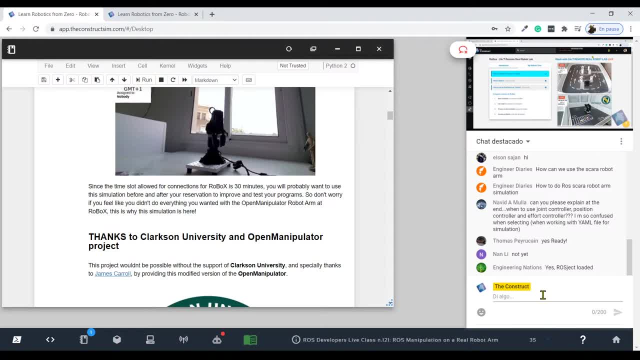 Okay, yes, ready, Not yet. Yes, project loaded. Benjamin Barnes: yes, Okay, great. So I can see that almost everybody has his project loaded. Let me see here I can see some questions. Navid, can you please explain at the end when to use joint controller, position controller and everything? 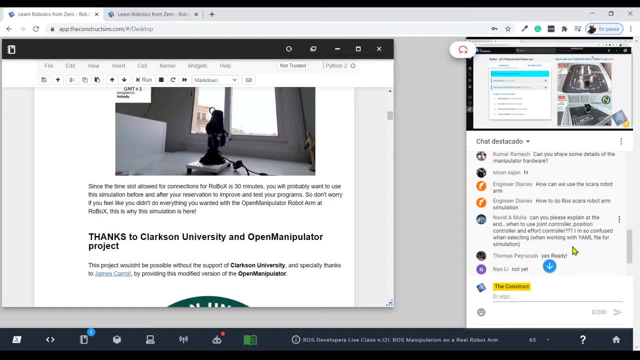 F4 controller. I'm so confused when selecting. We're working with YAML file for simulation. Well, it depends. It depends on the hardware you are using. It depends on many things. I can't really give you a proper answer. Usually, in manipulators, F4 controllers are used. However, you have to know that there are two controllers. 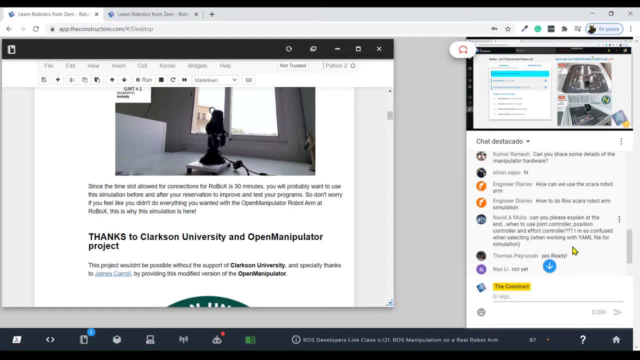 I mean from one end, which is the hardware end. let's say they are going to be, You are going to, You are going to be using an F4 controller, so the hardware is going to receive F4 commands. yeah, 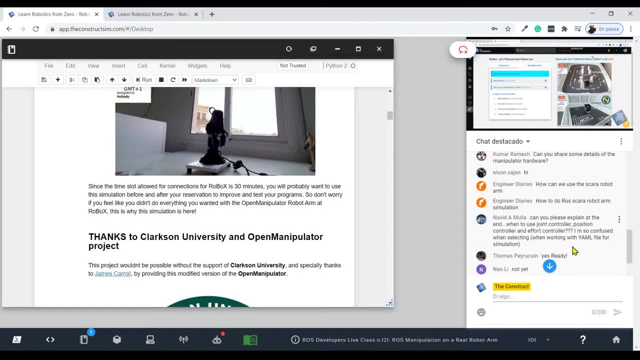 But in the ROS side, probably, you are going to use position controllers, So you are going to send positions to the controller and then the controller is going to convert it into F4, which is going to be sent to the manipulator hardware. I would say that this is the most common configuration. 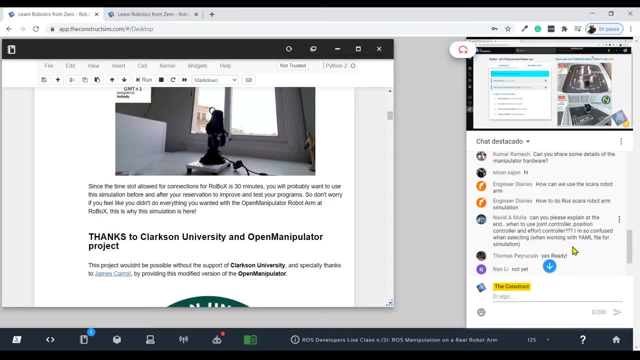 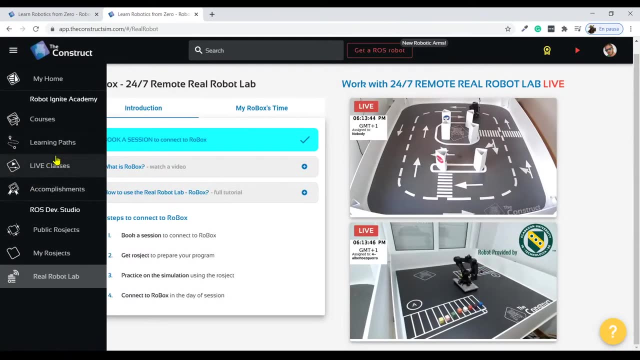 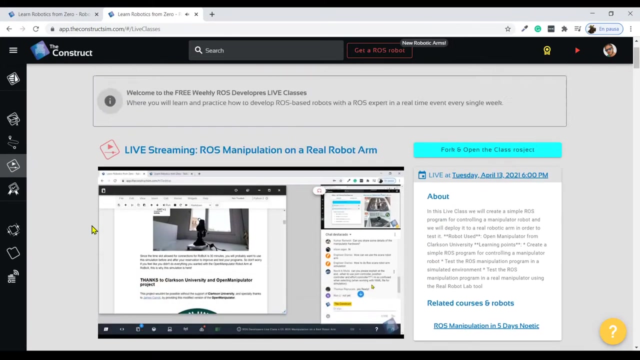 But it depends in many, many things. Rosette link. There is no Rosette link. Okay, Remember, you have to come here in the construct, to the live classes section, Live classes section, And then you click on the button here which is highlighted in light blue, which says fork. 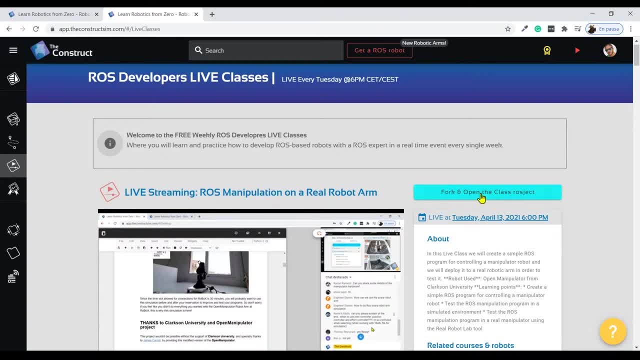 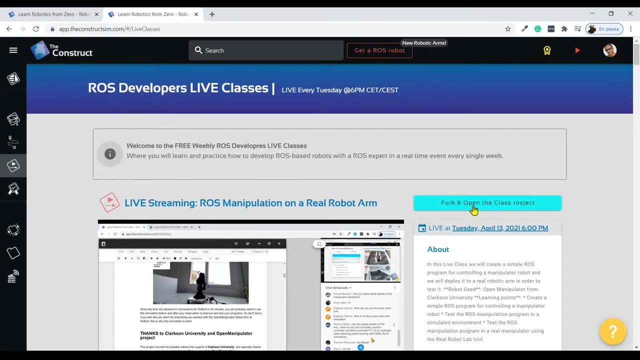 And And Open the class Rosette. You click on this button and you are going to automatically get the Rosette into your workspace And it's actually going to automatically open also. So left menu, live classes and fork and open the class Rosette. 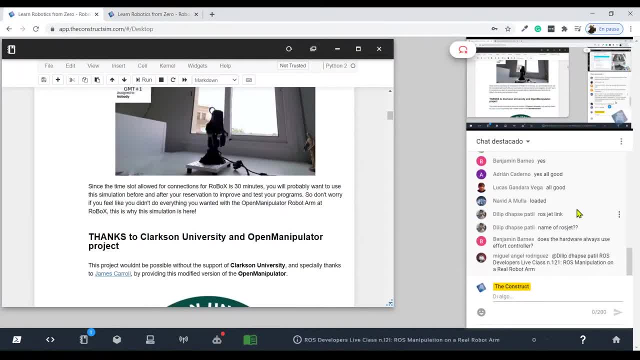 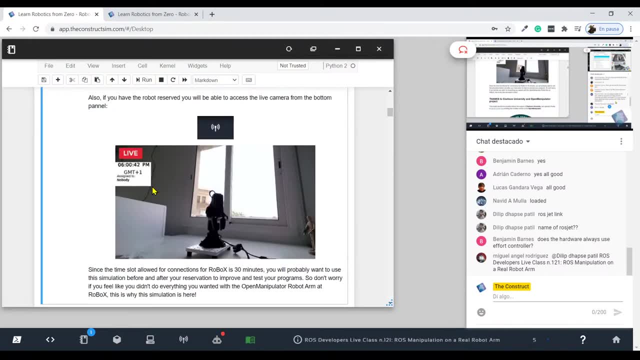 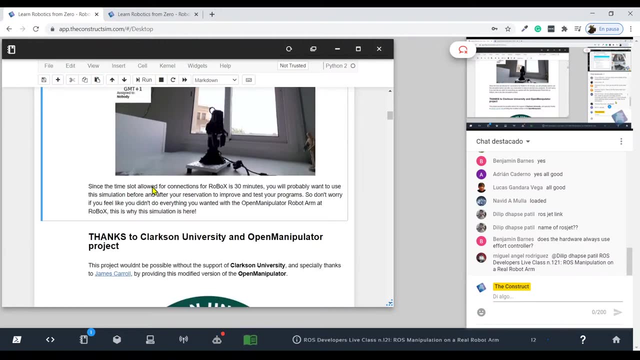 Okay, No Rosette link shared anymore. All right, All right, Let's start. So today we are going to be working with A version, a custom version, let's say, of the OpenManipulator robot, And it has been done, this custom version, by the guys of the Clarkson University. 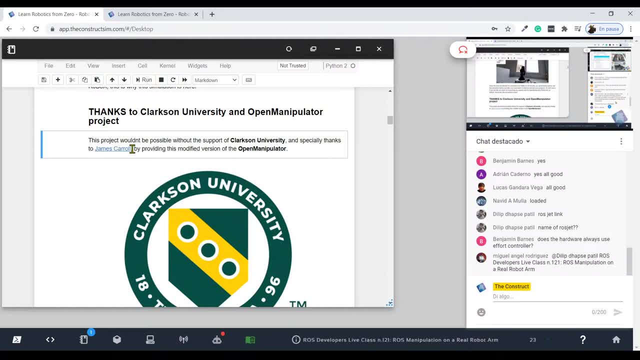 All right, Which are led by James Carroll. They have created this custom version of the OpenManipulator robot And indeed they have sent one of these robots to us. They are based in USA And they have. They have sent us this robot from USA here to Spain, to Barcelona. 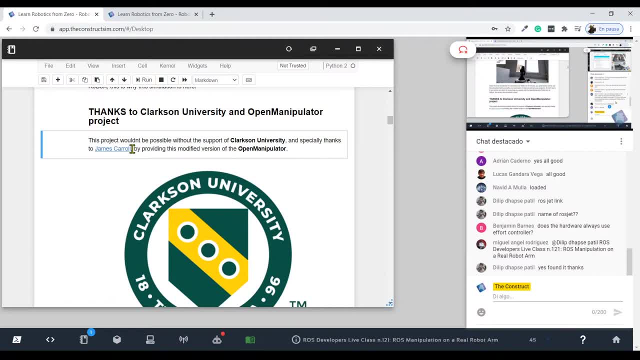 And actually, this is the robot, the one that they sent to us. This is the robot that we are going to be using today in the real robot lab, So it's the real robot that we are going to be connecting to. 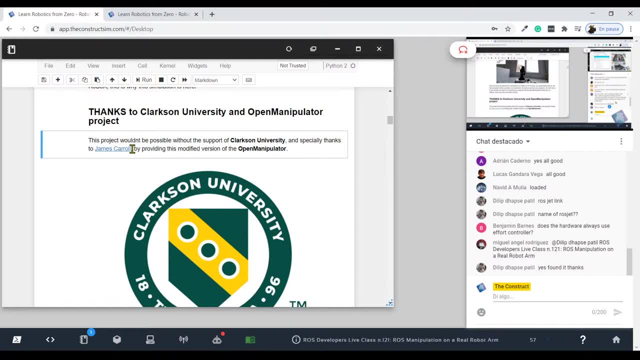 So a big thanks to the Clarkson University and James Carroll, And also, of course, to the OpenManipulator project, which is, let's say, the base of this manipulator robot that we are going to be using today. All right, 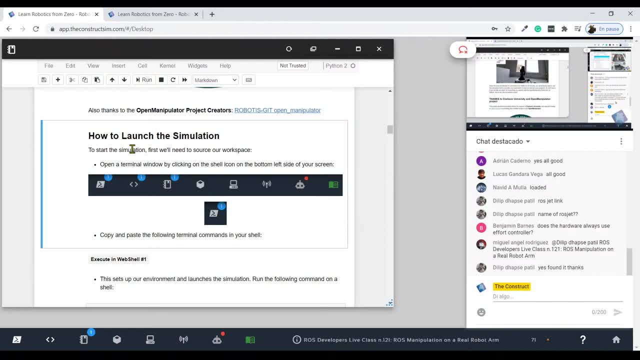 Then let's start by the beginning And, as I have said before, we are going to start by launching the simulation. So we are going to start by using a simulated version of this manipulator. So, in order to launch our simulation, we are going to first of all need to open a new web shell. 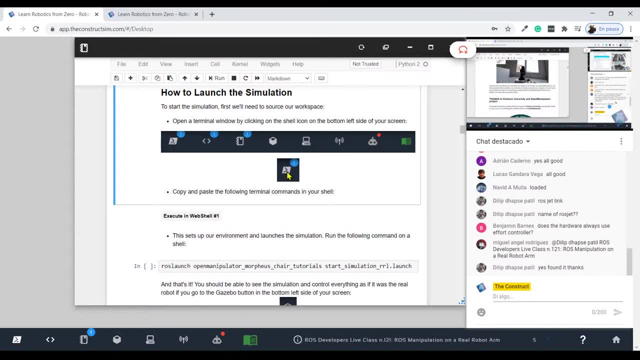 And we can open a new web shell by clicking on this icon that you can see here, Highlighted in the notebook, which is this one, the first one starting from the left. So by clicking in this button, we are going to open a new web shell. 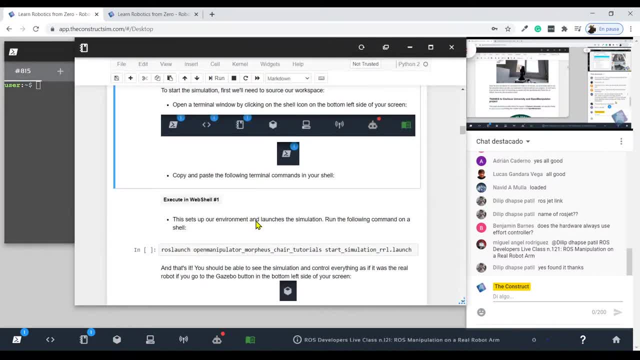 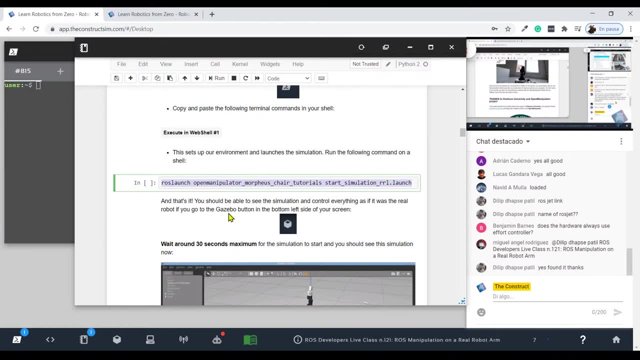 All right, Then, inside this web shell, we are going to run the command that we have here also in the notebook. I'm going to copy it here with Control-C, directly from the notebook And I'm going to paste it here into my web shell. 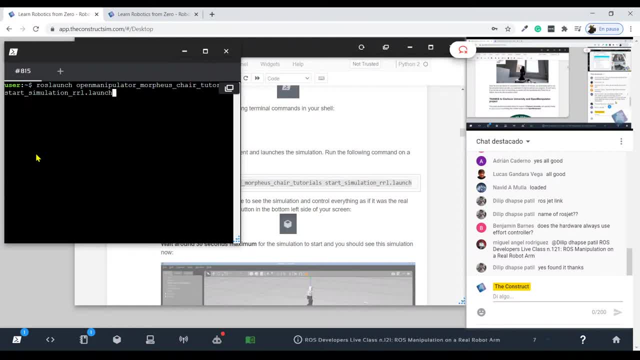 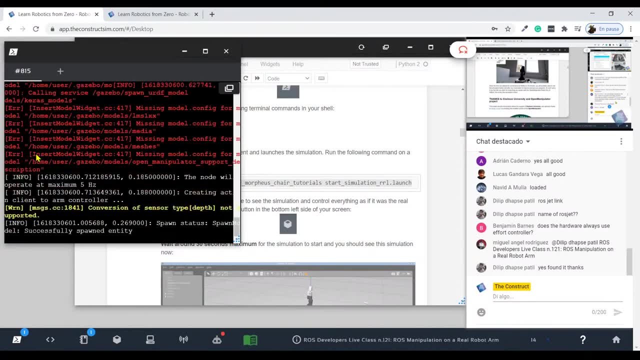 Yes, just copy and paste in order to save time, And then I'm going to run this command. So this is going to start launching Gazebo and loading the URDF and everything in order to have the simulation of this robot. 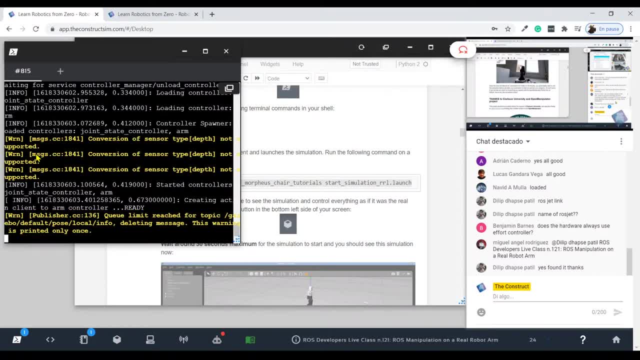 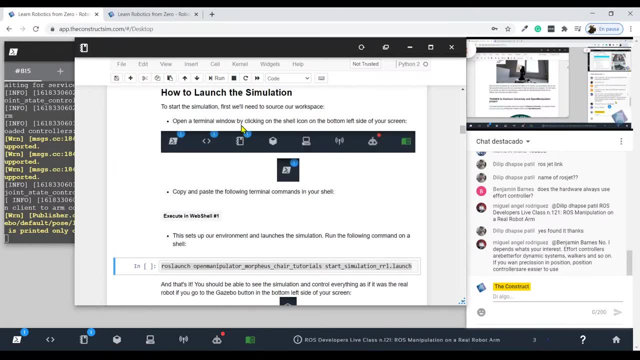 So now I have launched the simulation, but in order to visualize it, I'm going to have to click on this cube icon, As you can see all the instructions of everything that I am doing and everything that I will be doing during this live class. 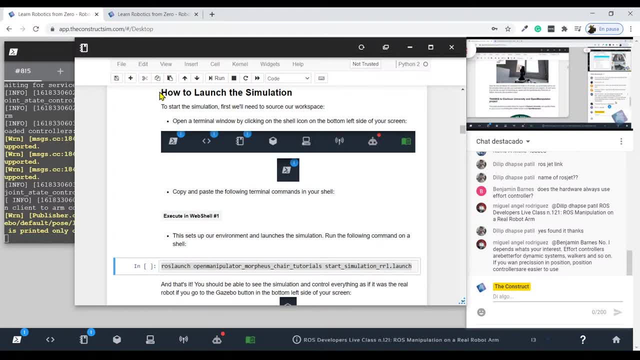 you can find it in the description. You can find all these instructions here in the notebook, All right. So in case you miss something that I am saying, in case you need to go to the bathroom in a rush and you miss a couple of minutes of the live class, 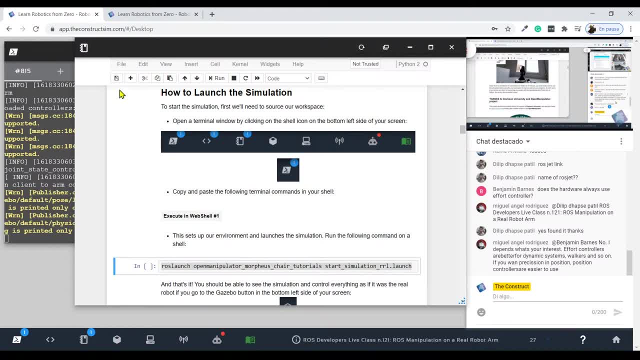 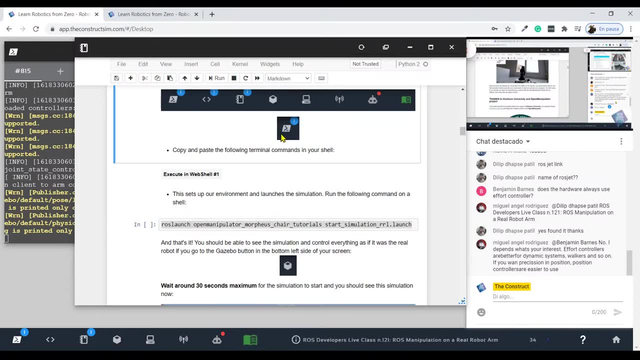 don't worry, don't panic, because you have all the instructions here in the notebook So you can follow them at your own pace. All right, Then we open a web shell So we launch the command here that we have in the notebook. 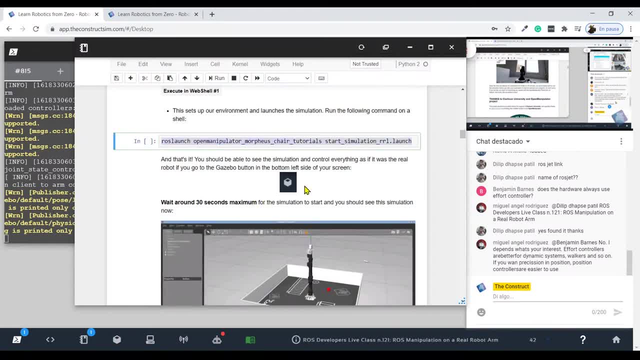 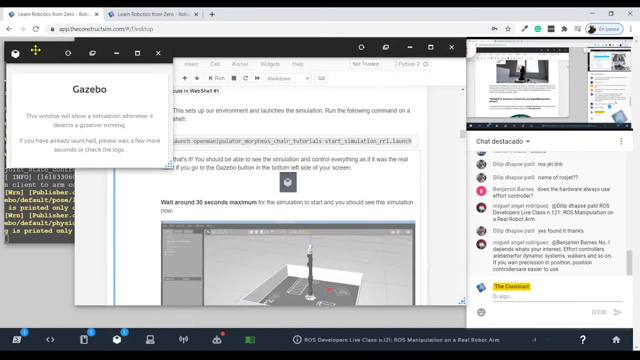 in order to Start the Gazebo simulation, And then, finally, we are going to click on this cube icon that you can see here, which is going to open the Gazebo display. let's say, Actually, it's a GC client. 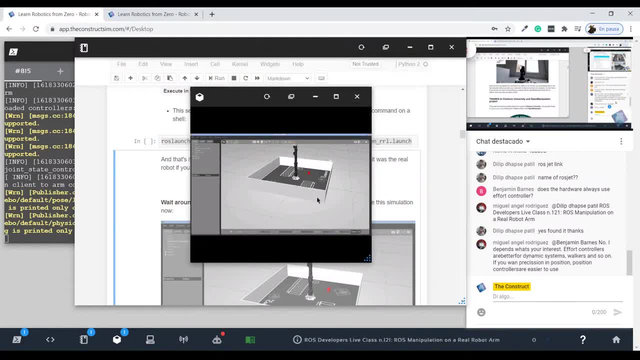 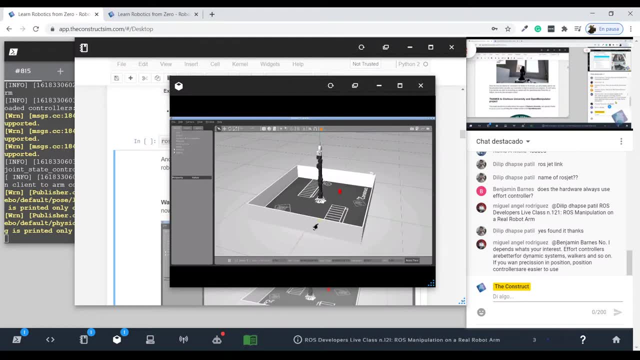 All right, It's going to open GC client And here, as you can see, we are now able to see the Gazebo simulation. Let me put it here a little bit more in the center. So here we have our manipulator robot. 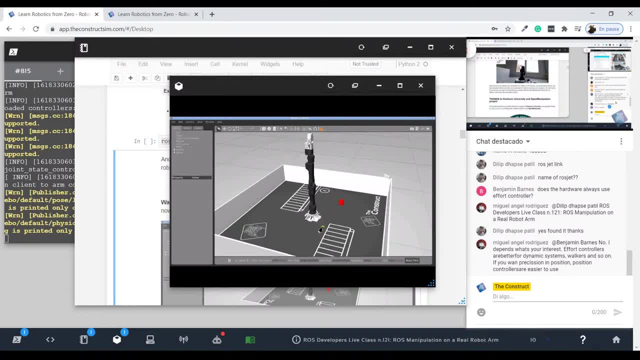 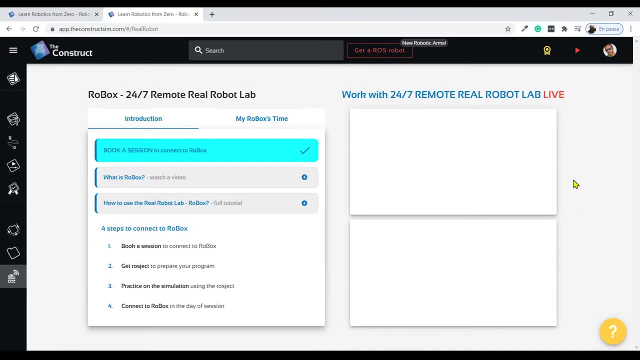 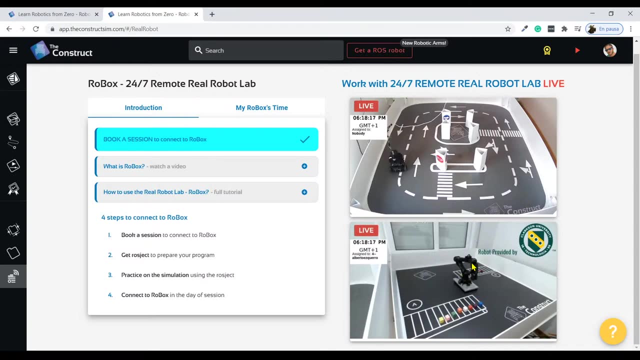 In Gazebo. this is actually a copy, a representation of the real one. So, as you can see, if you come here to a real robot lab, it's the same environment. So, basically, it's a copy of the real environment. 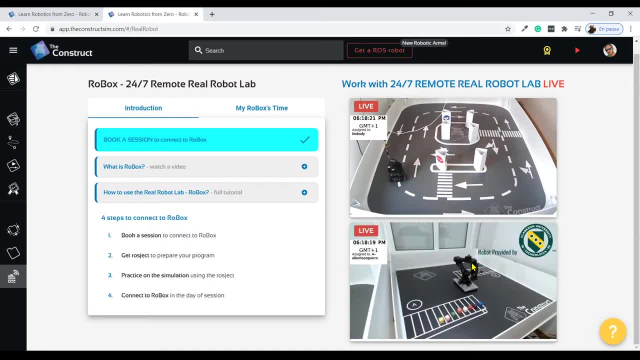 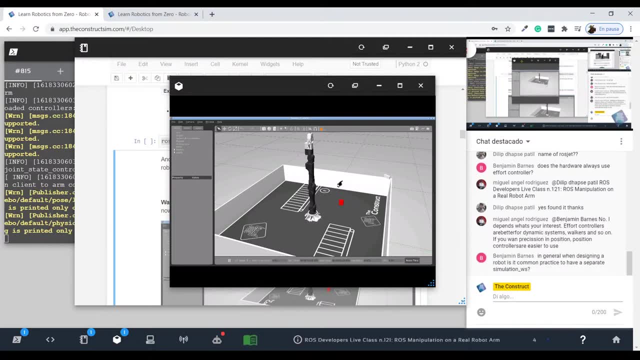 but in this case in a Gazebo simulation. This is convenient because, since we are going to be creating programs and testing them in the simulated version, what we want is that the simulated environment is as close as the real environment as possible. 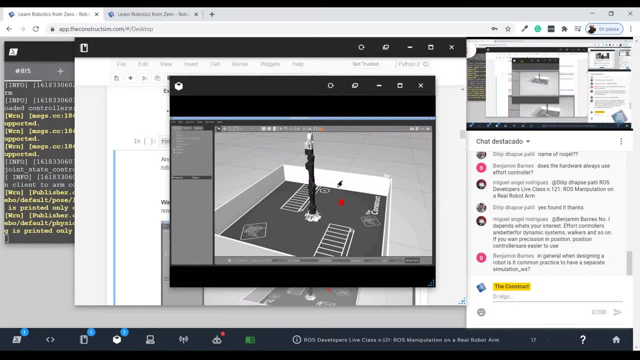 All right, Because basically this is going to mean that if something works in the simulation, it should work also in the real environment. All right, Of course, this is not always like this, but in general you have to try to make your simulated environment and robot. 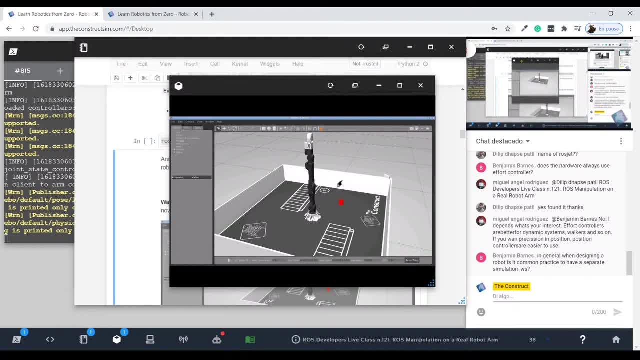 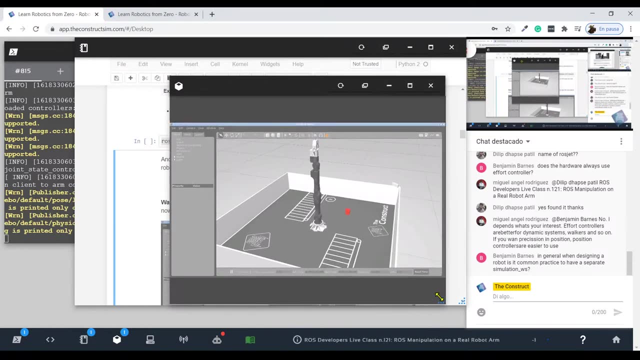 as similar as possible to the real one. All right, This is going to allow you to be able to replicate everything that you do and test in the simulated version into the real robot. All right, So we have started here, our Gazebo simulation of the manipulator. 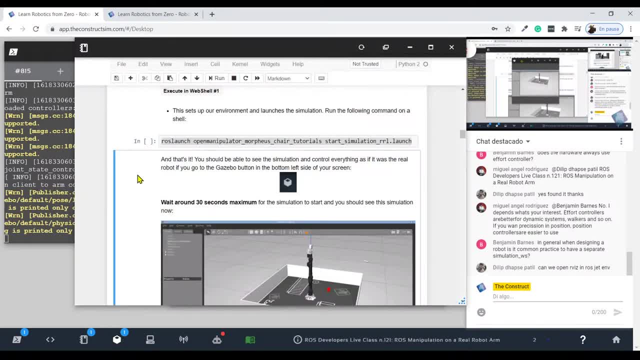 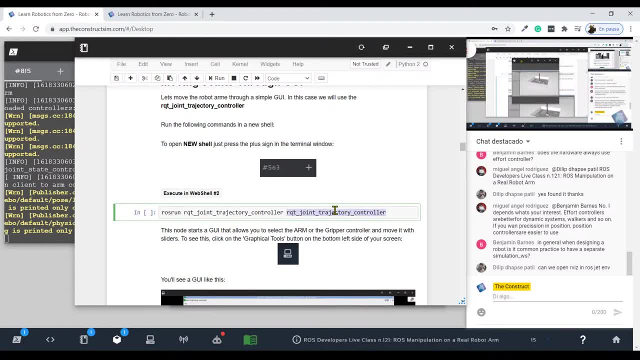 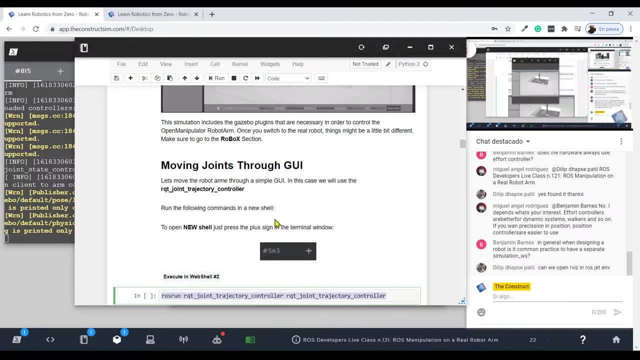 All right, Then in order to start this RQT GUI, we are going to have to execute this command here. So if you keep going down in the notebook, you are going to find the next section, which is moving joints through GUI. 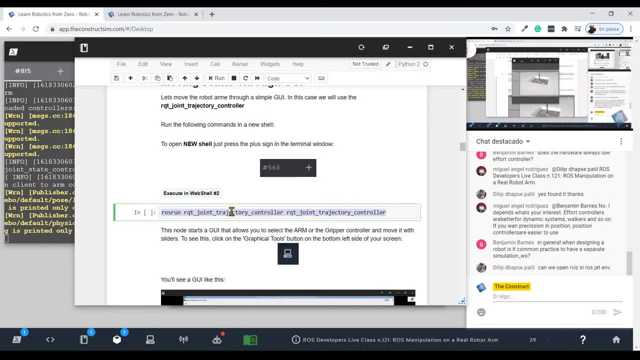 And here you are going to find another command, So we are going to have to launch also this command. Then I'm going to copy it here from the command from the notebook. Sorry, I'm going to copy it with CTRL-C. 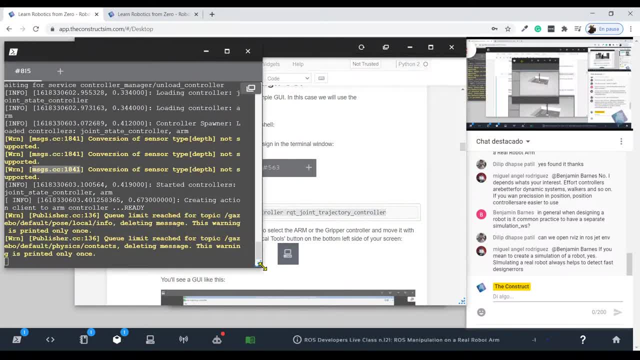 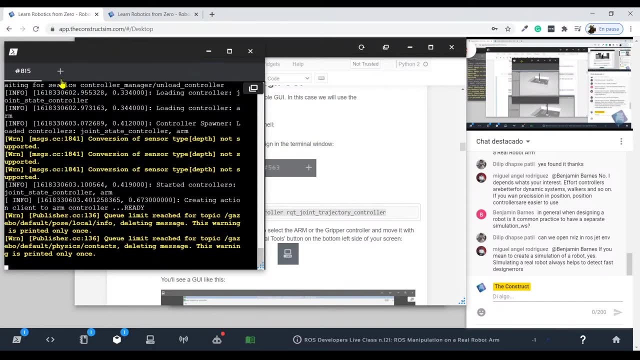 And I'm going to come back here to my web shells, And I already have this web shell occupied, right, I already have it occupied because I have here my simulation running, So I'm going to click here in the plus icon I have here in the top in order to open a new shell. 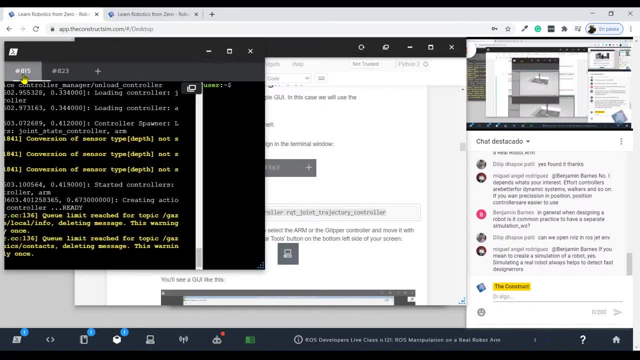 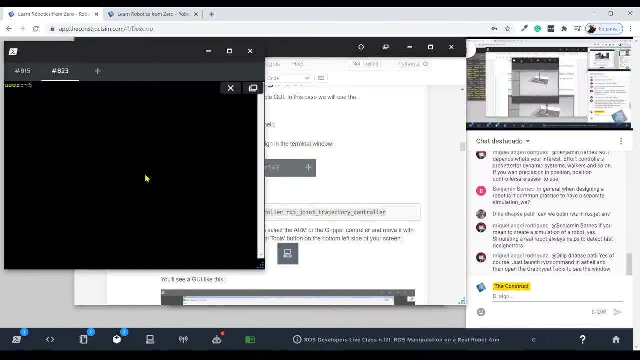 There we go. So now I have here my first shell And I can switch to the new shell And I can switch between them. So in this new shell I'm going to paste the command Which is going to launch Ercutty. 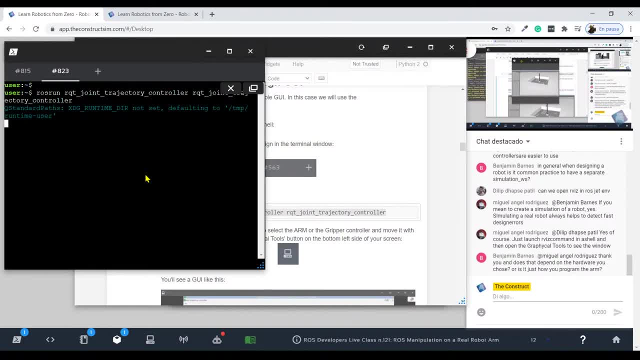 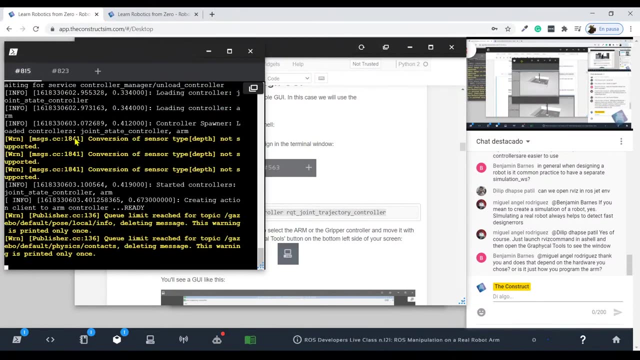 And this is going to allow me to control, using a GUI, in a visual way, the joints of my robot. So, again again, here in the web shell, what I have done right now is to just execute the command right. So here I have executed the simulation. 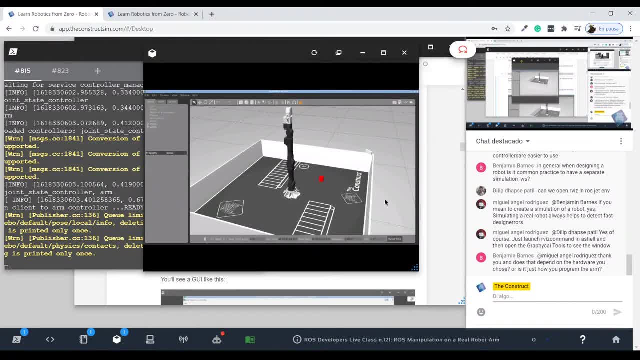 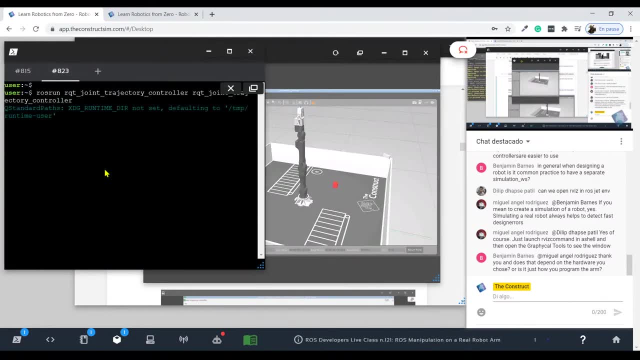 But I needed to start the client in order to be able to visualize The Gazebo simulation, right? So it's very similar here. Now I have started this Ercutty GUI, But in order to visualize it, in order to see it, to actually see it, I have to open the graphical tools. 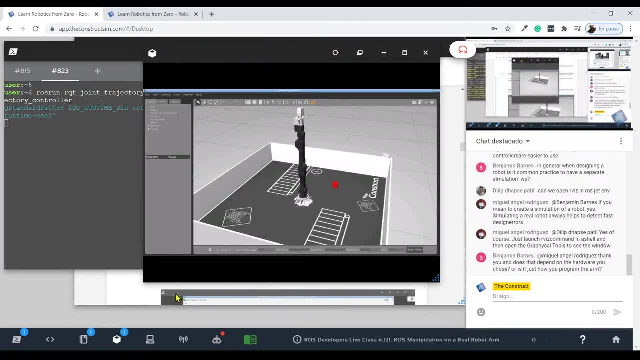 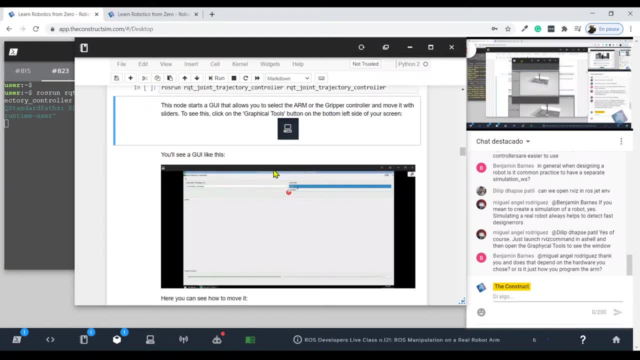 And how do I do so? Very easy, So I can open the graphical tools. Let me go back to the notebook By clicking on this computer icon, Which you can see. it's here, right next to the Gazebo icon, We have this computer-like icon. 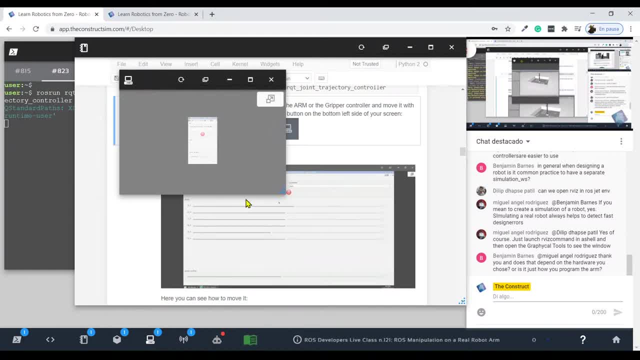 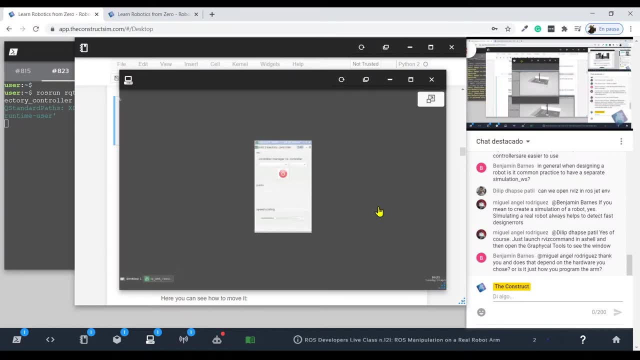 And if I click it, this is going to open a new window which contains the graphical tools. Here I have it. Here I have them, Alright, Alright. So now what I want to do is to maximize this window, Because right now it's very small. 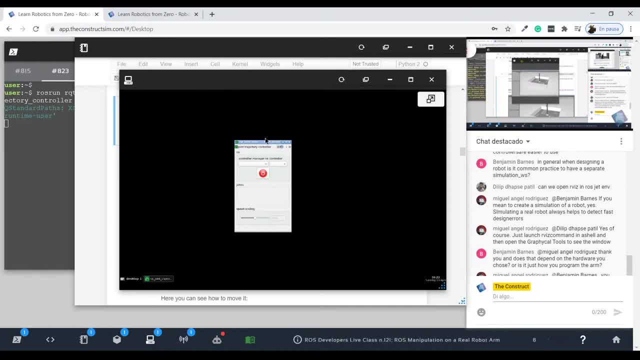 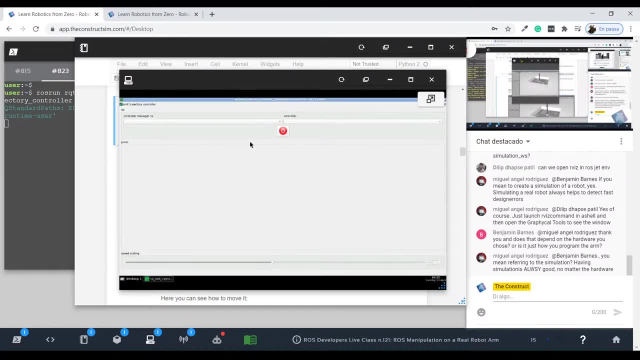 So if I double click here with my mouse, If I double click here in the top bar of the window, Let me do it Double click. This is going to maximize it, Okay. So this way I'm going to be able to visualize it. 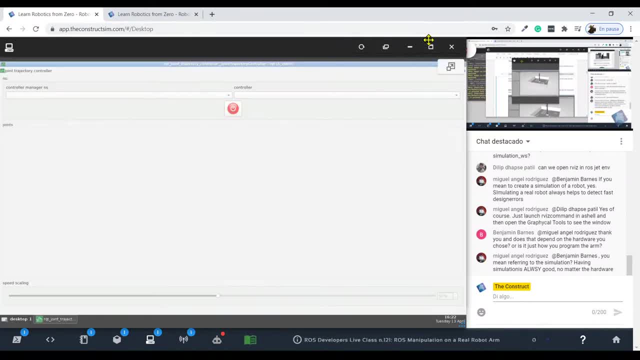 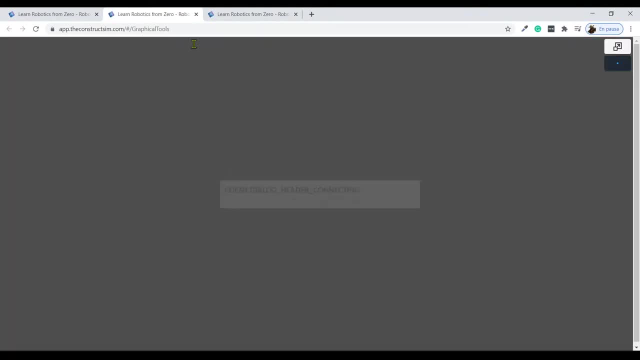 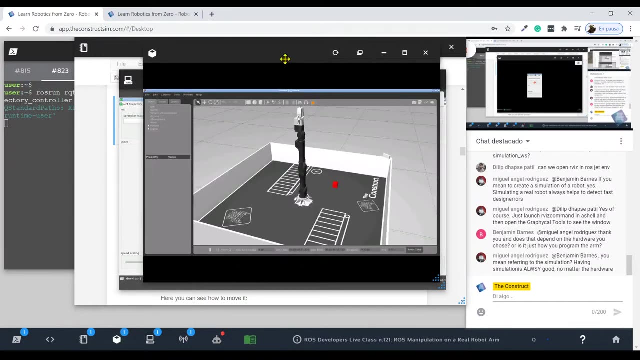 Visualize everything better. Of course, you can also maximize this, Minimize it. You can move it to a different tab if you prefer to work like this. Whatever configuration you prefer, Okay, I'm going to keep it all here. Let me, by the way, also put the simulation here. 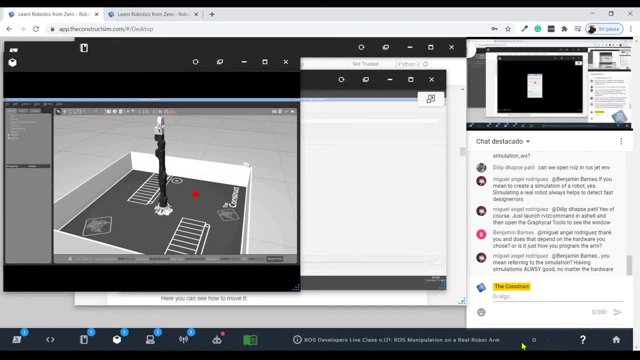 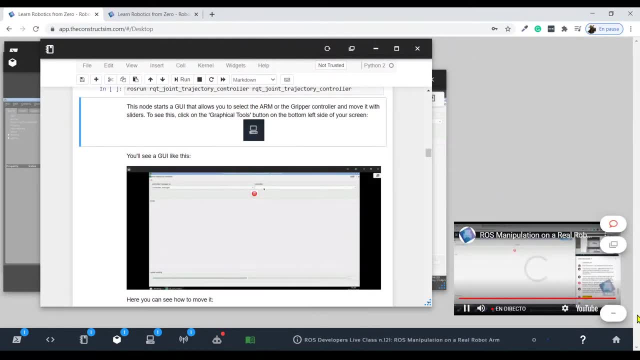 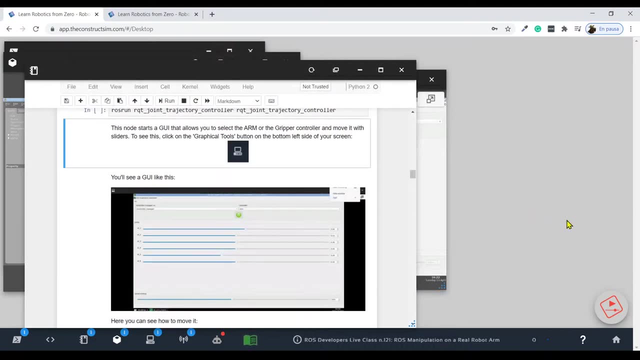 Okay, Okay, And I'm going to actually minimize, for now, this. Let me minimize this for a moment so that I have a bit more of a space. Let me put it: Okay, Action, Move it here. Okay, No problem. 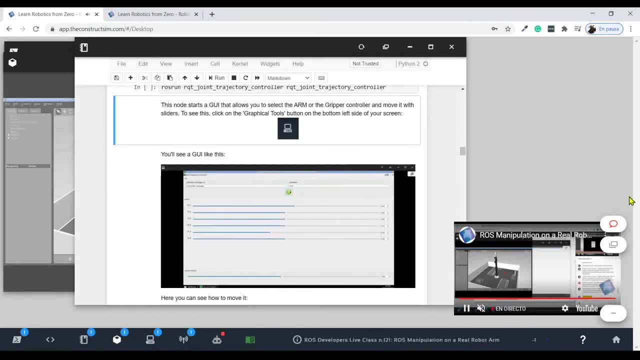 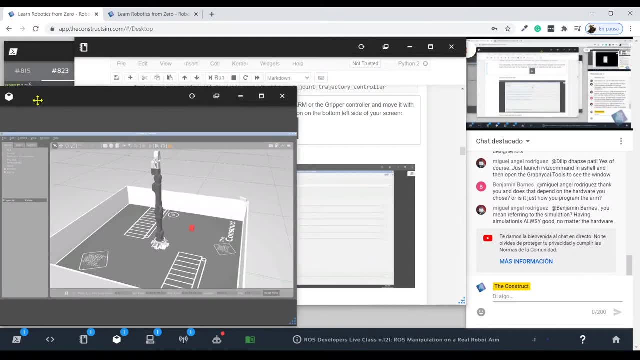 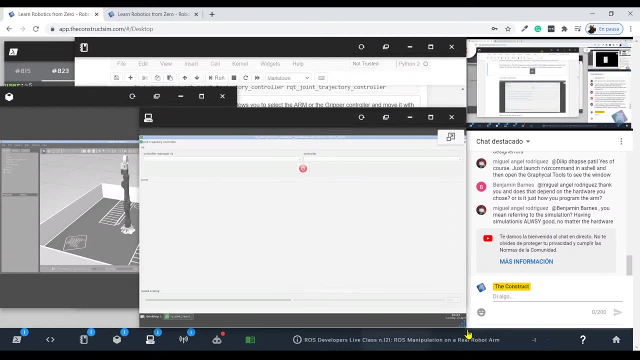 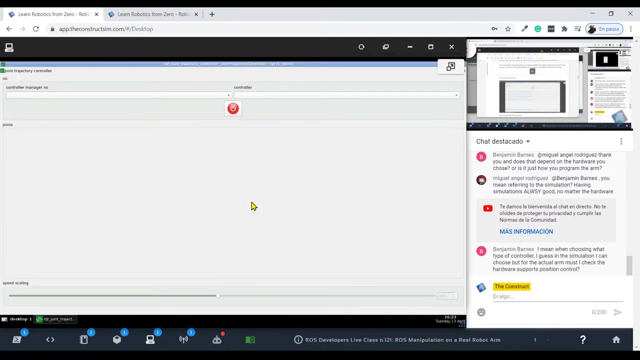 No problem, Here back again. Okay. So let me put the simulation here at one side and the graphical tools window here at the other side. Let me configure it a little bit like this. All right, Then let me maximize this for a moment so that you can see it better. 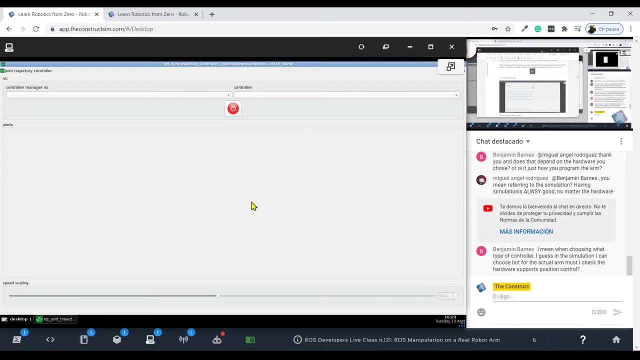 So now, here in this Ercucci GUI which I have launched, which contains the joint trajectory controller, what I'm going to do is to: first of all, I'm going to sell it here in the controller. So I'm going to sell it here in the controller manager namespace. 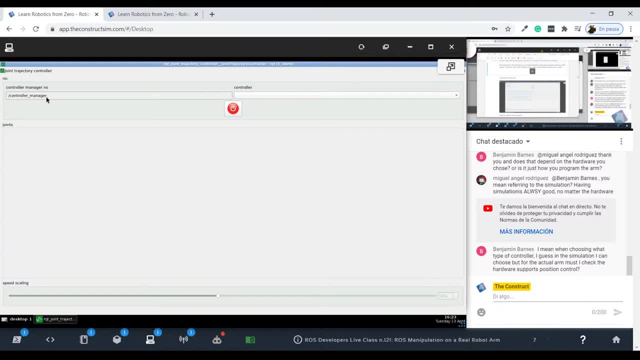 I'm going to select the only option that you have, which is controller manager. So we are going to select the namespace here, which is controller manager, And here, in the other menu, which says controller, we are going to select also the only option that you have. 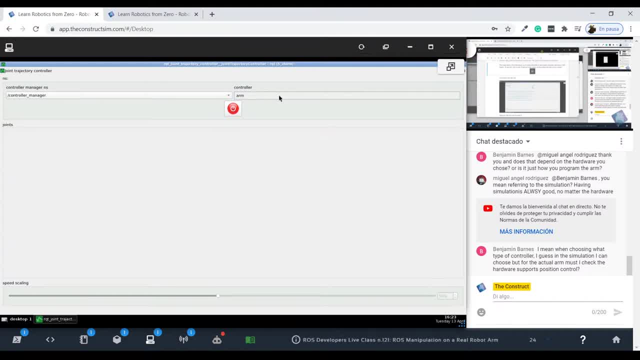 So no chance to fail here. Okay, You only have one option. So controller manager And here arm. Okay, There we go. Let me select it. There we go. Okay, Now I have selected it. So once you have the configuration here selected and set up, you're going to see that these sliders appear. 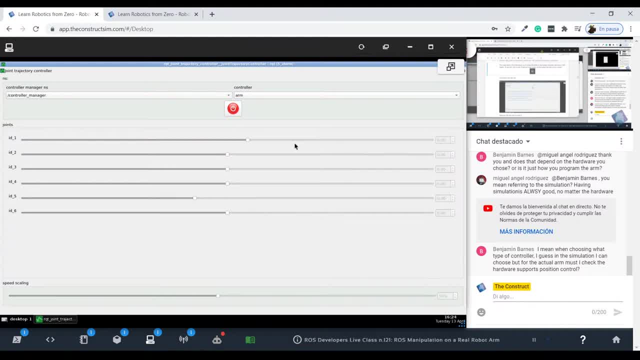 So, as you can see, you have one slider for each of the joints of the robot. Okay, So right now, as you can see, I have one slider for each of the joints of the robot And you can see this is in a faded gray color because we are not yet connected to the trajectory controller. 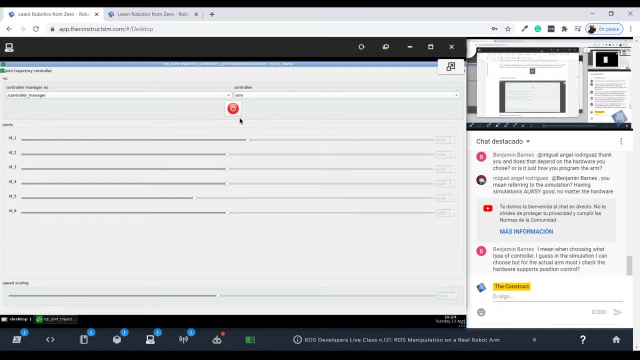 So, in order to connect to this trajectory controller, we need to click here in the on-off button. You need to click here and you are going to see that this red color is going to turn to green. So now we are connected with the joint trajectory controller to the robot arm. 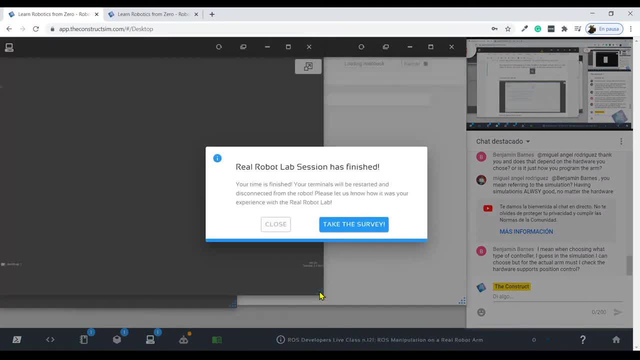 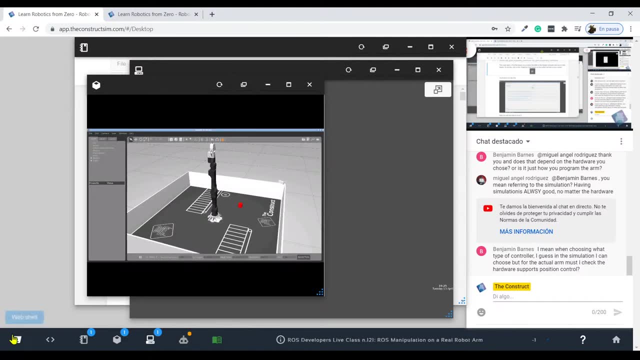 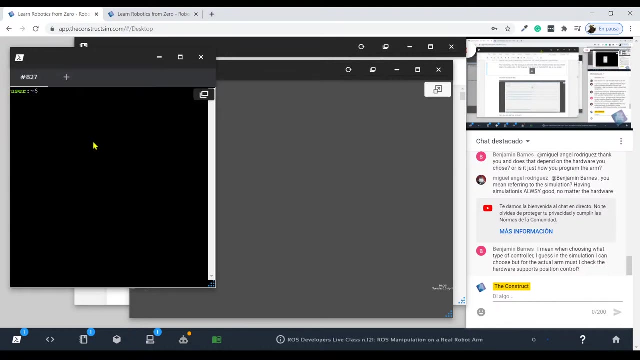 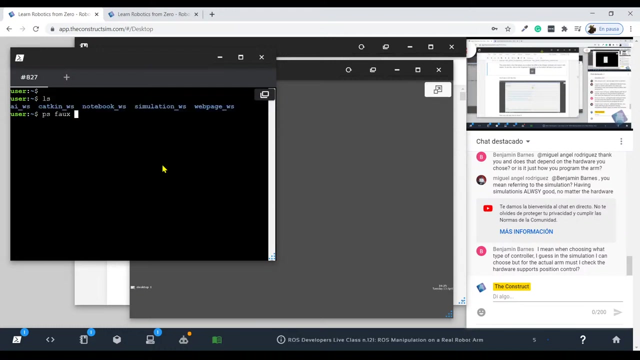 Then now let me- Oops, One session has finished of the robot lab. Okay, No worries, No worries, Let me just relaunch it again One second. Yes, Yes, Just one of the sessions that I have with the real robot. 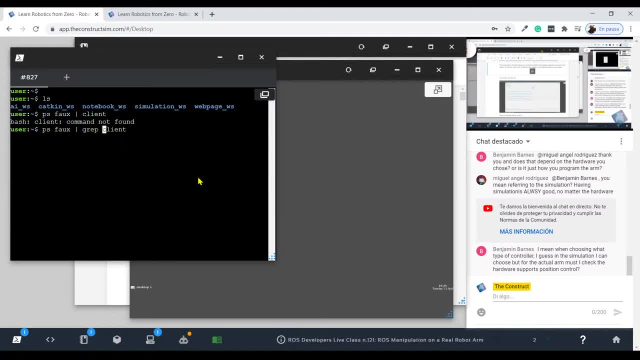 The real robot lab has finished it, So it has closed my shells. Okay, Then let me Very quickly. you don't need to do this because you are not connected right now to the real robot lab, So don't worry. 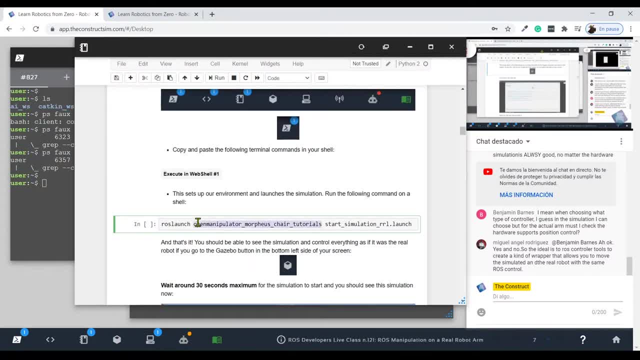 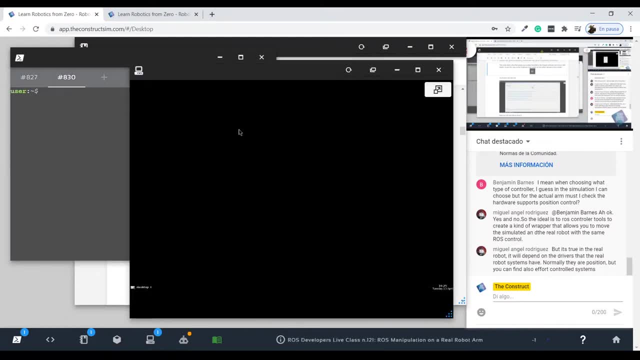 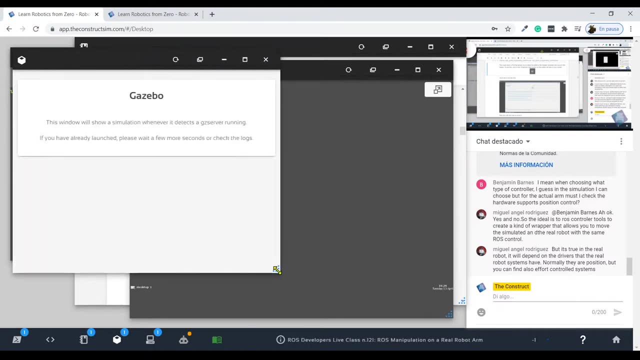 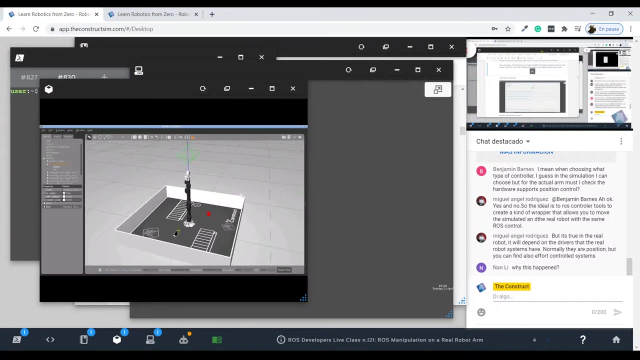 This is just only going to happen to me, So don't worry about it. I'm just going to relaunch everything very quickly. The simulation first, Which should, Which should, appear here. Here we have it, Great. And I'm going to launch again the RQT trajectory controller very quickly here. 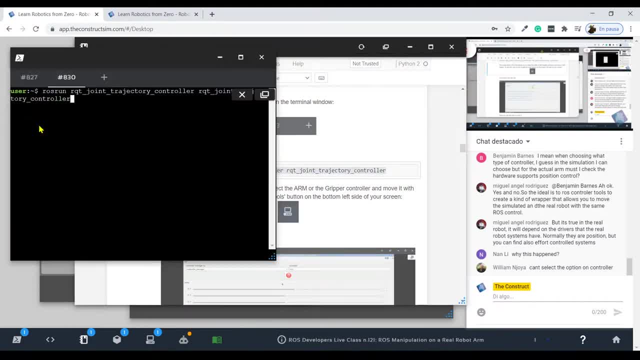 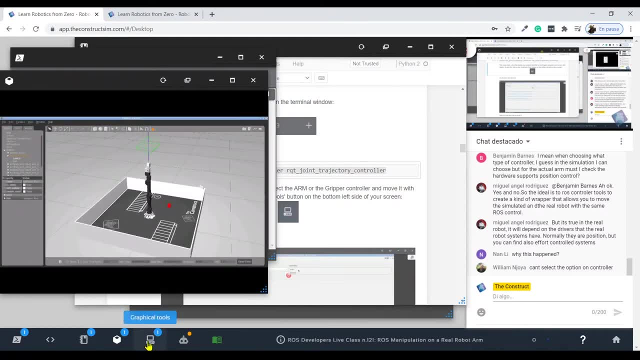 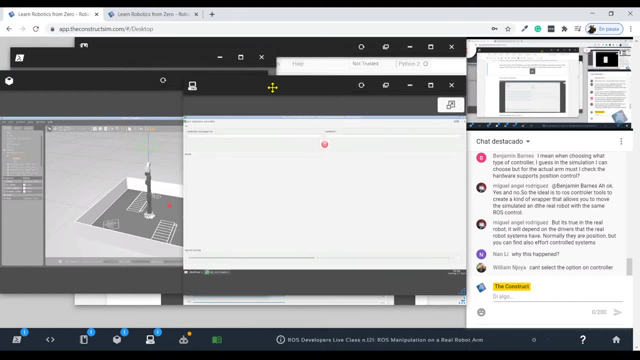 Copy and paste. There we go. Okay, So let me put again my setup: here At the left side the simulation At, here at the right side the trajectory controller. So let me make it a bit smaller here. 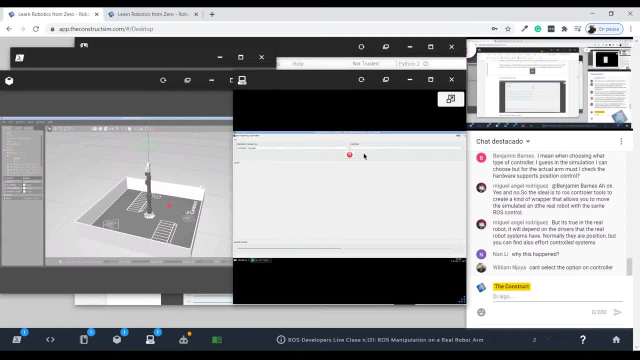 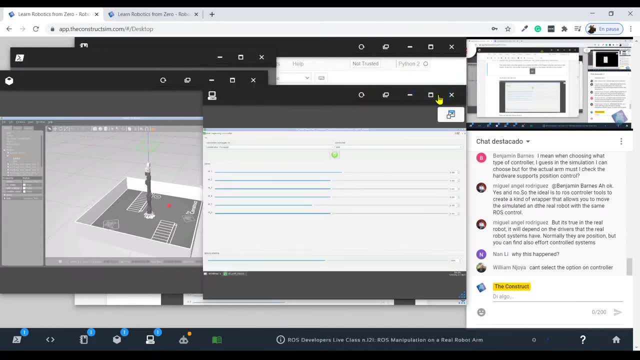 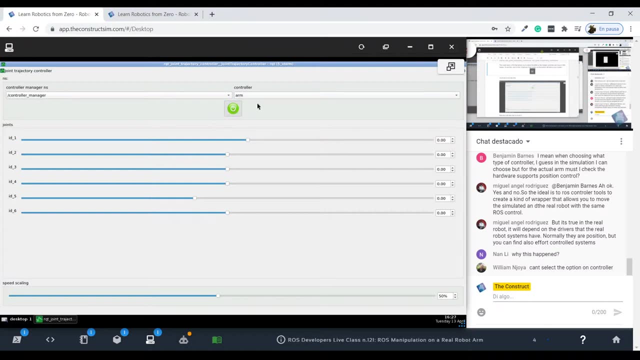 There we go. Okay, So I'm going to select one more time controller manager Arm. Connect to it. Make sure, Make sure that the button is in green so that you are going to be connected. If this button is in red, this means that it's not connected. 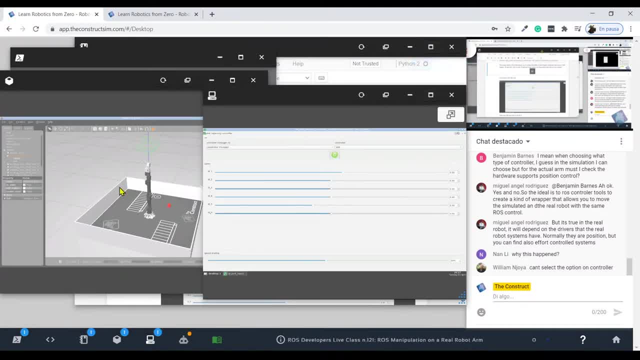 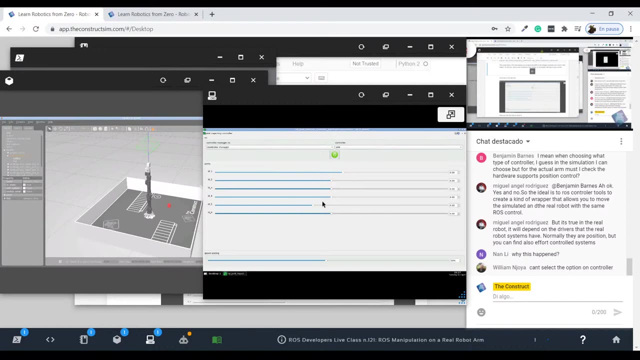 All right, Then let me. So, now that we are connected, we can move these slides in order to control the different joints of our robot. All right, So let me do it right now. So, for instance, let me move this ID 5.. 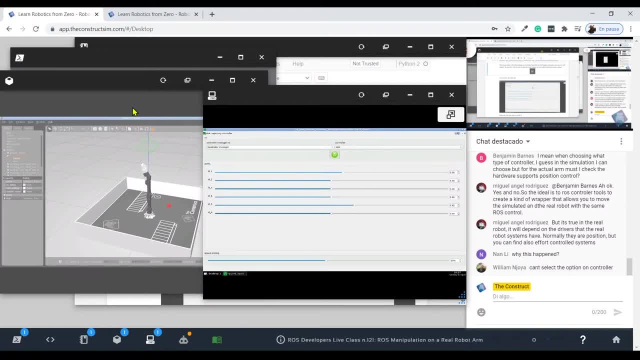 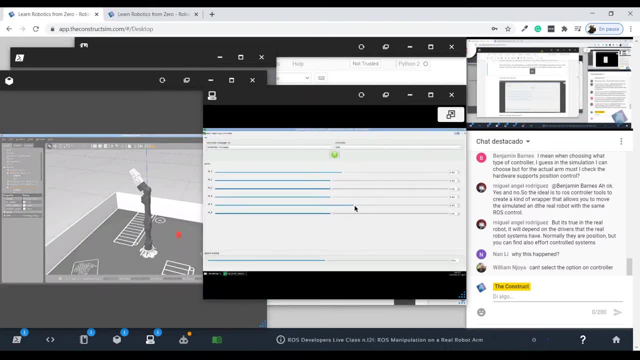 Let me move the slider And, as you can see here in the simulation, this: Let me get a bit. Let me get a bit closer so that you can see it better. There we go. So if you move the slider, you're going to see that the joint 5, in this case the joint 5, is going to move. 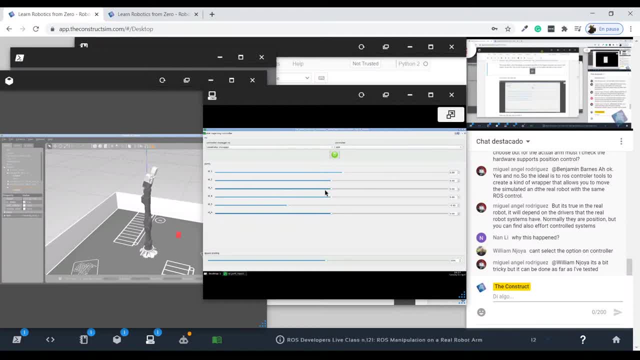 All right, Let me move now. for instance, let's try joint 3, which is this one- And I can control it here in a graphical and very easy way- all the joints of my robot. So, as you can see, in this case our robot has six different joints. 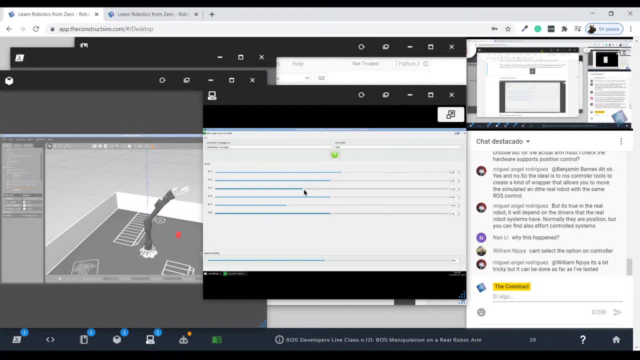 All right? Okay, then let's keep going. So once that we have introduced a little bit our manipulator robot, we have seen how to control the different joints and that everything is working in the simulation, I'm going to close this GUI. 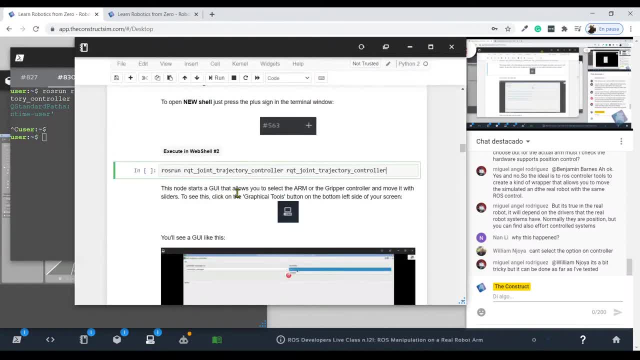 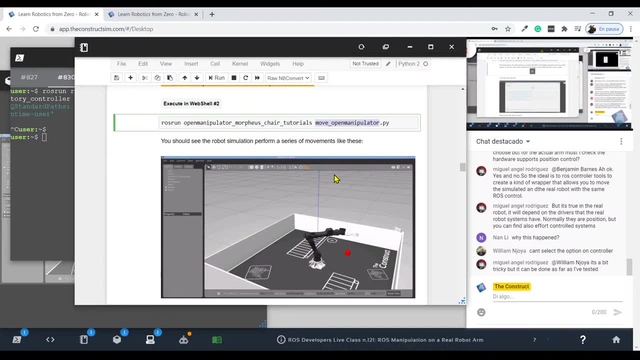 And what I'm going to do next- Let me come back here to the notebook- is to actually I'm going to execute a script, as you can see here, this moveOpenManipulatorpy script. So I'm going to execute a Python script that, basically, is going to start moving all the joints of the robot to random positions. 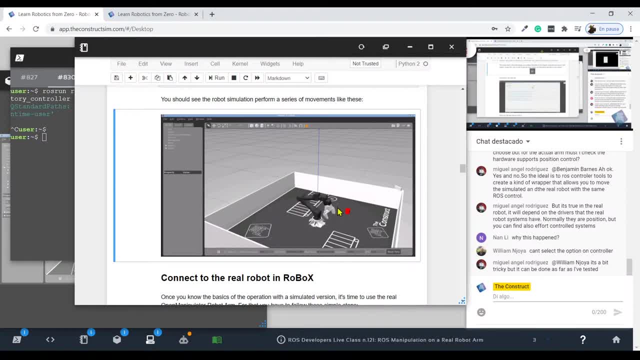 Something like this, like this behavior that you can see here in the GIF attached to the notebook. So we are going to- So we are going to do this using a Python script. In our Python script, basically, we are going to start sending our robot, or more precisely, the joints of our robot, to different positions. 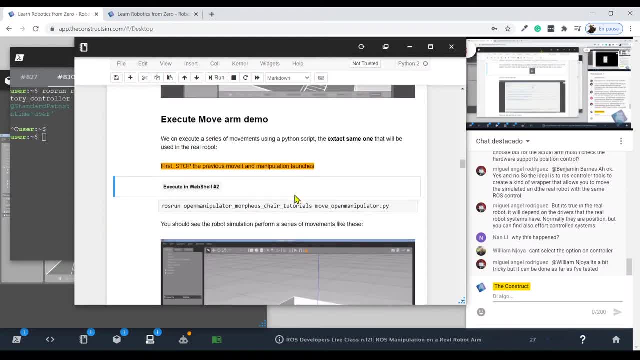 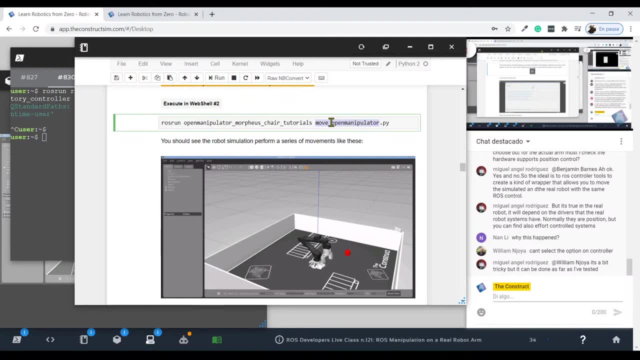 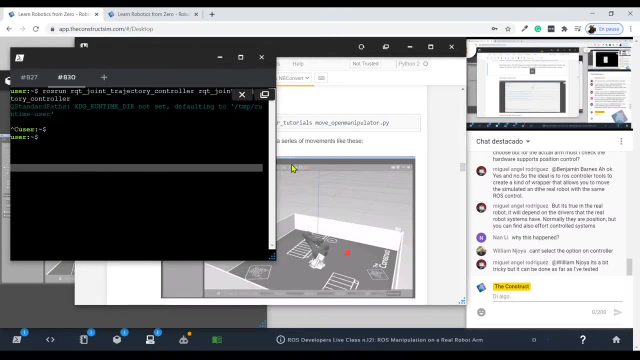 All right, Then, before actually running, So basically, in order to execute this script, all we have to do is to copy it here from the notebook and paste it here to the shell. Okay, But but before actually executing this script, I want to review it a little bit with all of you. 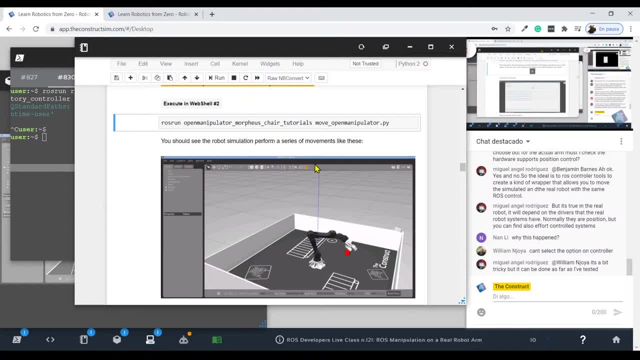 Okay, So that we can understand the script, what it is doing and what we expect from it. So, in order to have a look at this script, we are going to open the IDE, The IDE of our environment, which is this button here. 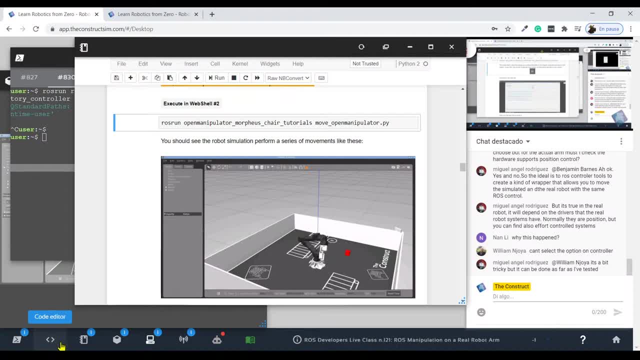 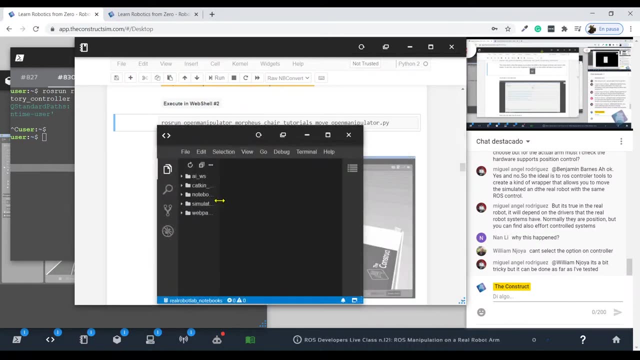 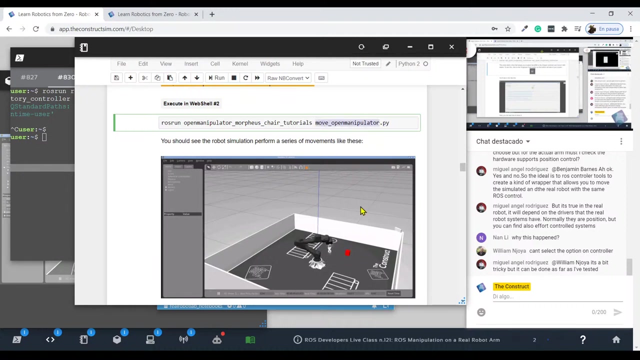 Okay, These two, these opening and closing tags. here, which is next to the web shell icon, It says code editor. as you can see, I'm going to click here and this is going to open my development environment. Okay, So, as you can see, our script, which is named move underscore, open manipulator dot py. 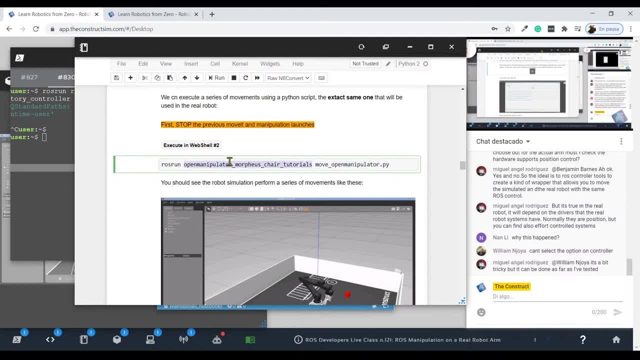 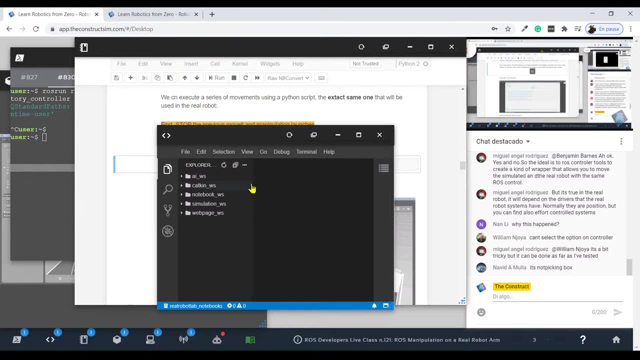 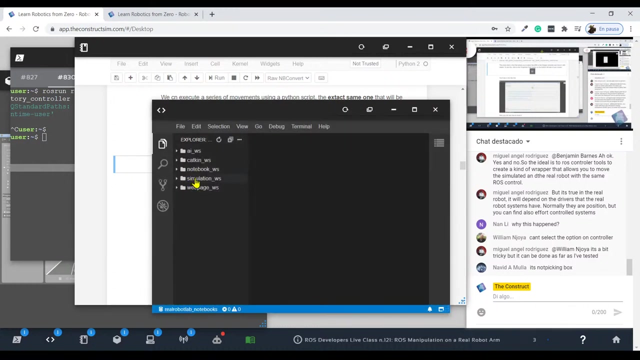 it is inside this Open manipulator: underscore Morpheus, underscore chair, underscore tutorials. So I'm going to look for this package in my workspace and since I already know where it is, I'm going to just tell it to you. So we are going to open, first of all, the simulation workspace. 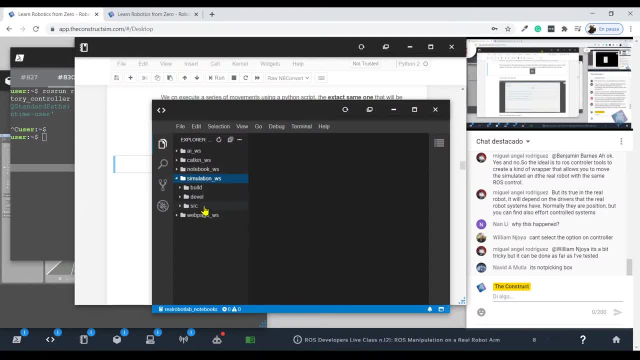 Then inside the simulation workspace, we are going to come here to the src folder And here you are going to see different packages: Mimic, join, Casivo, tutorial, open manipulator TC. And here we have a package which is named open manipulator underscore Morpheus underscore chair. 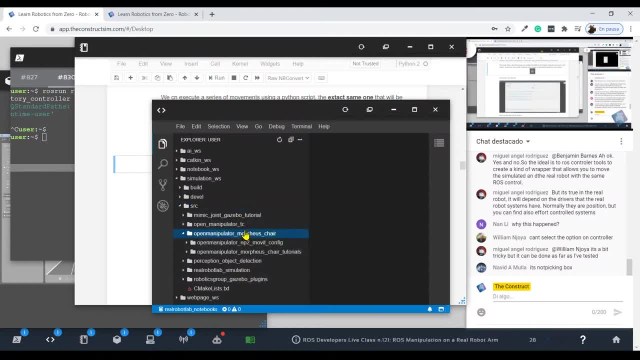 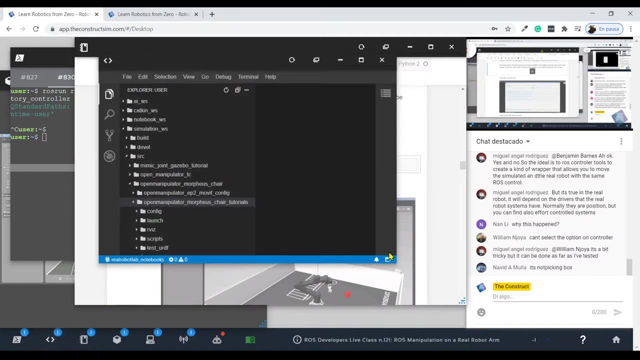 So let me open this and inside this folder we can see the open manipulator Morpheus chair tutorials package, which actually is the package that we are looking for. Then I'm going to open this And inside this package, here in the IDE, let me maximize the IDE for now also. 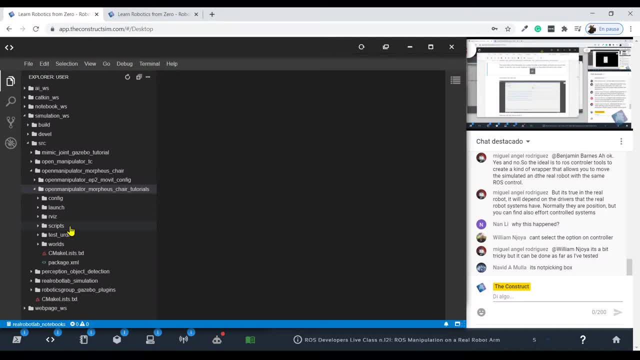 And here inside this package you are going to see that there is a folder named scripts here. So inside this scripts folder we are going to find the move underscore open manipulator dot py Python script. So if you double click on this it is going to open here in the IDE. 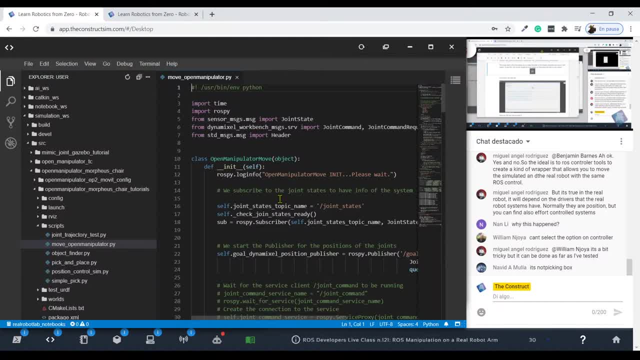 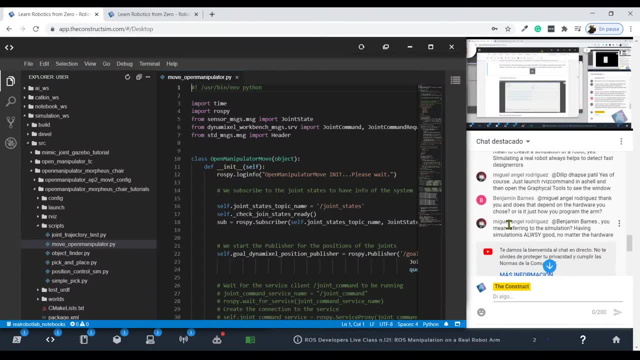 the code, And here you are going to find the name of this Python script. All right, Let me have a quick look here in the chat. I can see that Miguel is answering your questions. Thank you very much, Miguel, for the support. 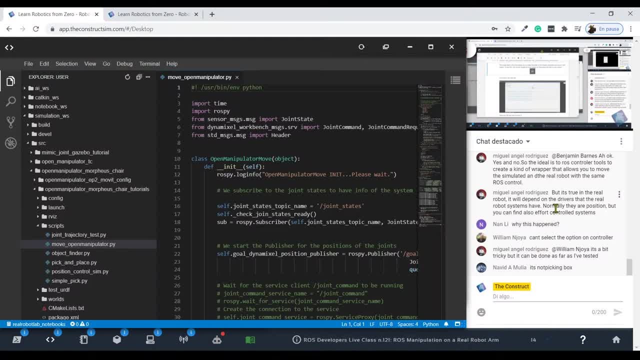 Why this happened. What do you mean? Lally, Lally? Ah, maybe you were referring to When I got disconnected by the real Robolab. Don't worry, this is not going to happen to you. It's not picking box. 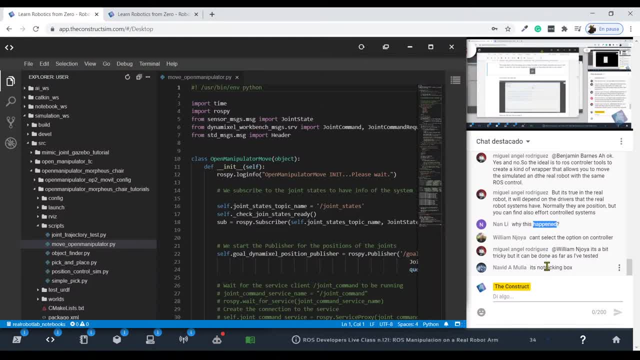 Yeah, yeah, yeah. It's not supposed to pick the box Now. it's not supposed to pick the box. The script, this script is only going to start moving the joints to different predefined positions. It's not supposed to pick the box. 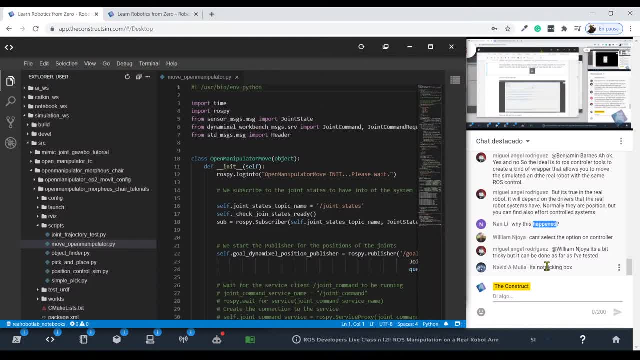 So it's not supposed to do the grasping here in this example, All right, So do you have guys this script open, all of you? Do you have it there open in your IDE So that we can review it together? 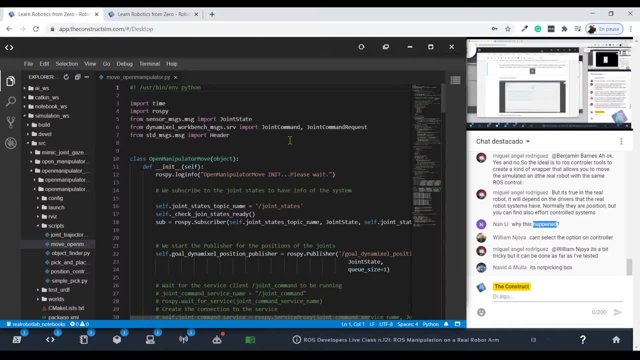 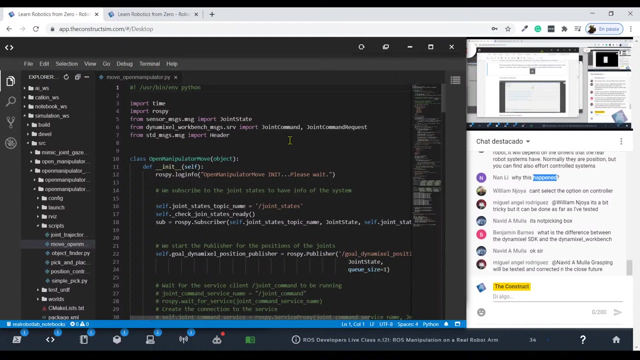 Yes, No, Let me know here in the chat. Okay, What is the difference? What is the difference between the dynamic cell SDK and the dynamic cell workbench? Well, it's basically the same. All of them are packages that are used in order. 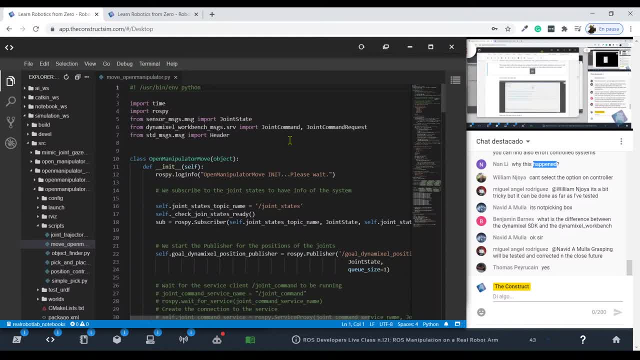 Are a set of packages that are used in order to control dynamic cell servos, which are the ones that this manipulator robot contains, So the dynamic cell workbench. it is contained inside the dynamic cell SDK That one is called. So the dynamic cell is a set of packages that are used in order to control the dynamic cells or the dynamic cells. 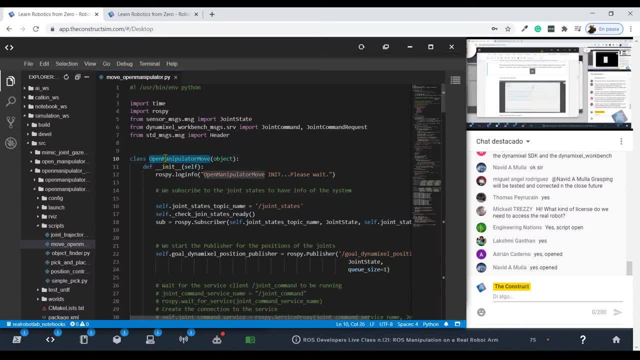 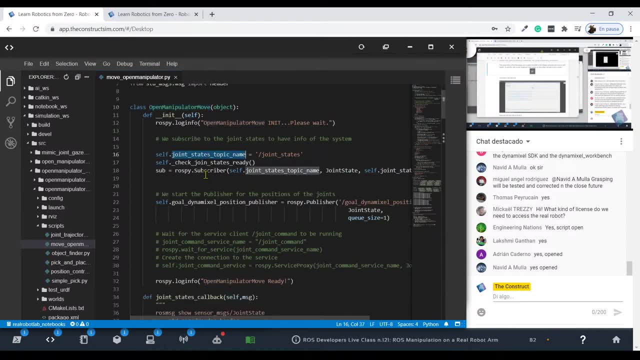 In order to allow this dynamic cell to move the target to a specific destination. Okay, So let's have a quick look here at the script, So you're going to see that it's super simple. So, first of all, we are defining our class, which is named open manipulator move. 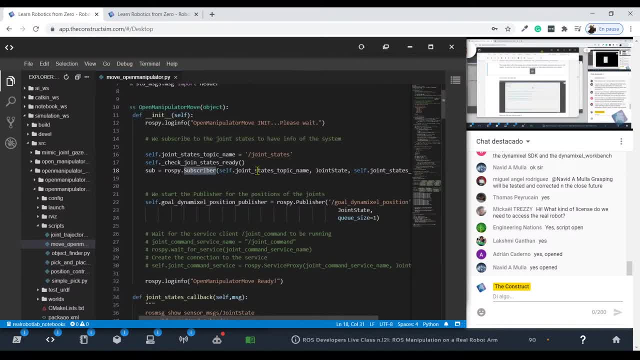 All right, Then what are we doing? First of all, we are defining as subscriber. subscribe to this topic, as you can see, The topic which is contained inside this variable, which is joint states. So, basically, here we are creating a raw subscriber. 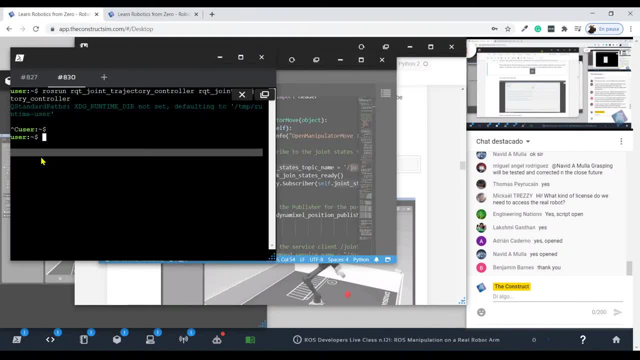 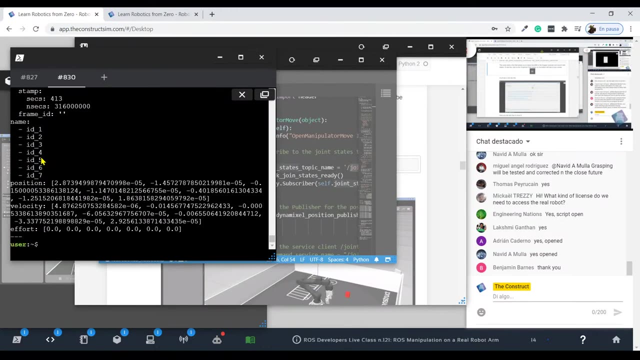 for the joint states topic. And what is this joint states topic? Well, we can come here to the shell and do a raw topic echo to the joint states topic. Let me do it. So, basically, let me stop it right now, As you can see, this joint states topic. 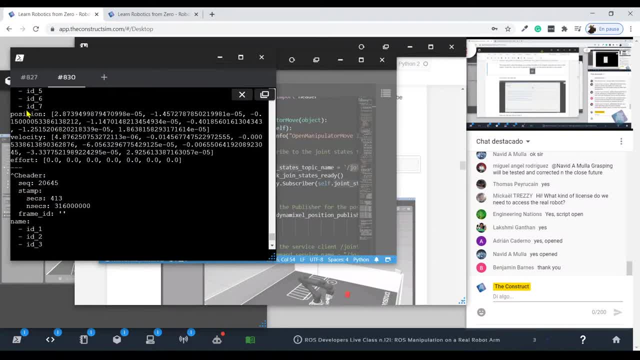 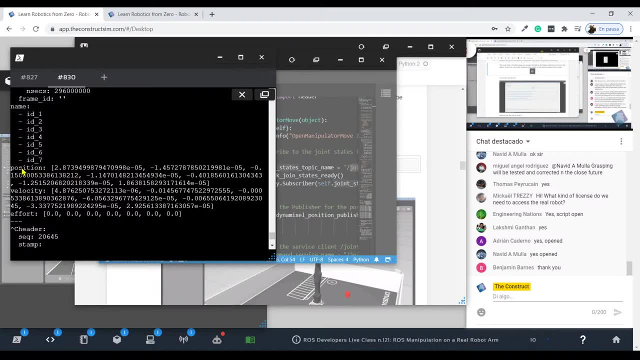 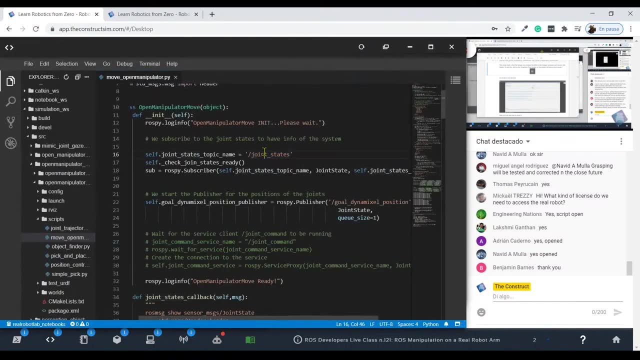 is going to continuously be publishing all the positions of my joints. Here I have the list of all my joints and here I have the positions of my joints. So basically, as the name says, this joint states topic is going to be continuously publishing the positions of my joints. 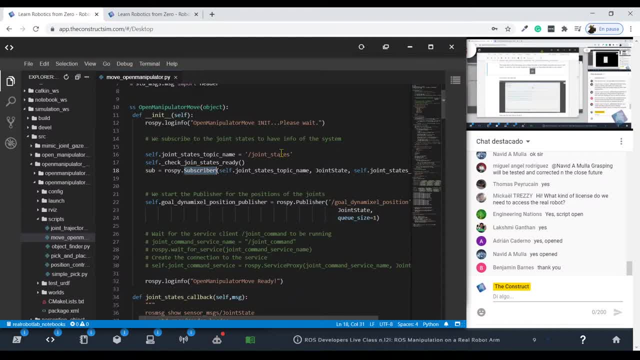 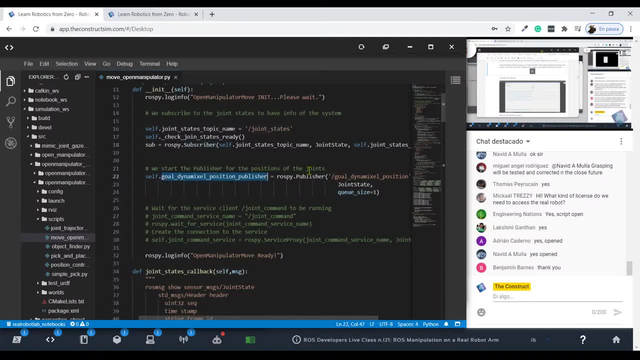 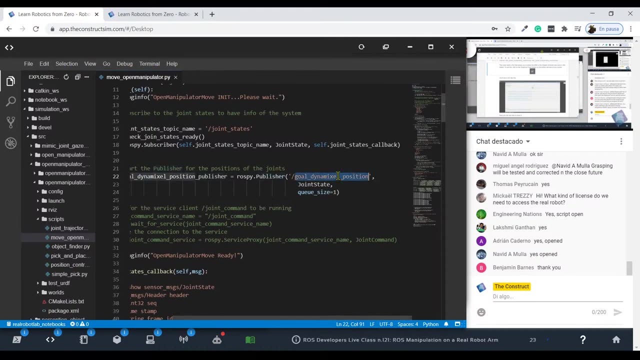 So I have first of all created a subscriber for this topic so that I know the information and the position of the joints of my manipulator robot, And also I am creating a ROS publisher here. I am going to be publishing into this goal dynamic cell position topic. 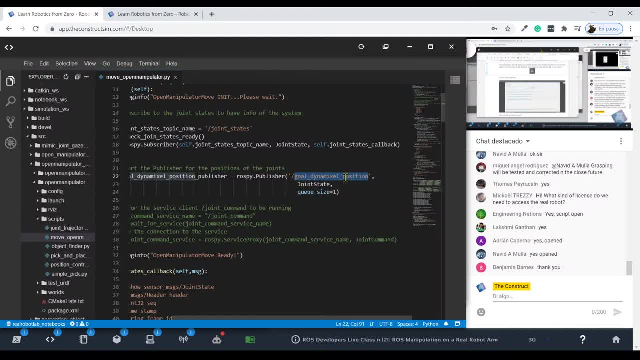 This topic is the one that I have to publish to in order to control the dynamic cell servos. so, in order to control the joints, Then by publishing messages in this topic, messages of the type joint state, I'm going to be able to control the different joints. 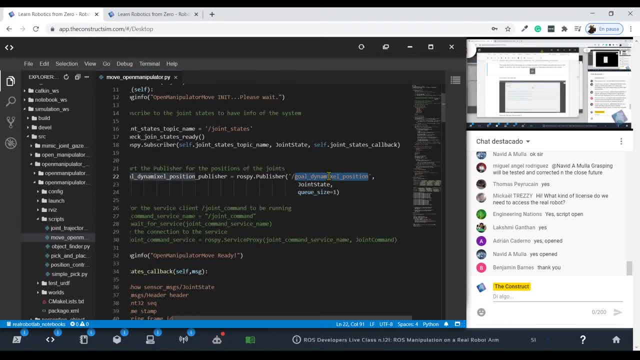 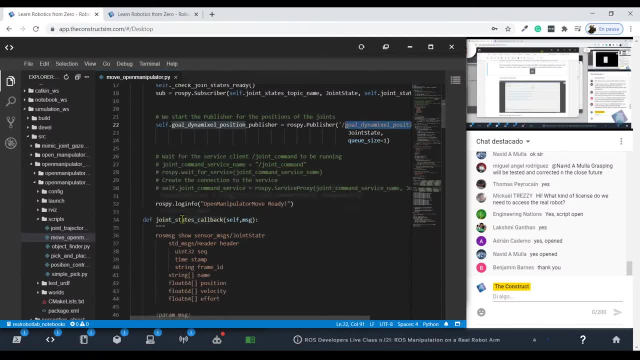 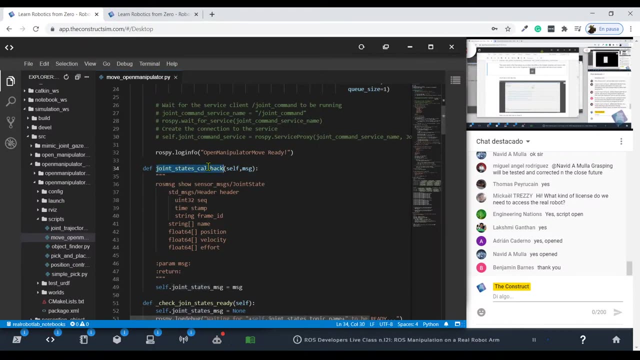 of the robot and move them to one position or another. All right, Let's keep going. Here I have the joint states callback, the callback. so every time a new message is published here into the joint states topic, this callback is going to be triggered. and here, basically all. 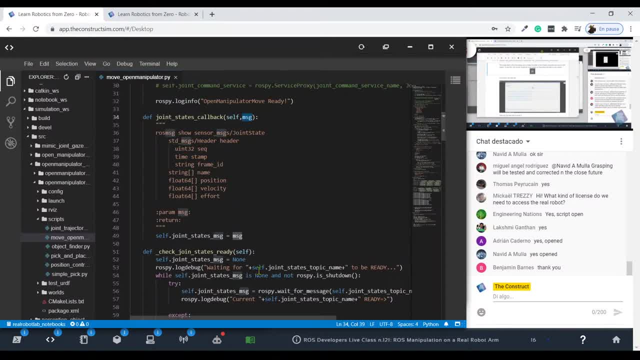 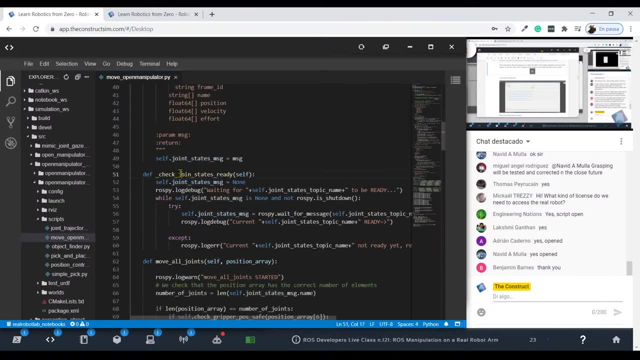 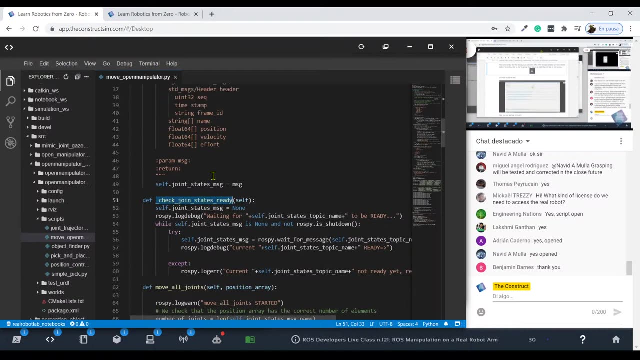 what I'm doing is to save the message which contains all the information of my joints here into this variable of the class, this joint states message. I have this function which says check joint states ready. so basically here I am just checking that the joint states topic- the joint states topic- is ready. 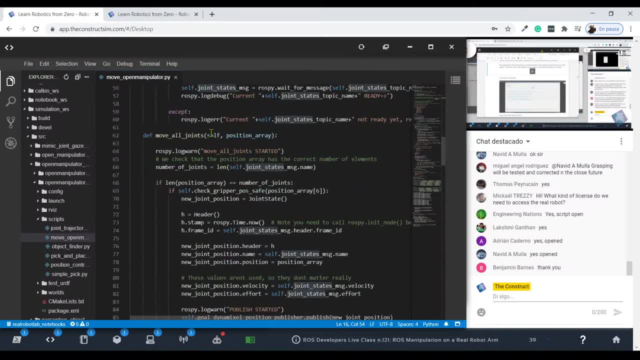 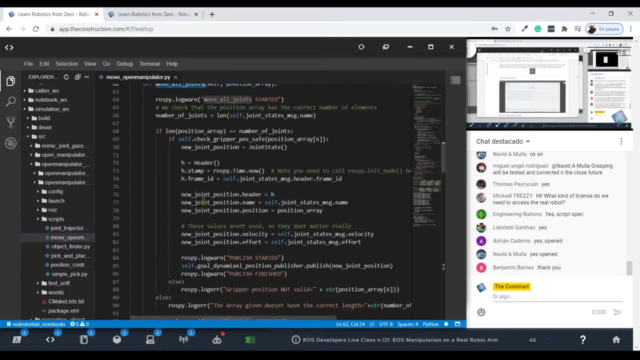 nothing tricky here. here I have a function named move all joints. so basically, here what I am doing is I am generating a message of the type joint state. as you can see, I am generating a message, a joint state message. I am filling this message with the header information. 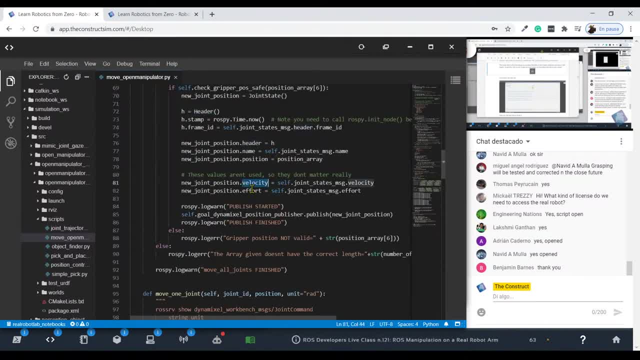 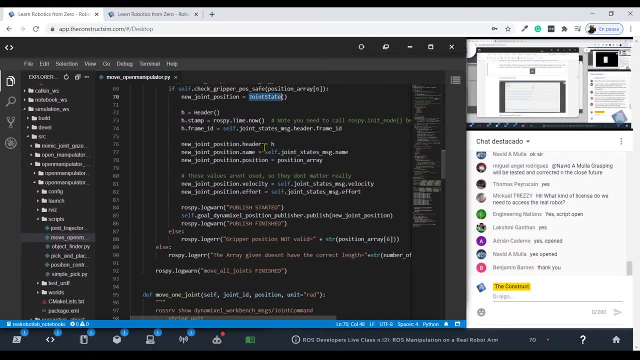 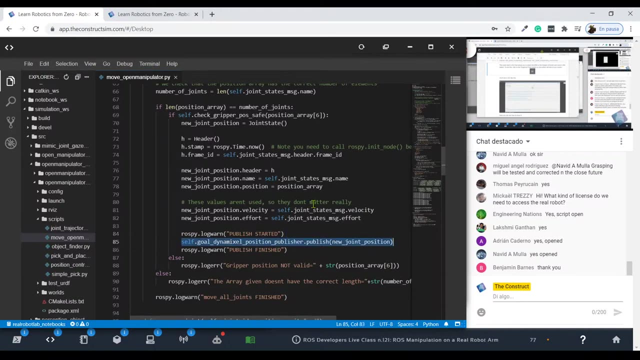 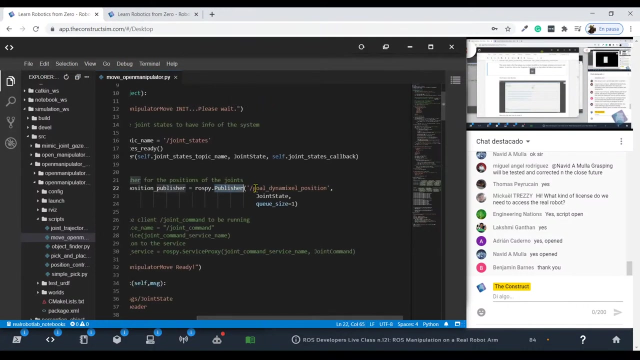 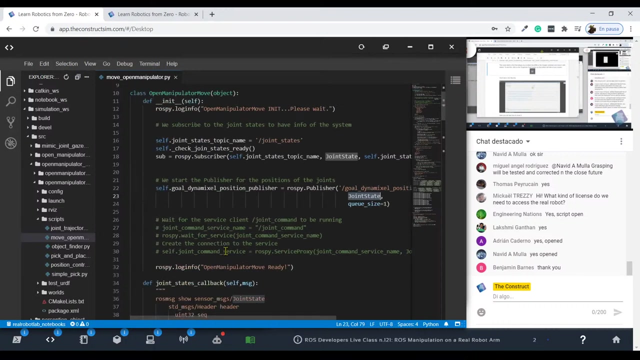 velocity efforts, positions of the joints, etc. so I create a message, a joint state message, and and I publish it here. yeah, remember, remember that we created here a publisher for the for this topic goal underscore, dynamic cell, underscore position which uses joint state messages. so basically, in this function, 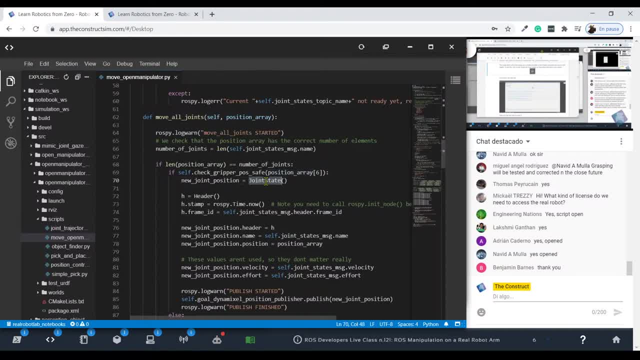 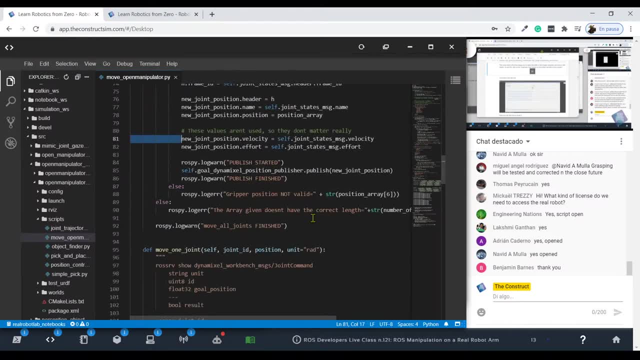 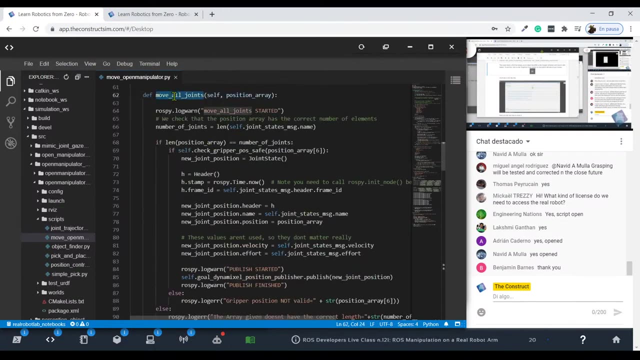 what I am doing is to create a joint state message and publishing into the topic. alright, so here I am going to move all the joints. so I am going to move all the joints, and then here, yeah, here, in this case, with this function, I am going to move. 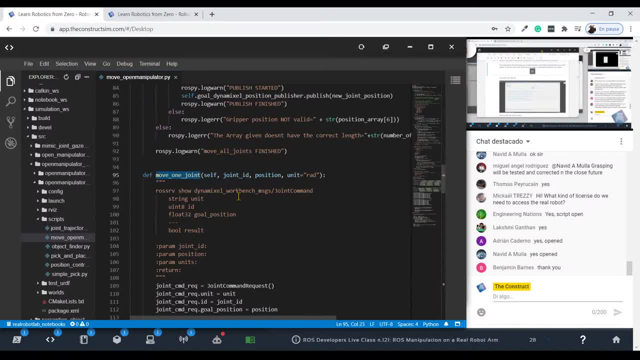 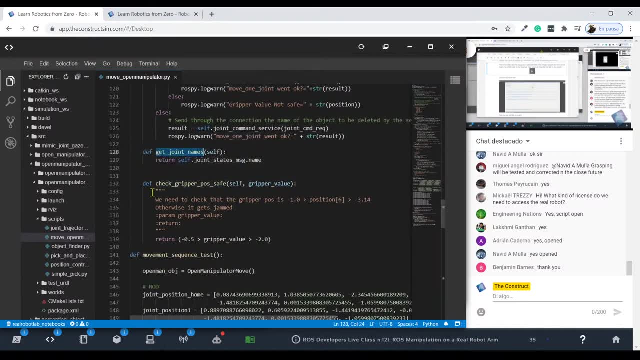 all the joints. here I have one function which is to move only one joint, so it is the same, but here I am going to move only one joint. here I have another helper function to get the names of the joints, yeah, the names of the of the joints. 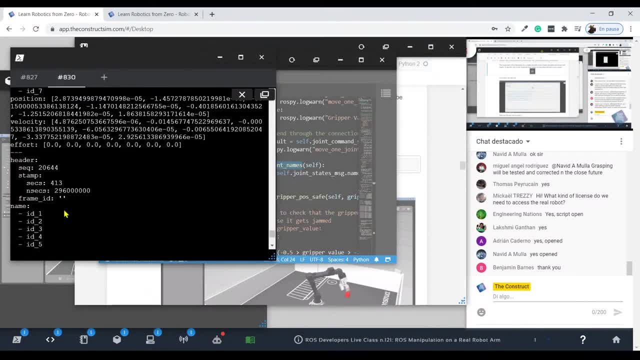 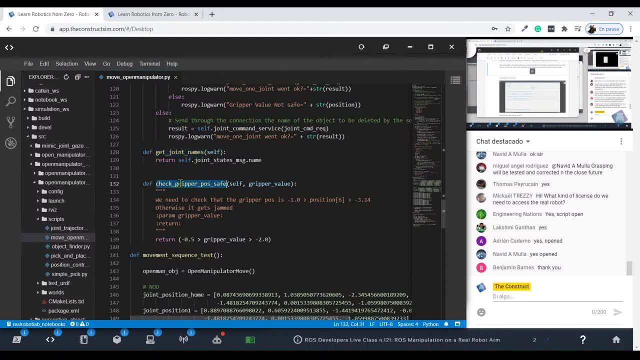 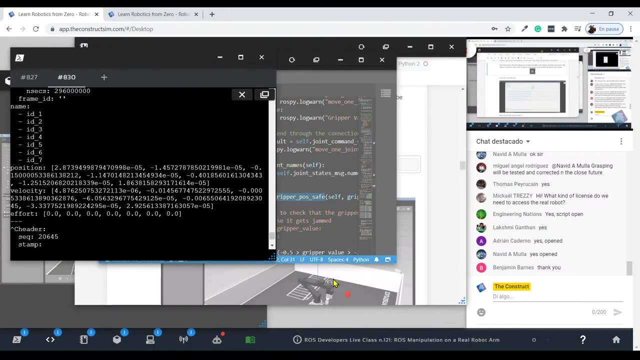 which you can see here: id1, id2, id3, id4, id5, id6, id7, id8, id9, id10, id11, id12, id12, id13, etc. so just a helper function. and finally another helper function: check gripper, post save, which basically is going to: 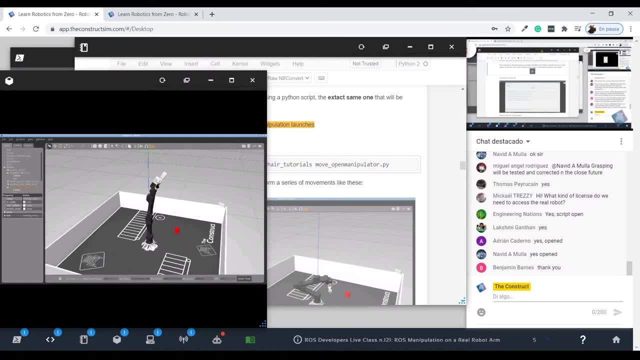 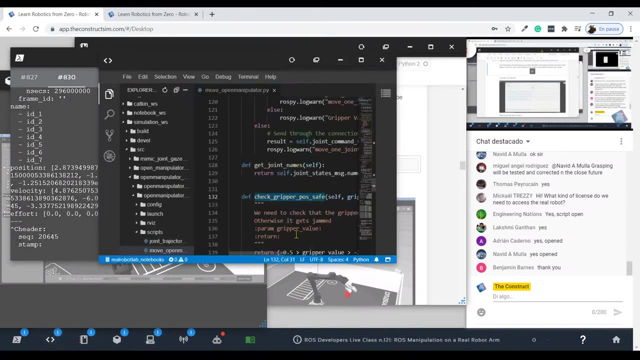 check. if the gripper position, if the end effector position of the robot, yeah, then the end effector, which is? which is this? yeah, this is the end effector of my robot. so, basically, this is the end effector of my robot. this function, sorry, this function. 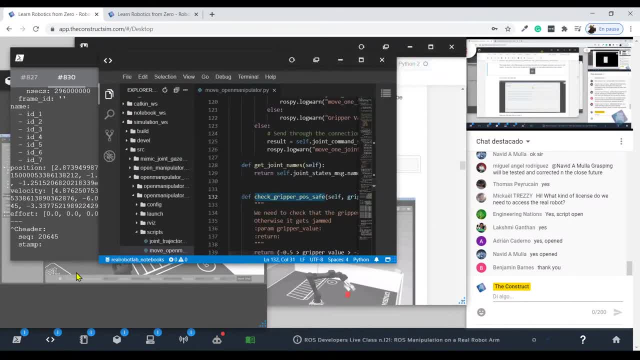 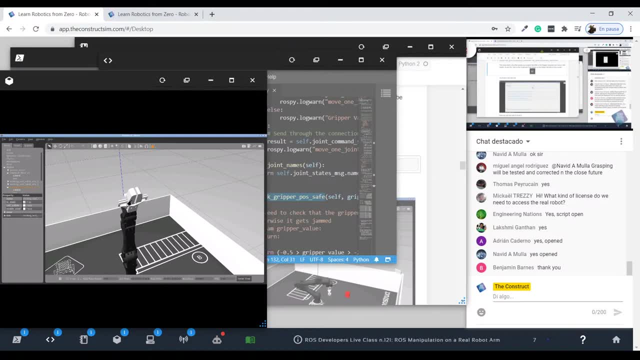 check. gripper post save is going to check if, by moving the joints of my robot, I'm going to put the end effector in a safe position, for instance. a position which is not safe would be under the ground, for instance. it's not possible to reach that position. 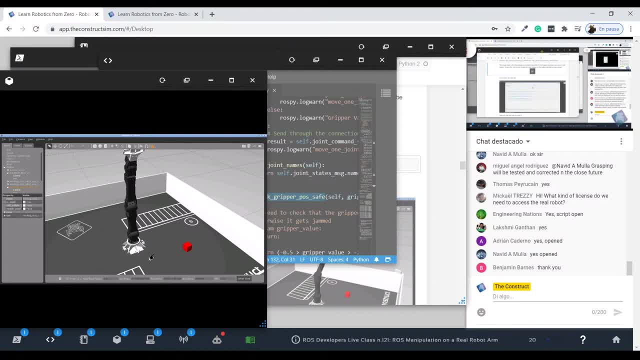 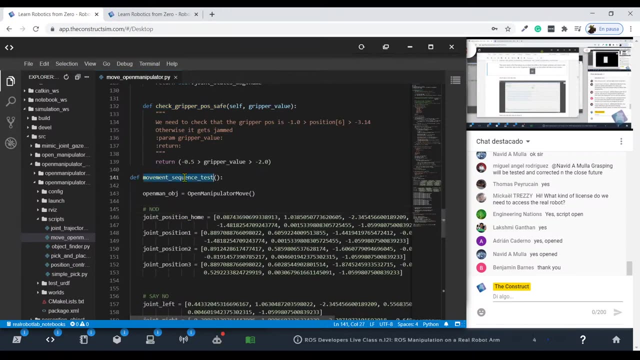 for the robot. so it's not safe. okay, because by moving to that position I would make the gripper, the end effector of the robot, crash against something. all right then. finally, I have a couple of functions. one is movement sequence test and the other one is 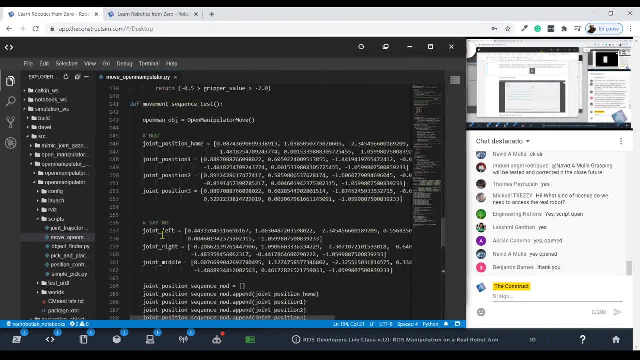 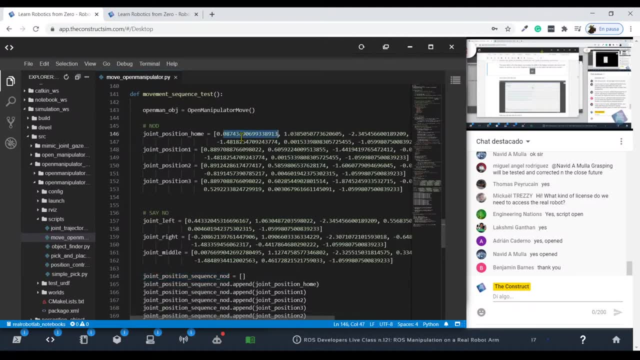 move joints test. so this movement sequence test. basically, what I am doing is to set different positions for the joints of my robot, as you can see. so here I have one set of positions. this would be the position for the joint: one joint two joint three joint four. 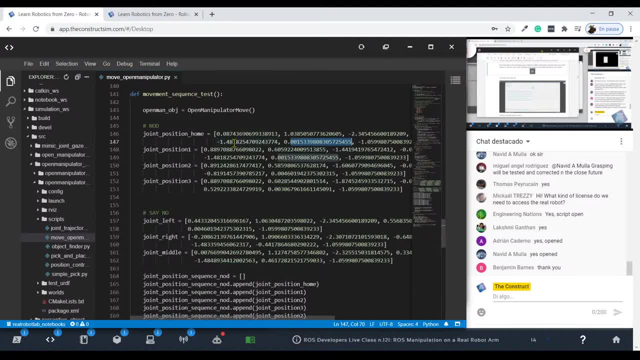 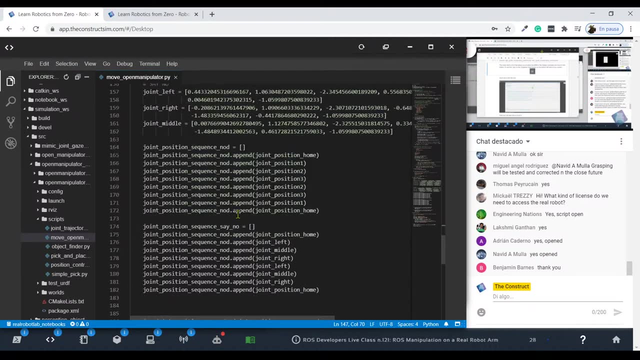 joint five, etc. etc. so basically, here I pass to my manipulator robot a set of positions to all of the joints, a sequence, let's say a sequence of positions for all the joints, so that it will keep moving from one position to another. and finally, here in this function, 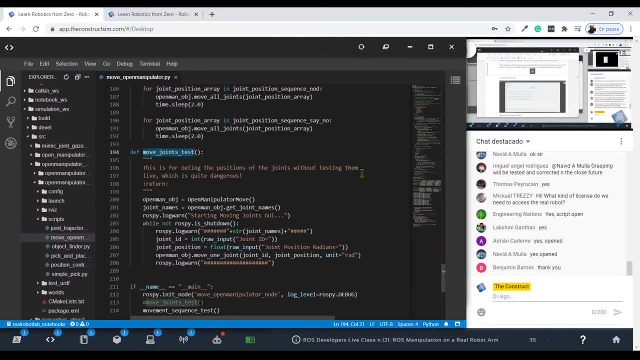 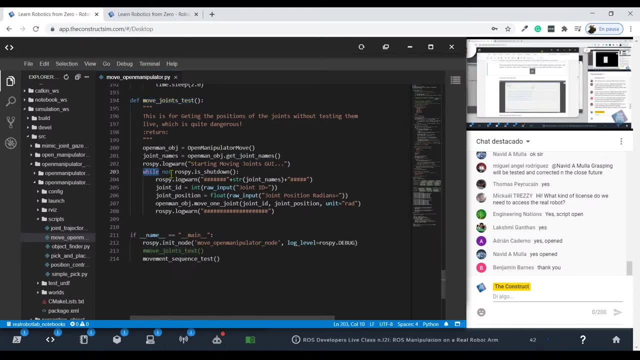 I have in the move joints test function. what I am doing is to I generate a loop, so meanwhile my program is not shoot down, so meanwhile I am not closing my program, for instance by pressing ctrl c. I'm going to call this move, so I will be. 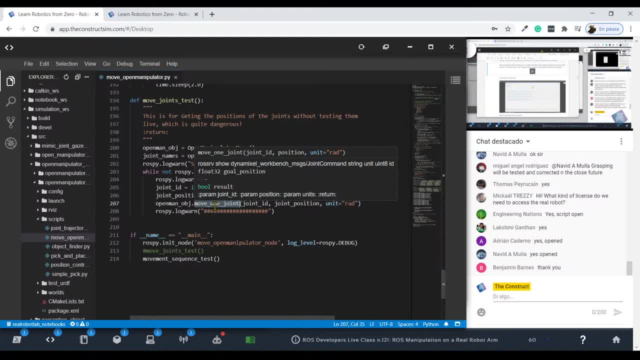 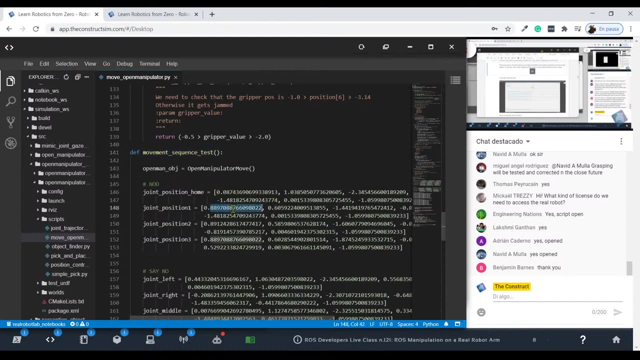 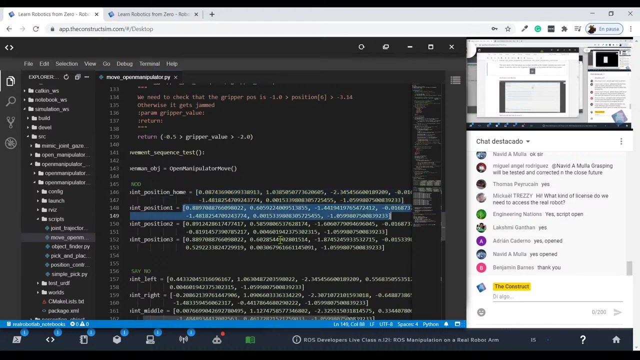 moving one of the joints of the robot continuously? yeah, so in this case, the function that we are going to test is the move sequence. test this one here. okay, so basically, we are going to pass different, different sets of positions to my manipulator arm and, more specifically, 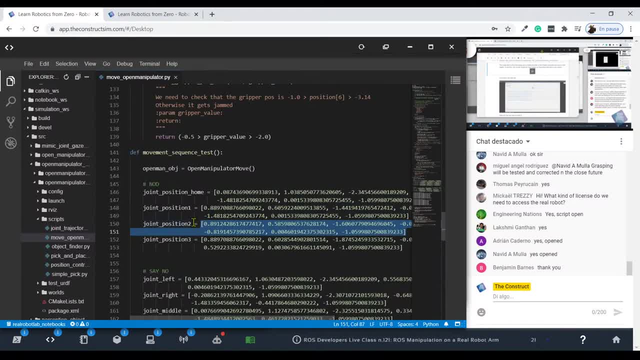 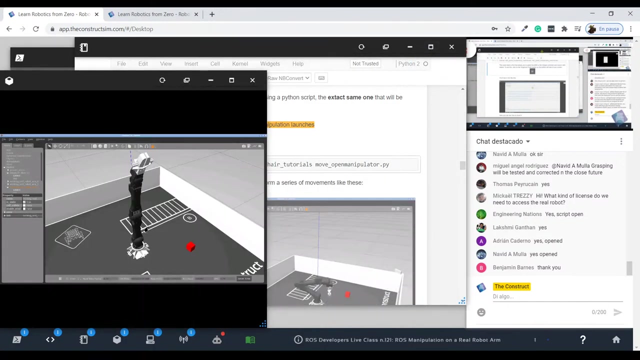 to the joints of my manipulator arm. all right, let me get a quick drink, since, since I am getting my throat dry. all right, then, once we have reviewed our python script, let's run it, let's execute it. so let me minimize this. let me put here: 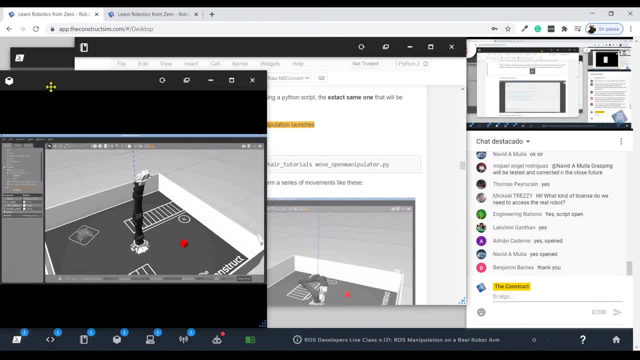 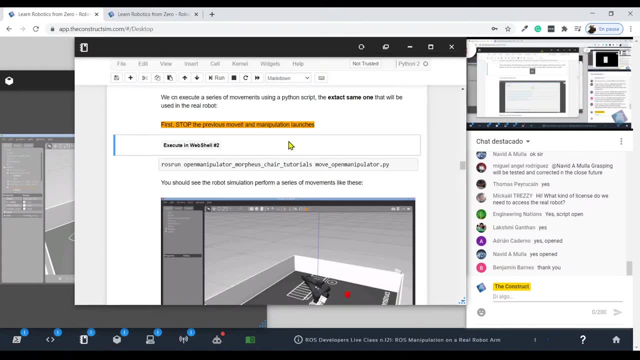 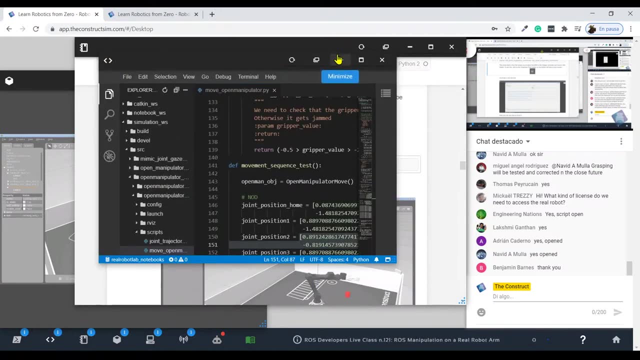 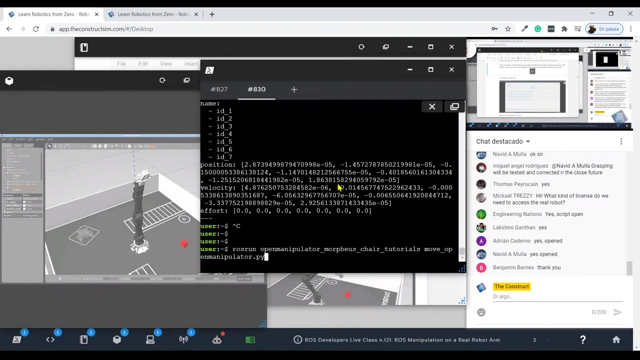 my simulation so that I can see it properly, and let me go here to the shell, and I am going to paste this command from the notebook into my web shell here. let me do it. yeah, rosh, run open. manipulators, morpheus, chair tutorials- move open. 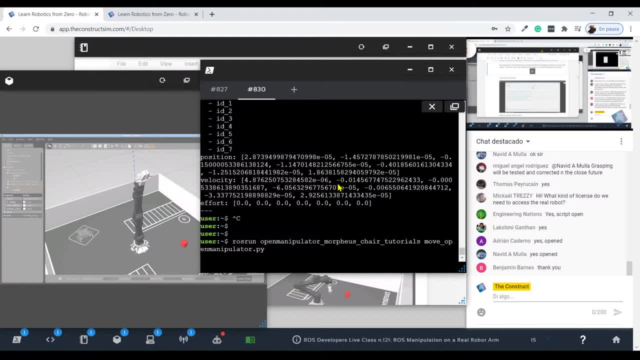 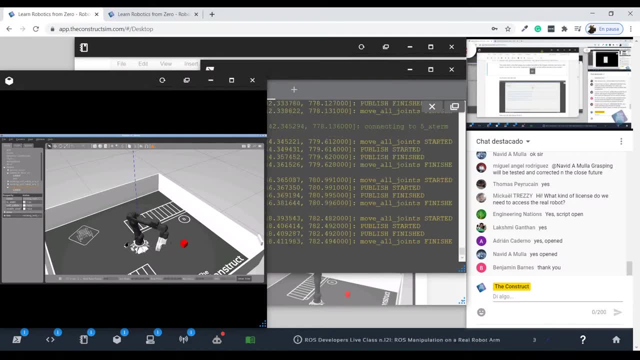 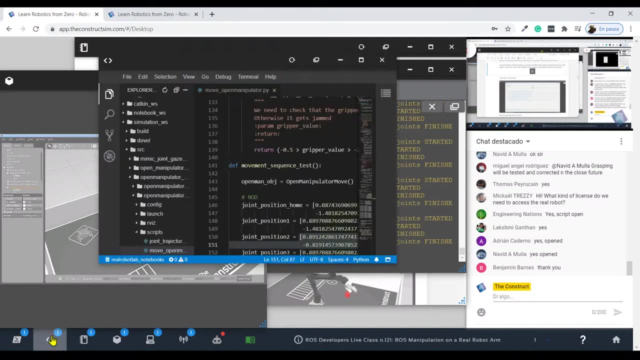 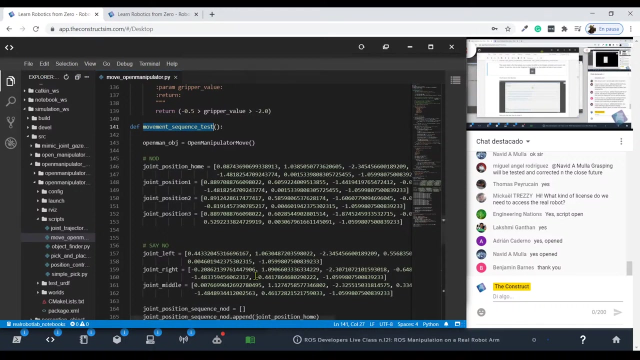 manipulator dot execute this script and we are going to see here in the simulation how the robot starts moving joints here in a sequence as you can see. so it's moving here the joints in a sequence as defined here in the movement sequence test function. so it's starting to execute. 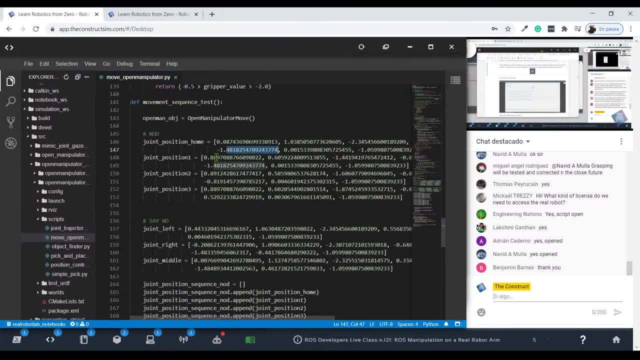 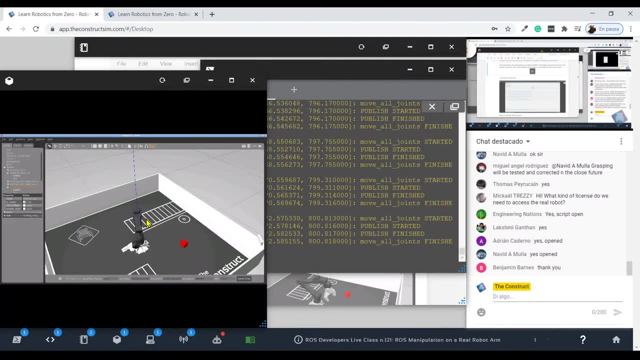 all these different positions that I am sending to the joints of my manipulator robot. all right, great. so everything is working fine. in the simulation, we can see that our manipulator is working properly, we can send positions to the joints and they are going to start executing here. 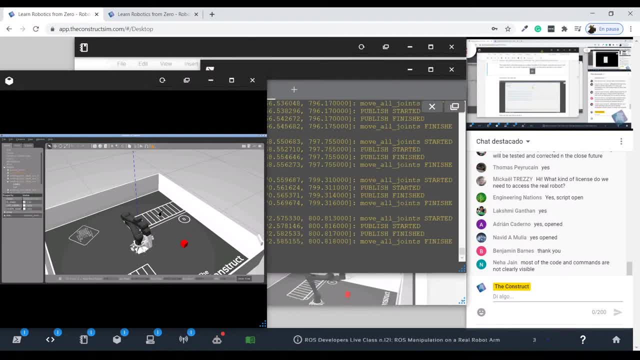 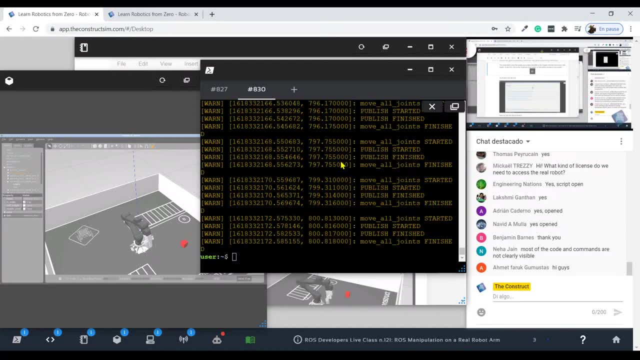 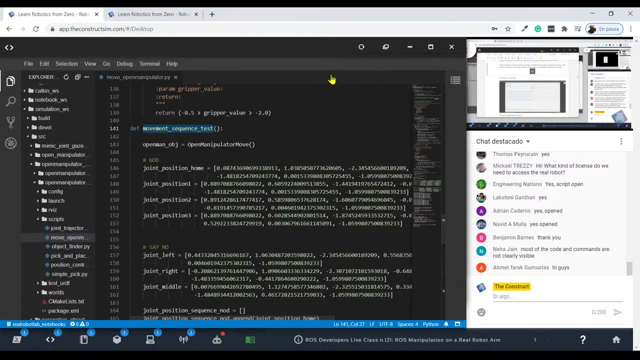 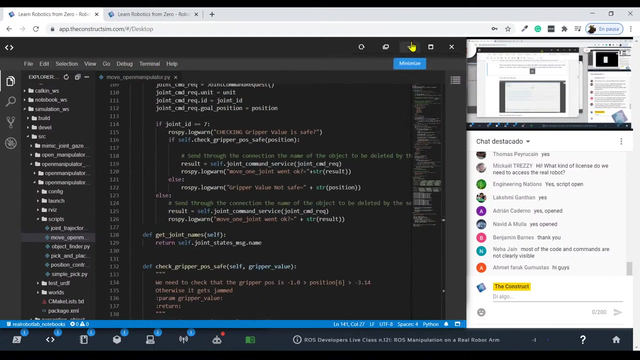 in the simulation- excellent. so what should we do now? well, what we are going to do right now is to execute this same script here. we are going to execute this same script in the real robot. so now we have executed it into the simulated gazebo robot. but now 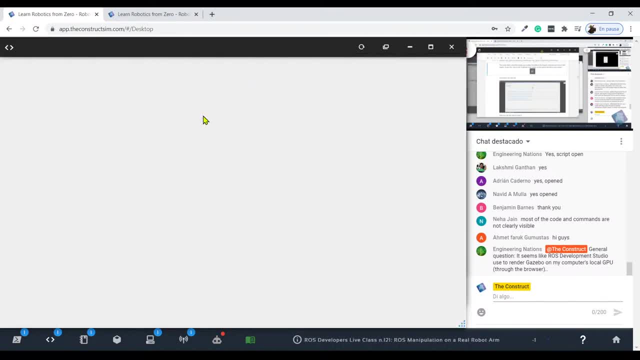 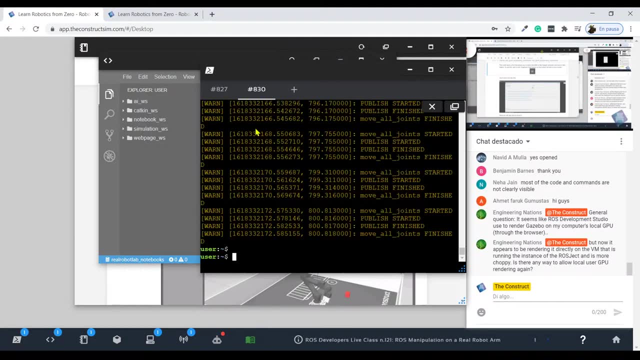 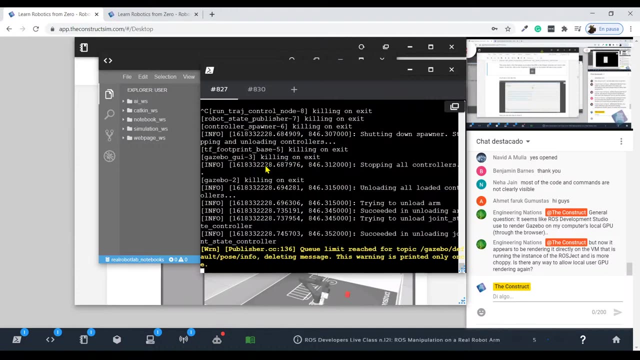 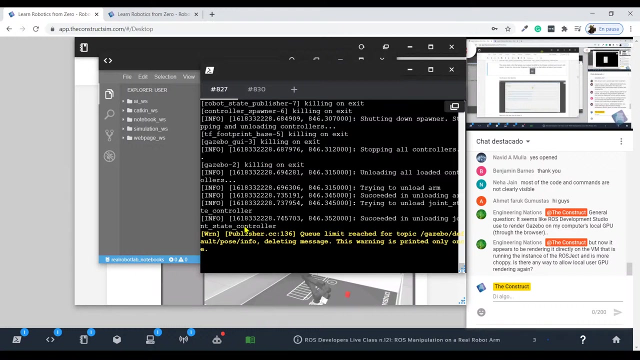 let's forget about the simulation. let me close it. let me close the simulation. let me come here and stop my simulation. also from here, let me stop it, and I'm going to connect to the real robot. so here I am, stopping the simulation. there we go. so 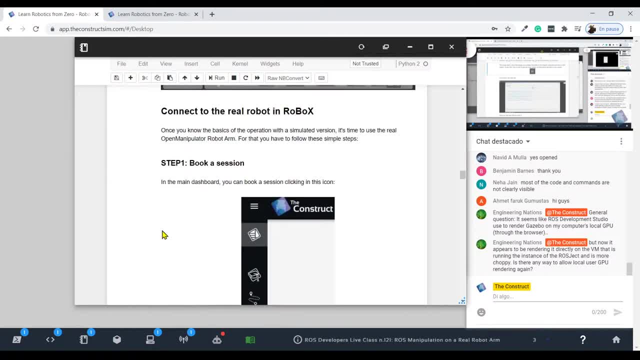 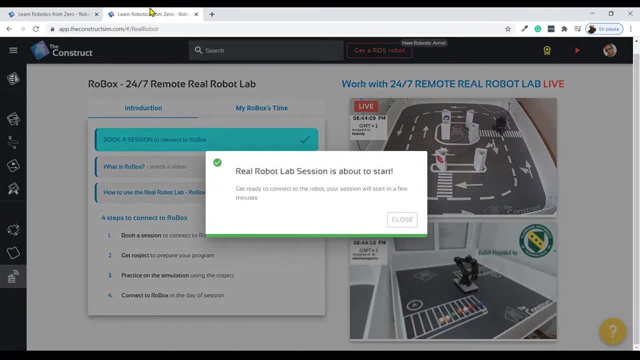 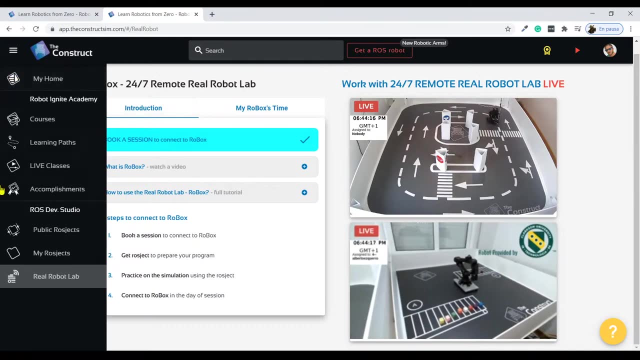 how do I connect? how do how do I connect? well, the first step in order to connect to a real robot, of course, is to have a session booked- right- I explained it before- of the live class. how to do this booking. so you have to come here to the real robot lab. 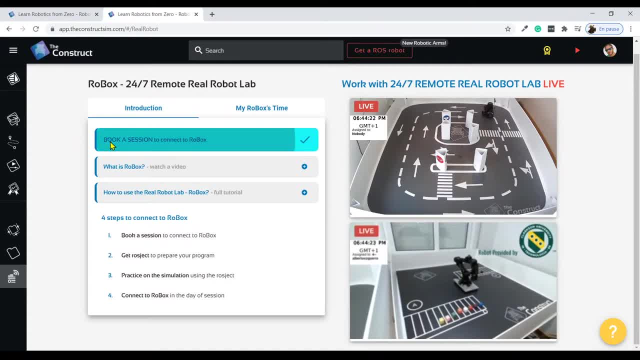 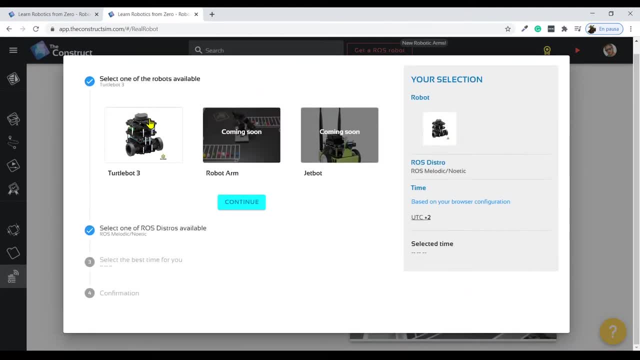 click here in the book a session to connect to robots and then you can select the robot. in this case I have selected. so right now you only have the turtlebot 3 option, but remember that tomorrow we are going to activate for free this robot arm, so 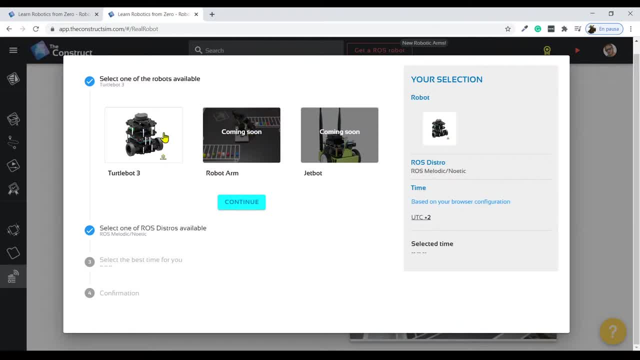 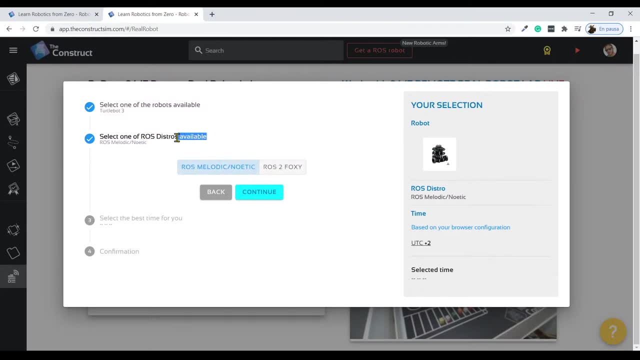 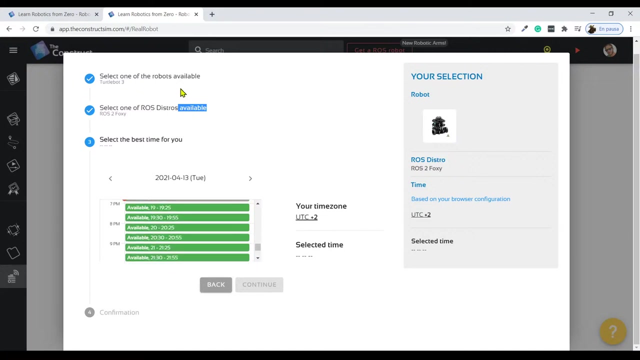 basically, you would come here, you would select the robot you want to work with, the distribution you want to work with. for the turtlebot 3, we have ROS2. for the manipulator: no, we only have noetic for now. you select the distribution you want to work. 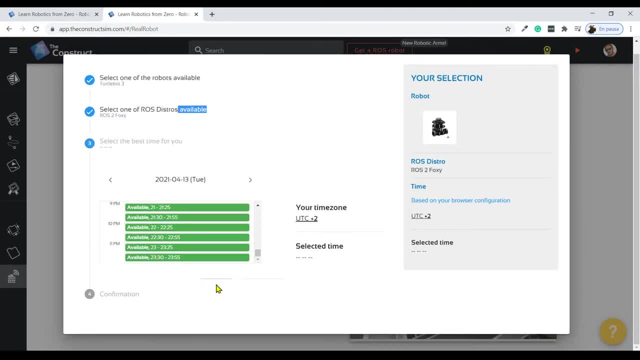 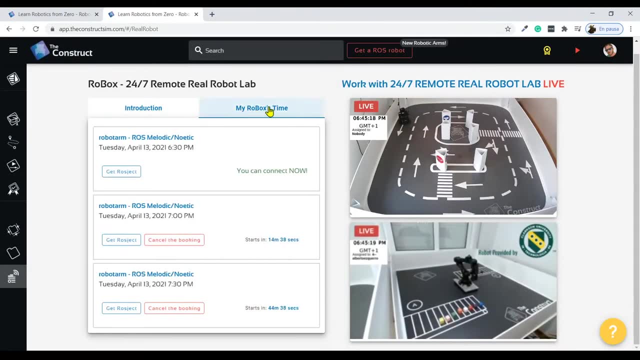 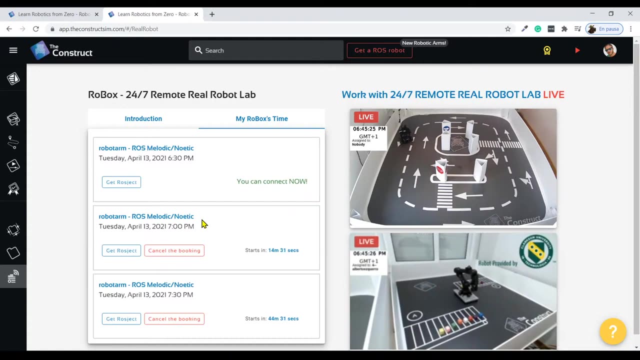 with and then you select the robot. you are going to be able to see your bookings here in myroboxtime. you are going to be able to see your bookings and remember you have two free bookings available, so you are going to be able to book two sessions. 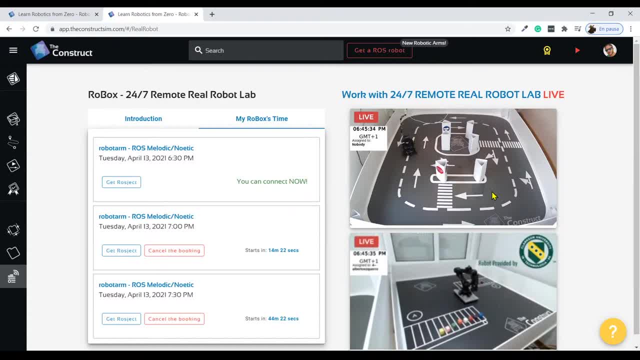 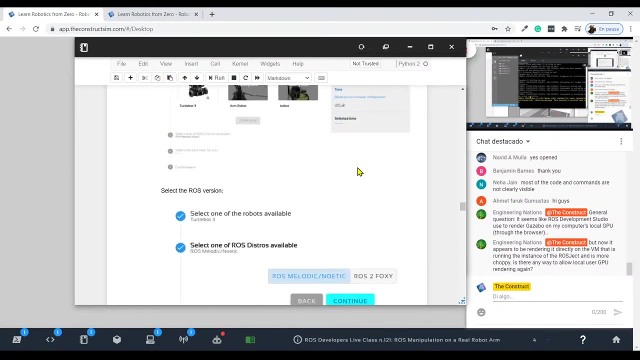 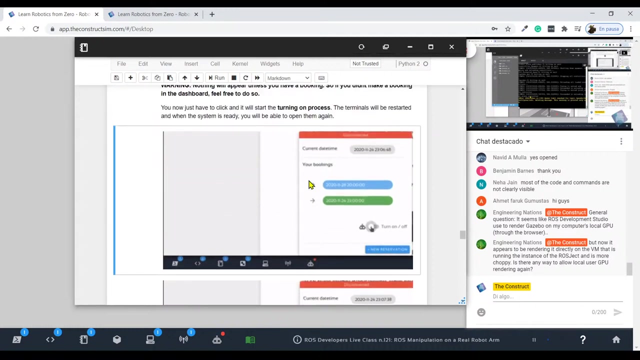 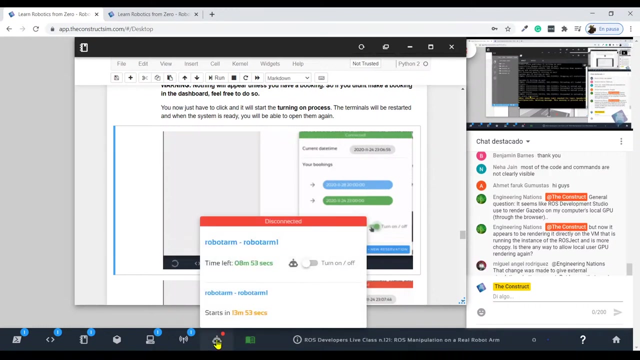 which the robot you prefer, completely for free, starting from tomorrow until the end, which says hey, you can connect now to the robot. okay, so once you have your booking, the next step is to click on this robot like icon that you are going to see here. you, you guys. 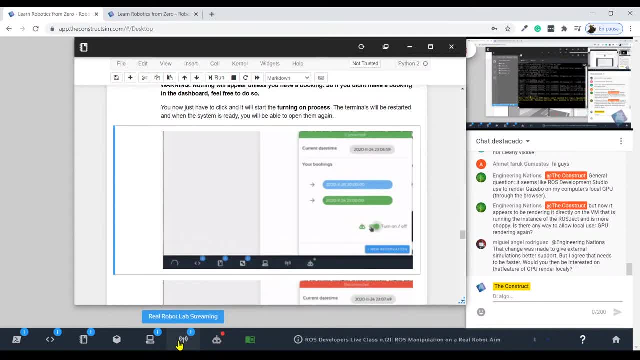 you are not going to see this icon, this: you are not going to see this one. for the person who has a session active for the real robot lab- okay, which in this case it's me. you don't have a session right now because i am connected to the lab. 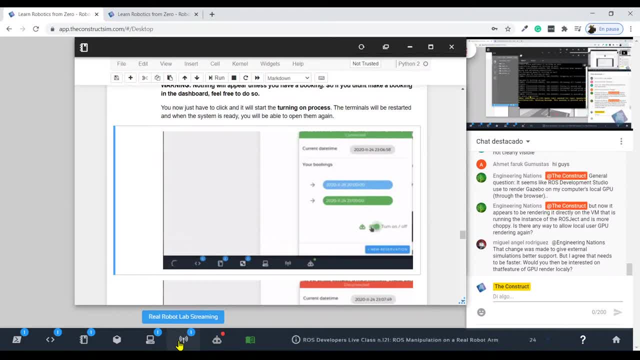 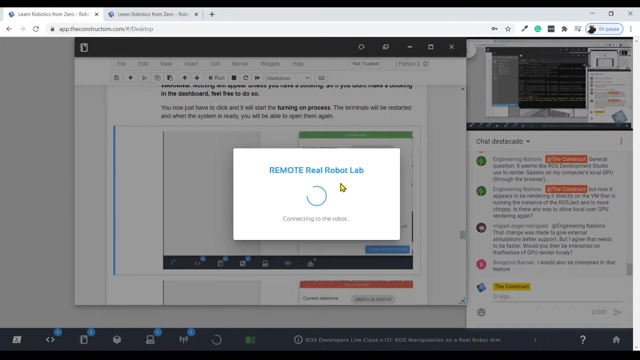 so if when you are connected to the lab and your session is active, so you are in the time of your book session, you are going to be able to click here in turn on off. so i am going to do it right now. let me click on the. 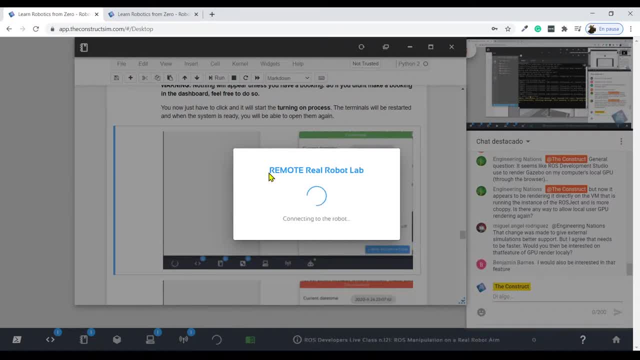 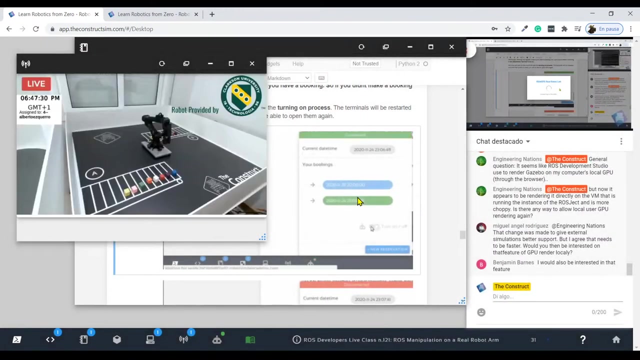 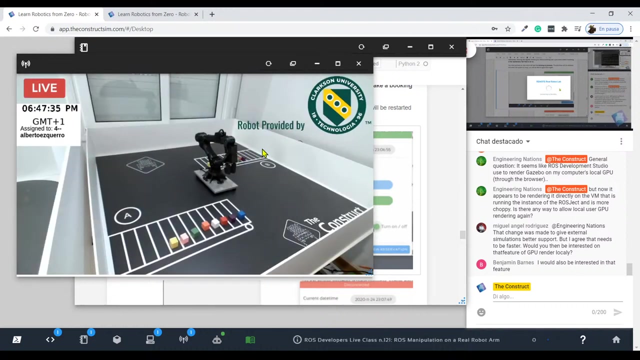 turn on button and this is going to start connecting to the real robot. as you can see, remote real level lab to the real robot. okay, let's wait until this connection is established. there we go. so now i am connected to the real robot and all of my 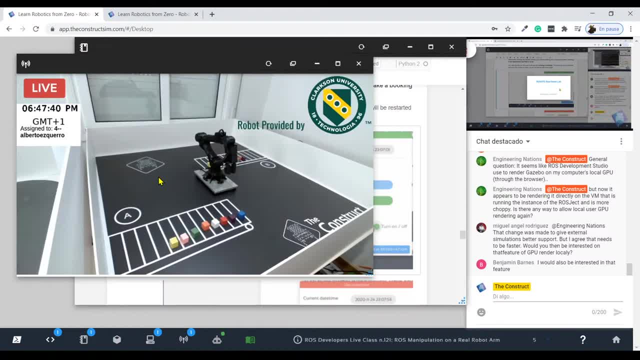 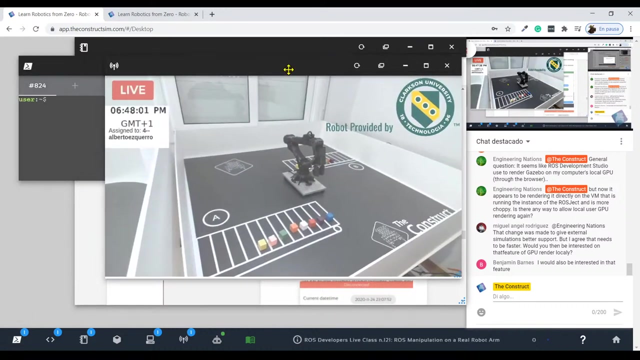 real, of my real manipulator robot, which we have here in our, in our offices based in barcelona. all right, this is a live streaming, so this is happening right now and, as you can see, alberto, which is me, i am connected to the robot, make sure. 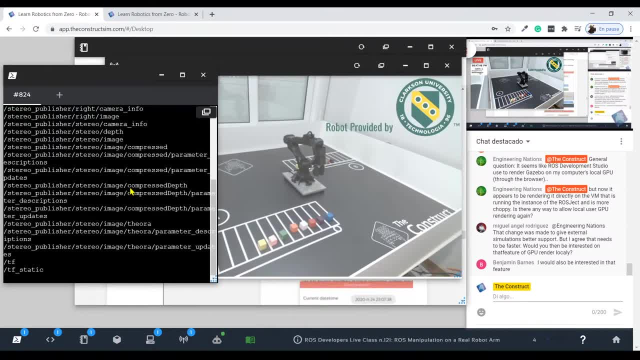 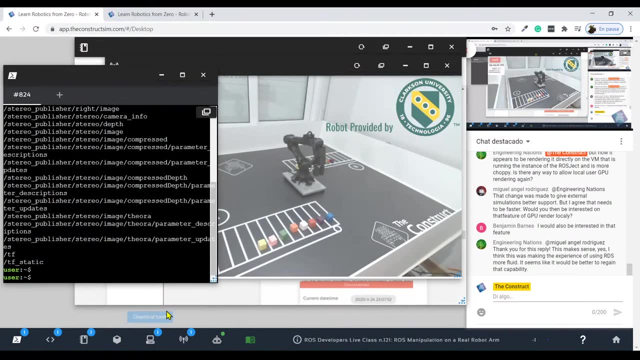 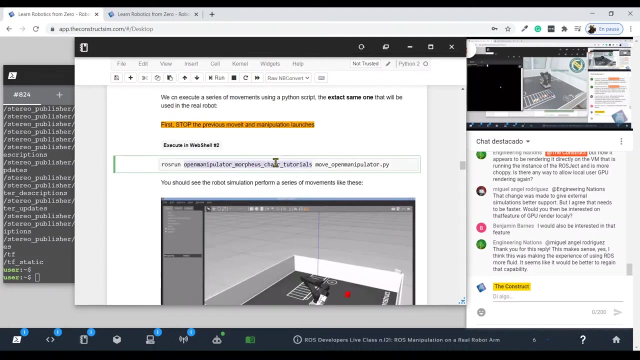 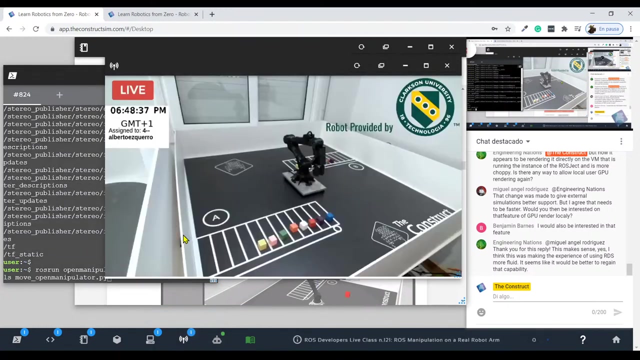 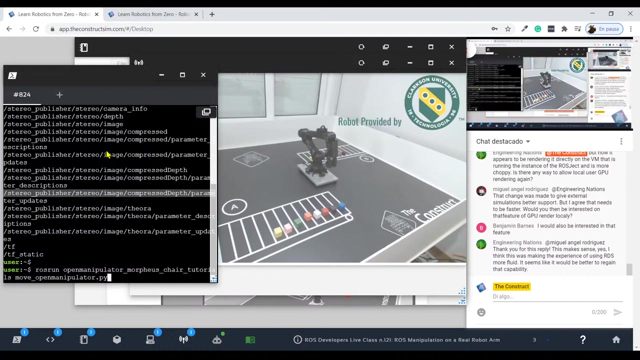 that everything is properly connected. so now, here i am, visualizing the topics of the real robot. okay, so i don't have any simulation running now. now i'm working on this one on the real robot and i'm going to run it, and now within some seconds. 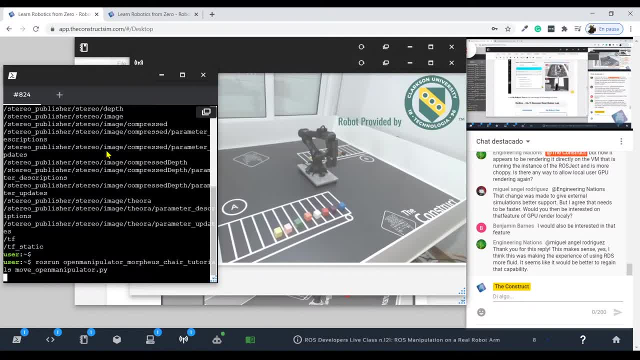 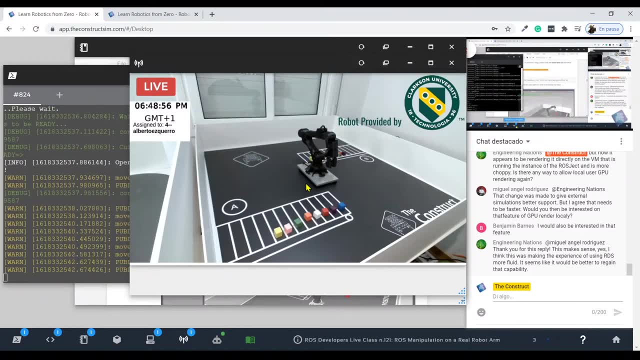 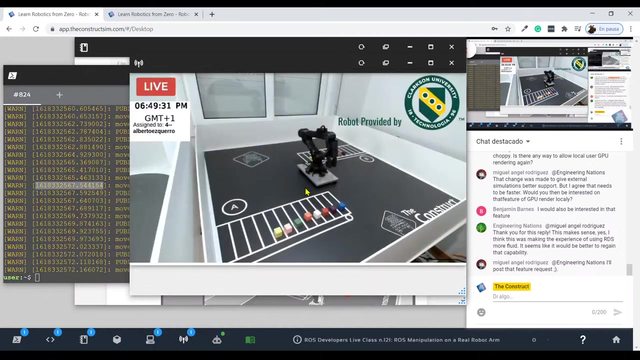 i should see the real robot start moving. it has some delay. the video. let's wait a little bit. they joined to different positions. let me see this is having this. i don't know if this is having a lot of delay or something is not working as expected. 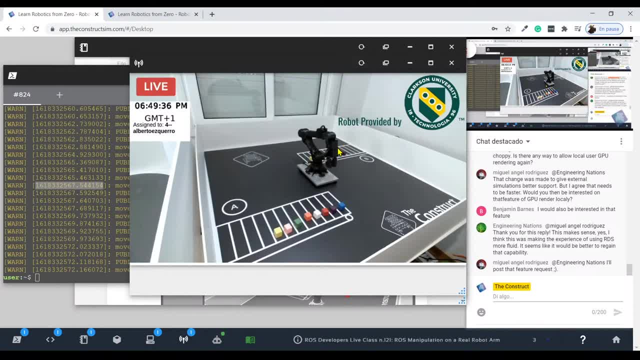 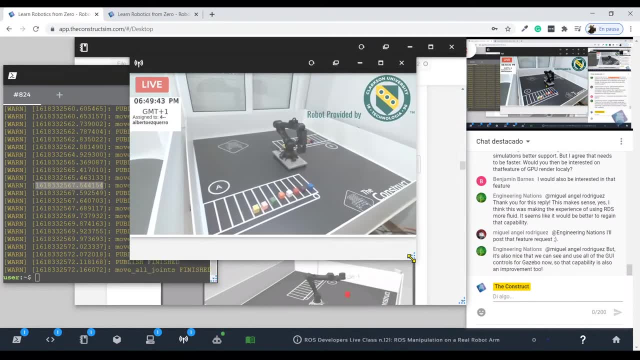 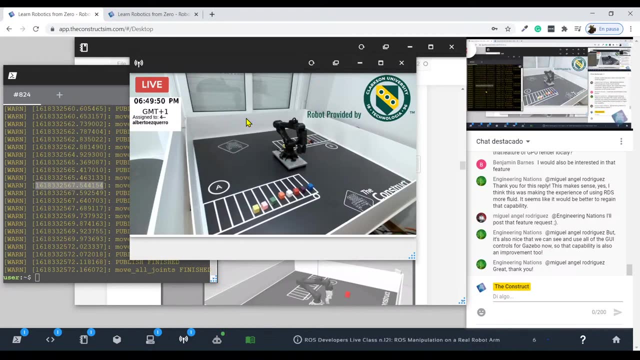 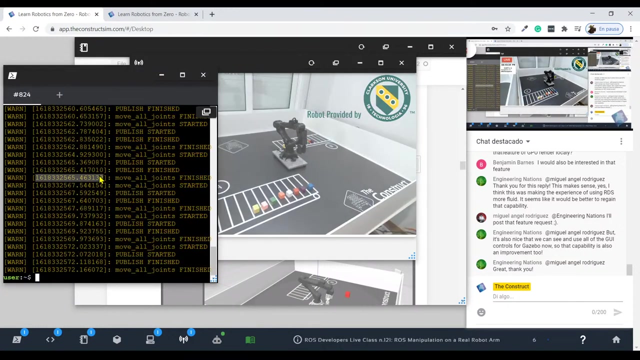 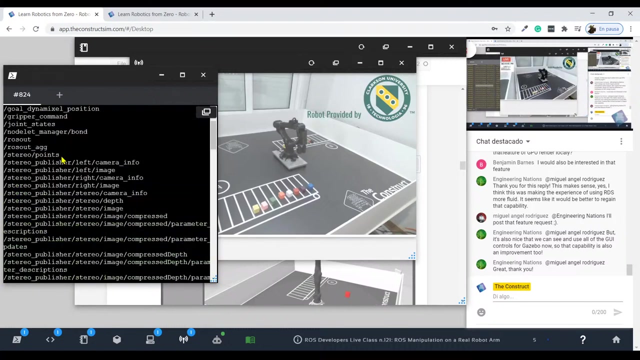 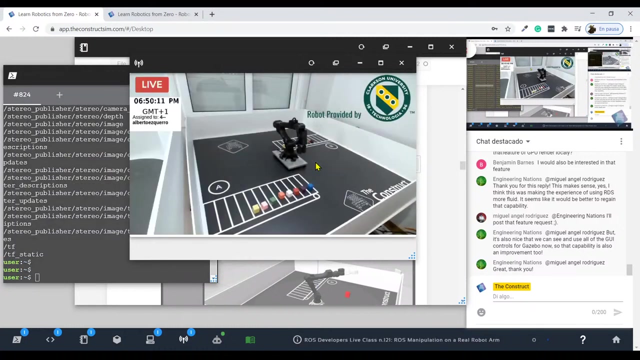 maybe it's the delay. yes, the robot is not moving for sure. let me see in. any work have worked fine here. cross topic list. let me see everything seems fine here. i don't know why it's not moving. this doesn't seem to be no, no, no. 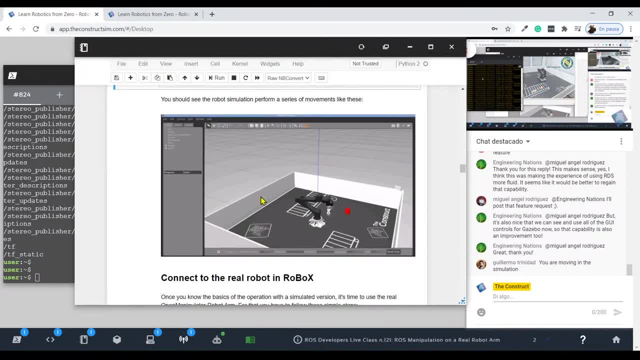 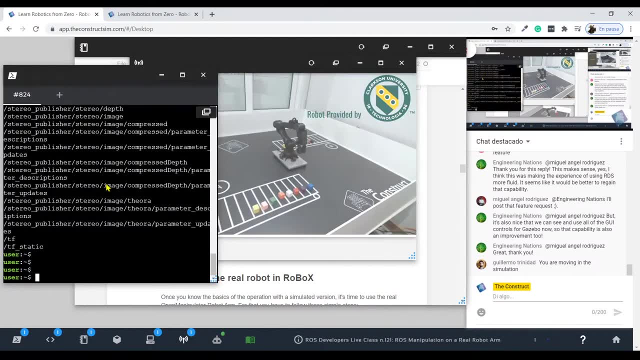 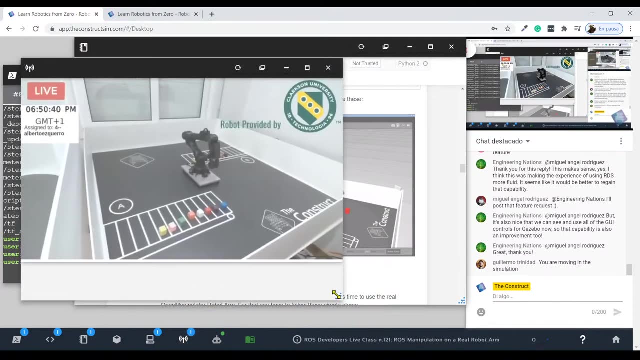 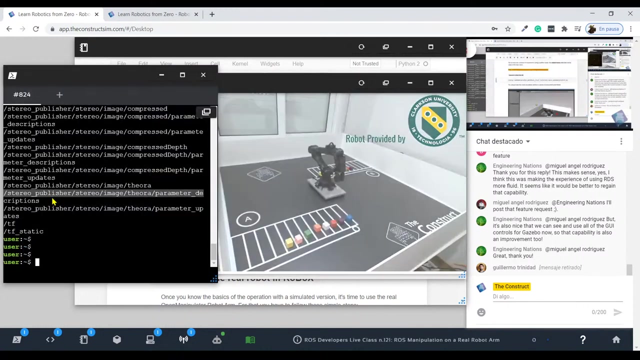 you're moving in the simulation. no, no, guillermo, this is. this is a gif of the notebook, the simulation. let me close this and open it again. let's see. try to read it one more time and see this is not working. let me try to read. 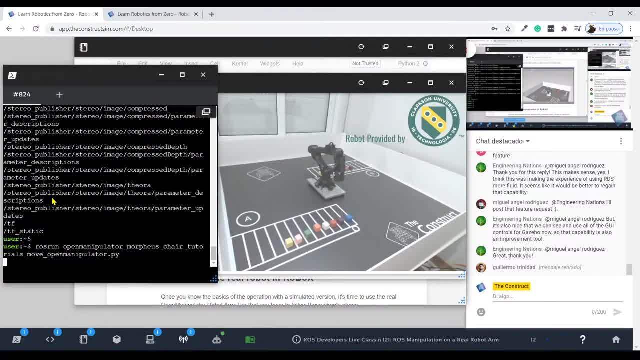 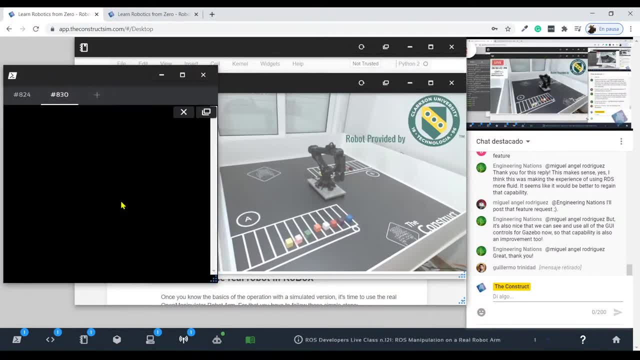 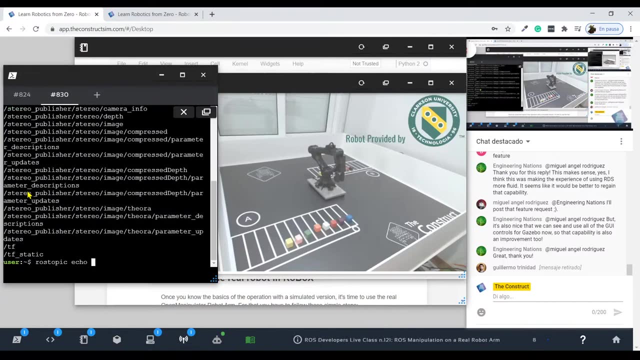 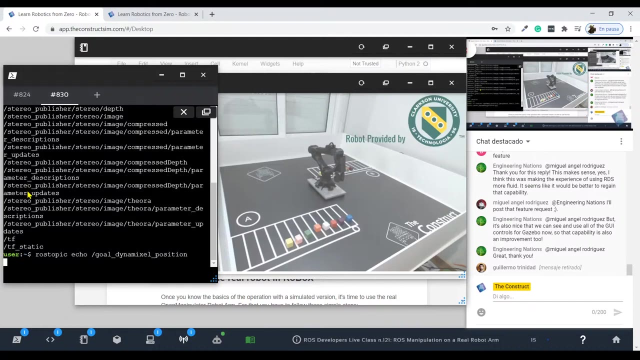 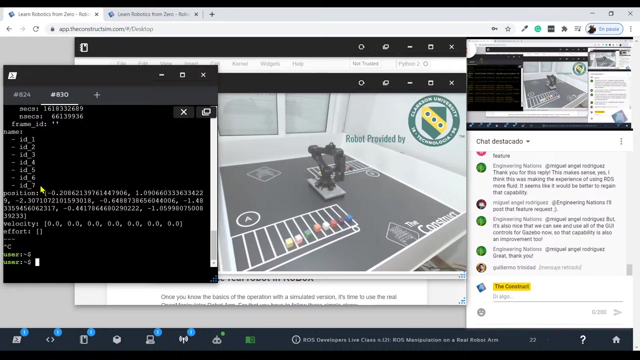 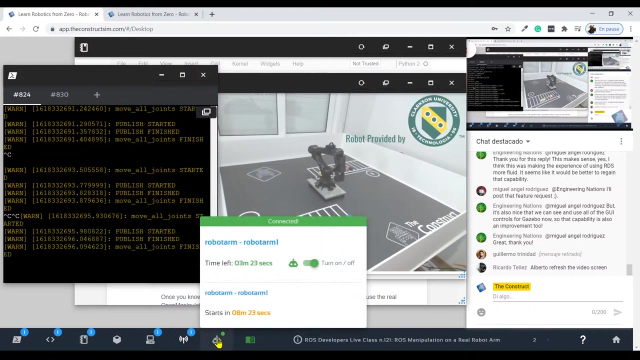 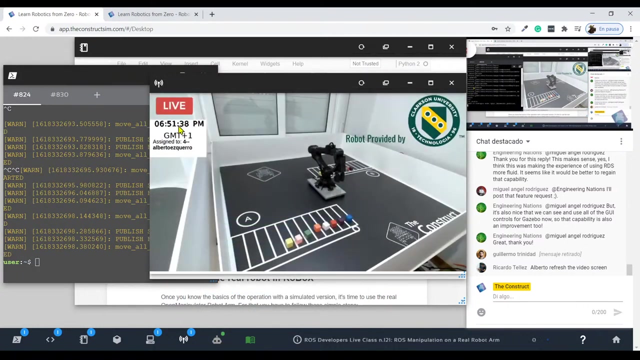 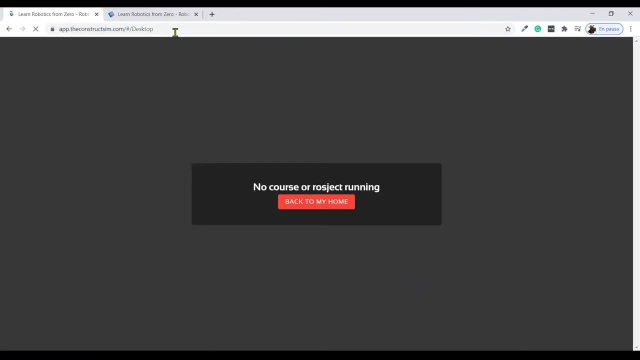 it one more time and see this is finished. let me see here. let's see if the messages are being published into the topic, but there is some more information, so let's try to close the connection and turn it on again. alberto, refresh the video screen. 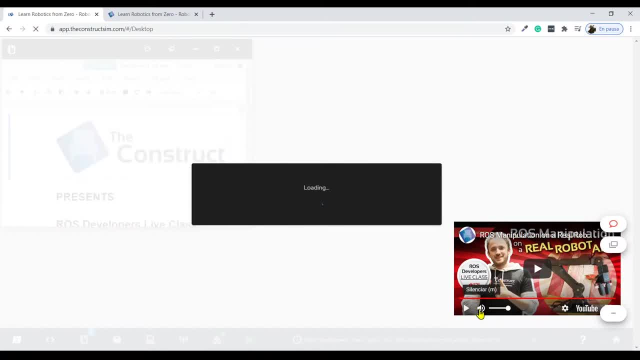 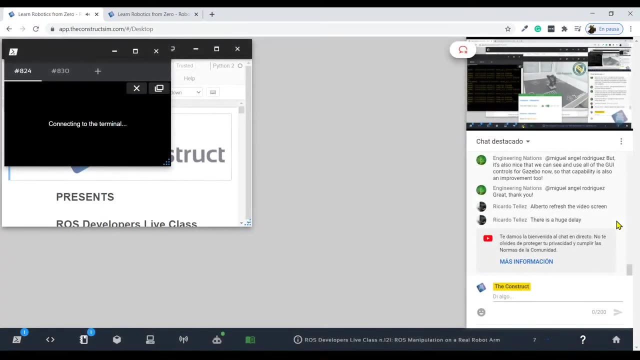 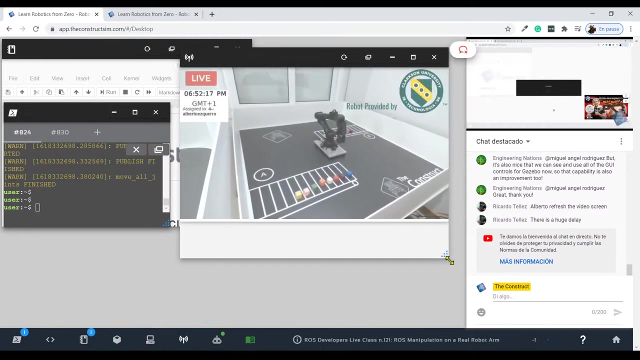 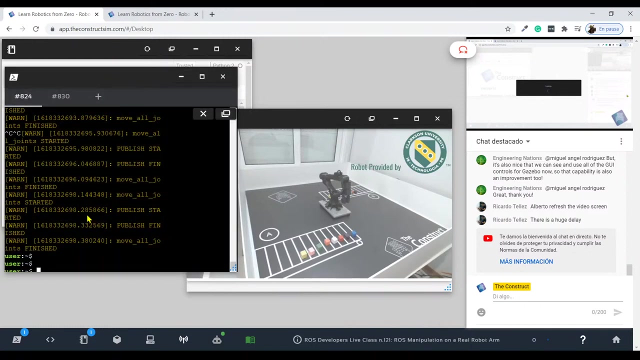 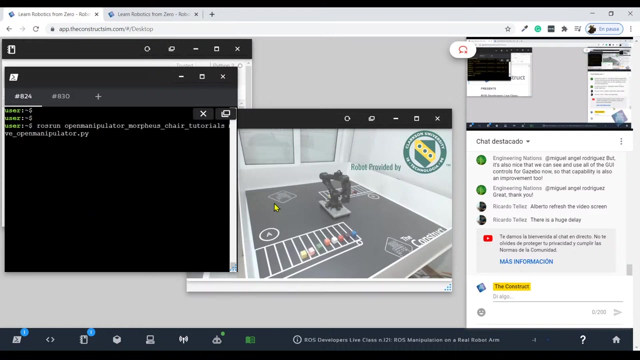 says this seems to be okay because the time is moving and everything is moving. I will put you back here. there is a huge delay. is telling me Ricardo, okay, your robot lab, okay, I have refreshed it. now this, so let me see the topics, so let me run. 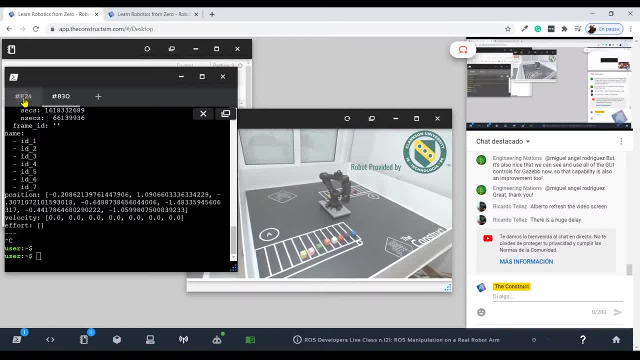 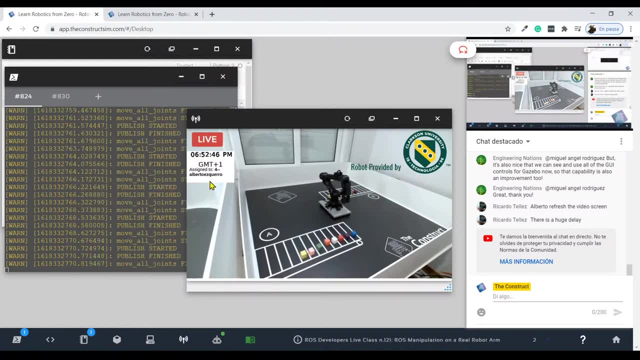 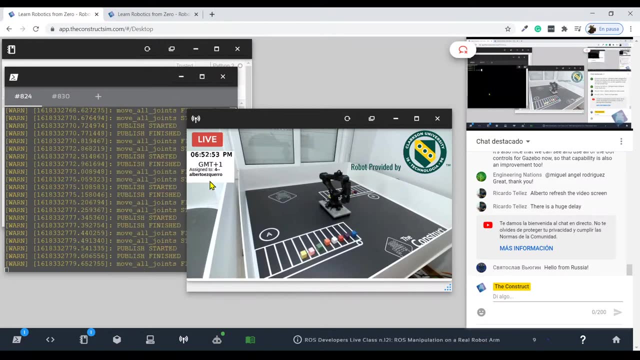 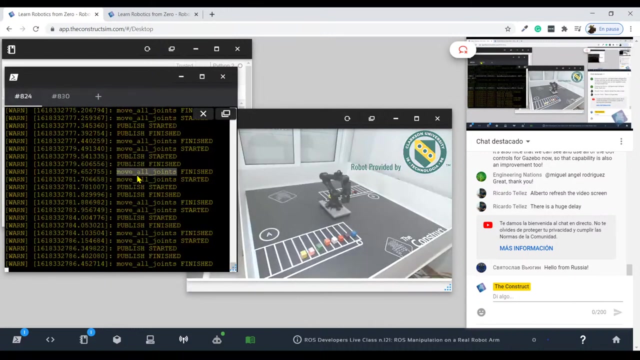 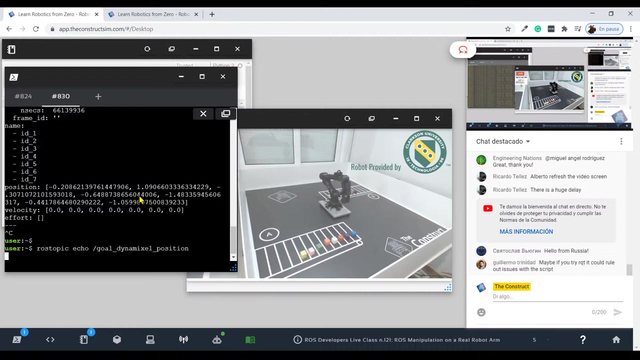 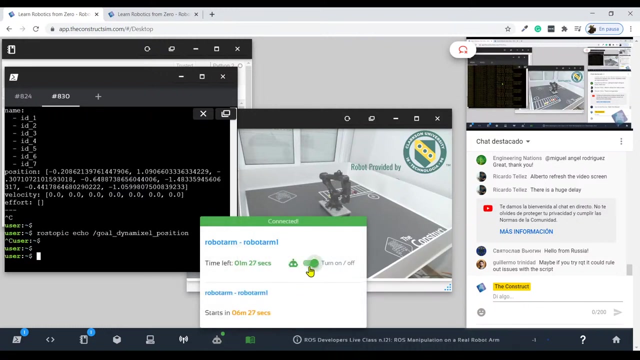 it again. maybe it's yay. everything is super strange because I have checked that the topics are not the most important topics, so I will go to the next page and I will go to the next page, and I will go to the next page and again. however, the 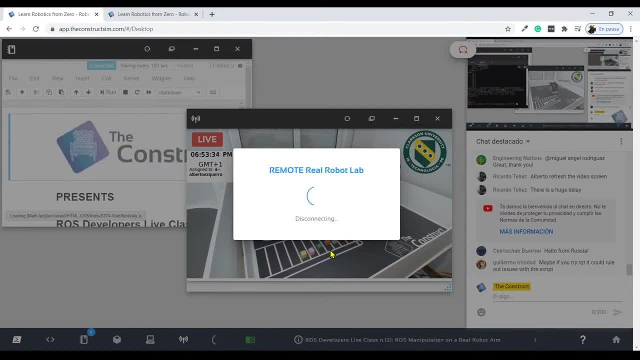 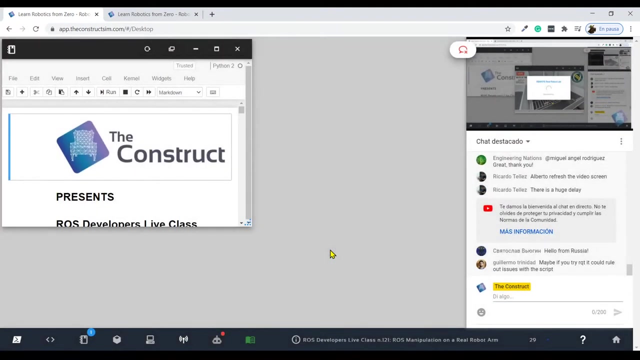 time is running out, unfortunately, but let me do it. I'm going to try to do it really, really quick and maybe by resetting the connection to show properly. okay, now I'm disconnected, but, yeah, 50 seconds. I'm going to wait for the next session, okay, which? 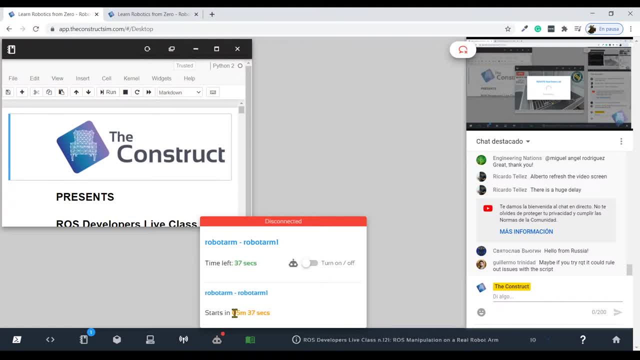 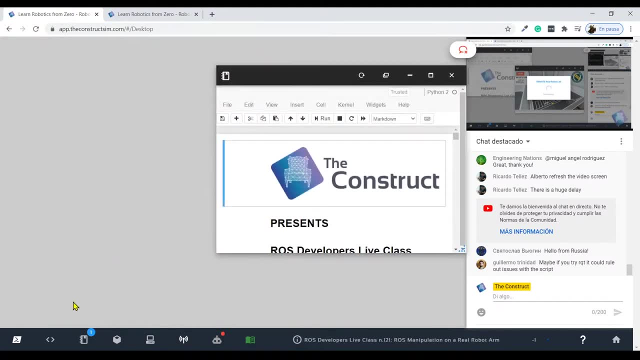 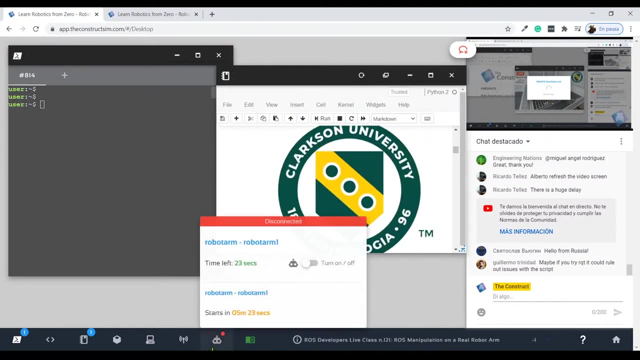 starts in five minutes. we already have some time, more or less, with the robot arm that you can also use. let me, well, let me- wait these 22 seconds until everything finishes. you might want to wait. yes, yes, I'm going to wait for the next session to do. 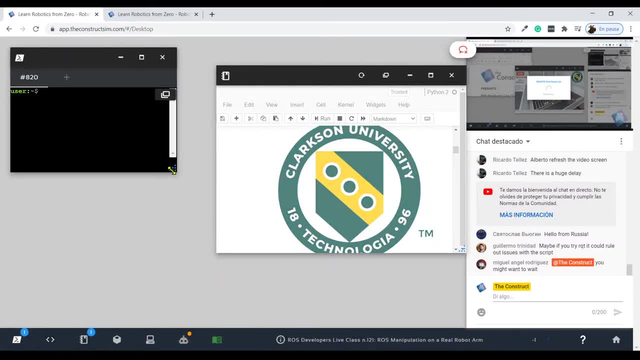 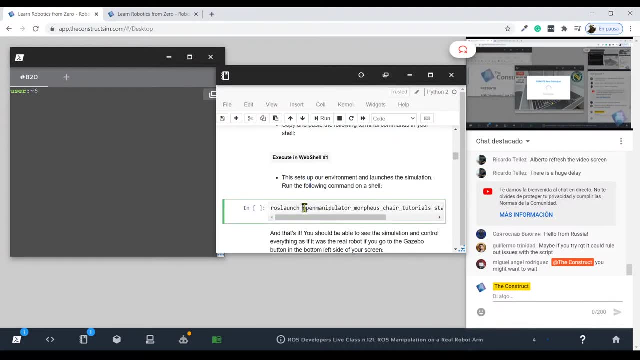 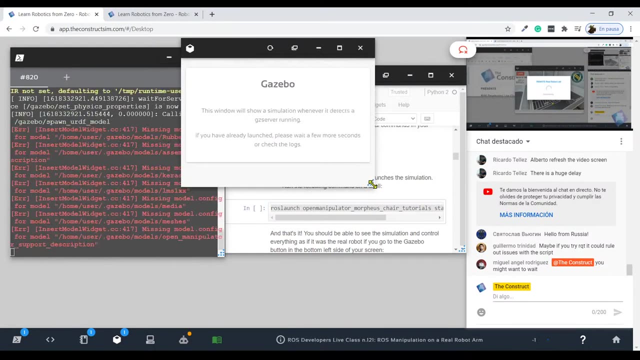 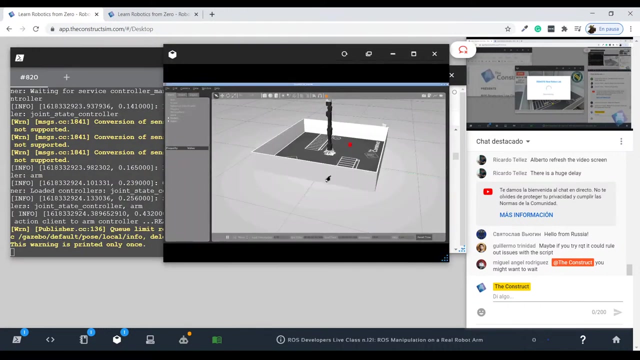 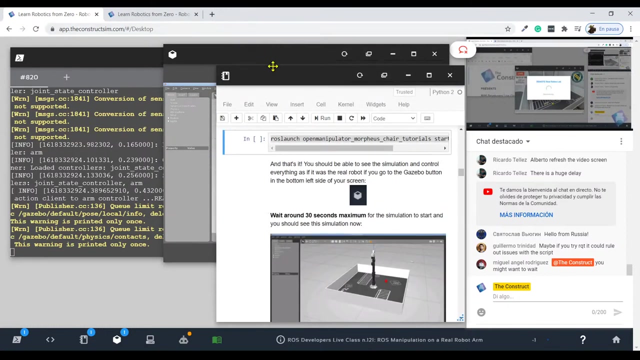 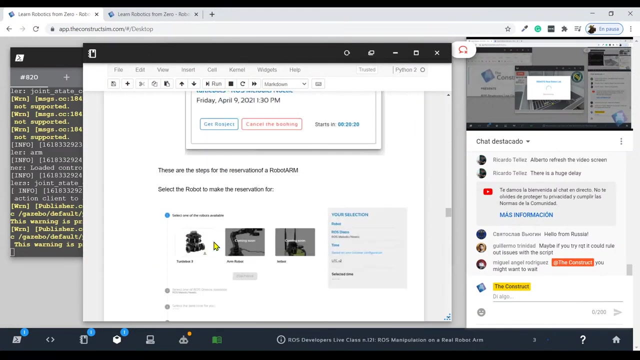 it with movie. there we go. robot session has finished it. now let me open here a new shell and very quickly, I'm going to launch the simulation. so I'm going to launch the simulation and there we go. okay, so here at the final part of the notebook. 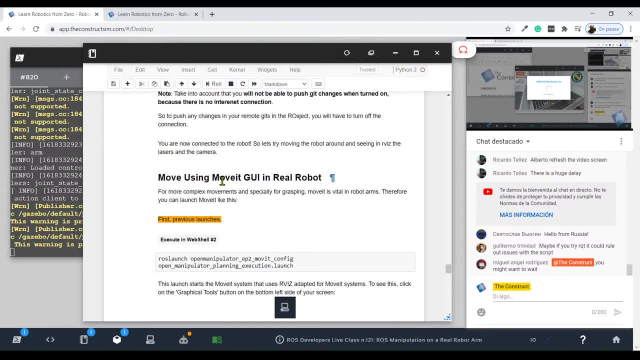 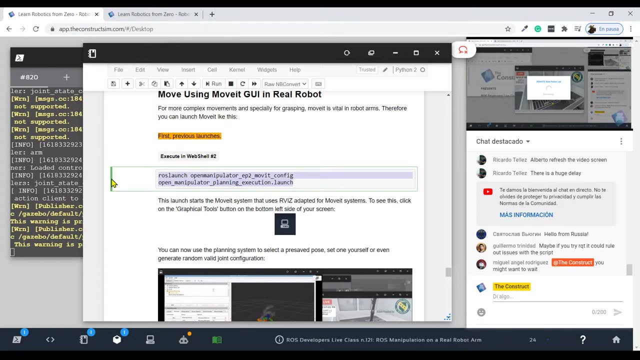 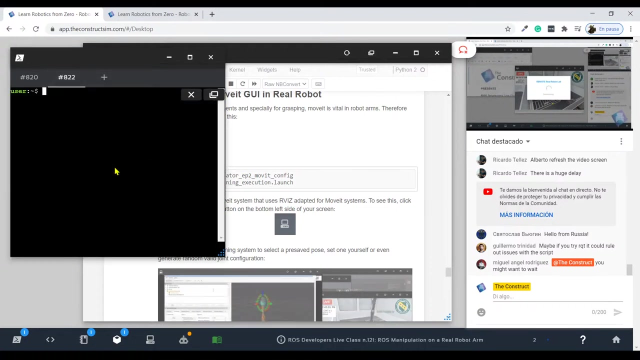 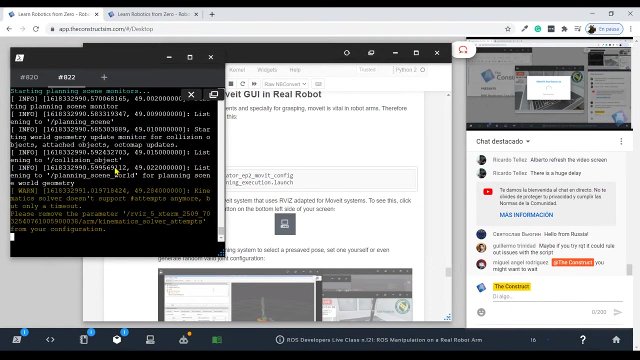 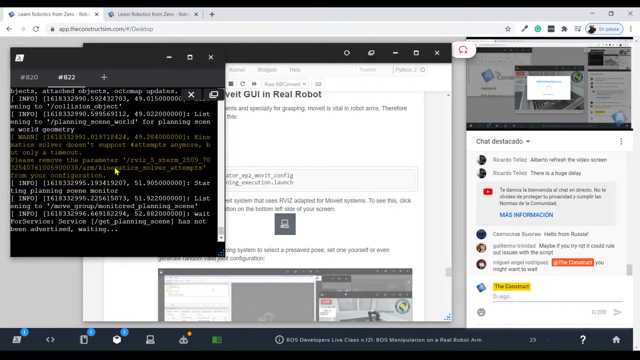 also you're going to find instructions. let me launch movie for the simulated robot and also for the real robot, and you can do it with this command. so I'm going to show it how to do so movie. basically, it's the main ROS tool, the main tool. 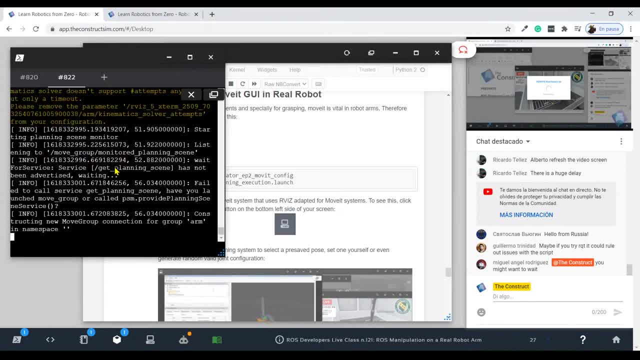 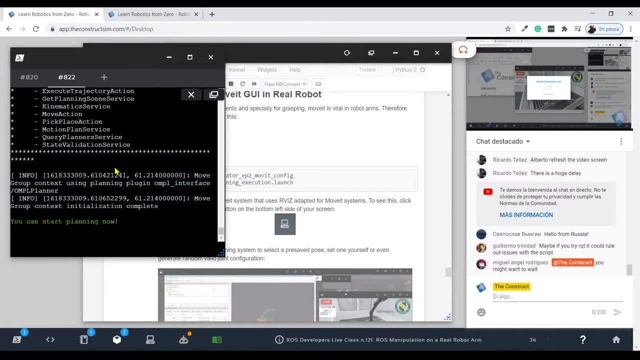 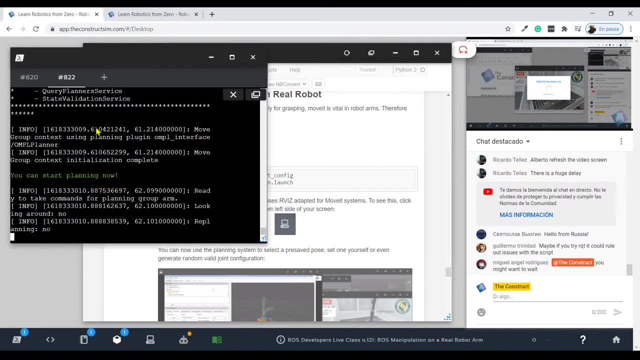 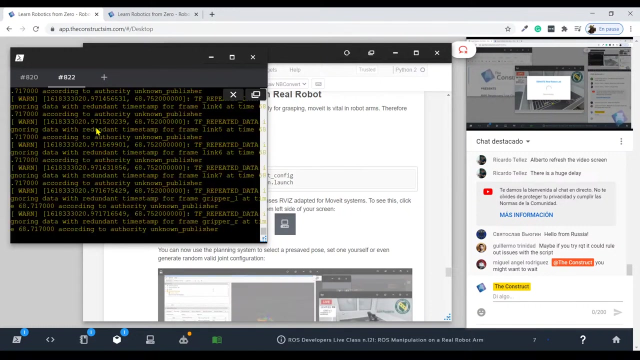 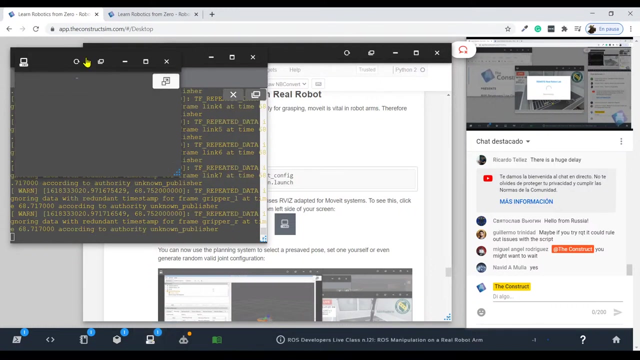 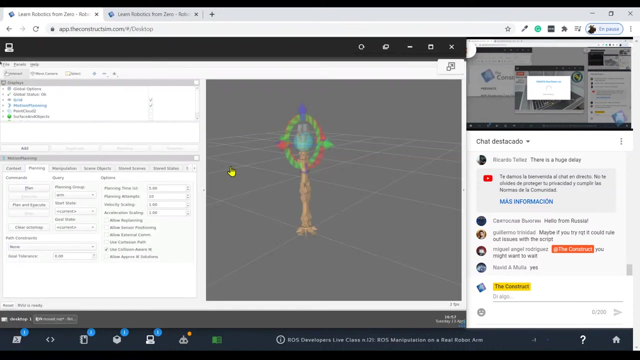 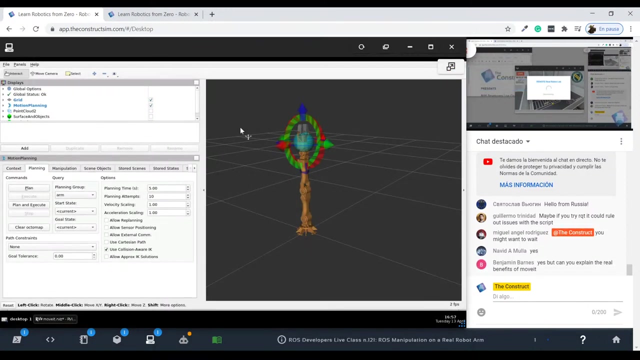 used in ROS in order to perform manipulation, so it provides a very nice looking and easy to use GUI. in order to move it, but in the same way that we did with the RQT that we launched at the beginning of the class, we need to open the. 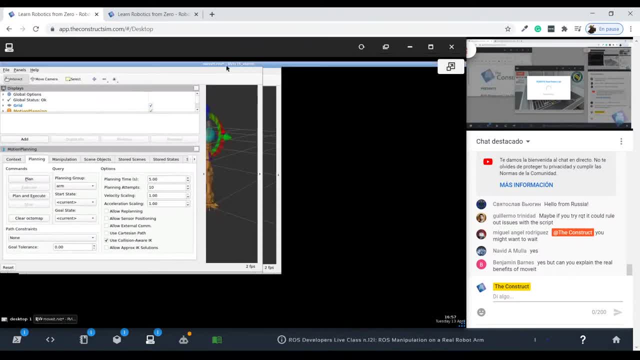 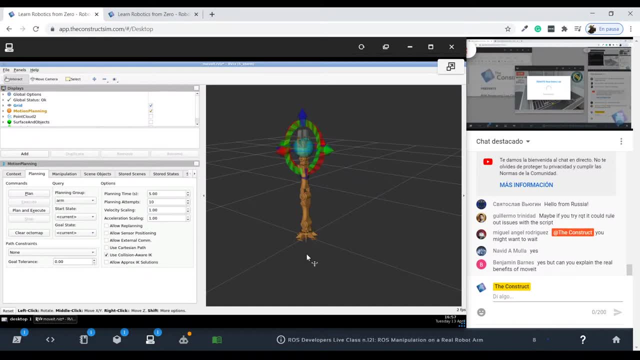 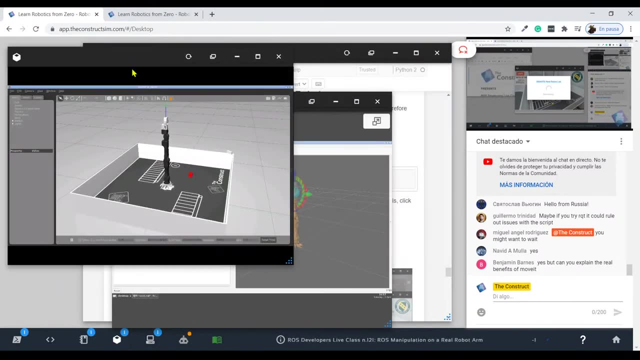 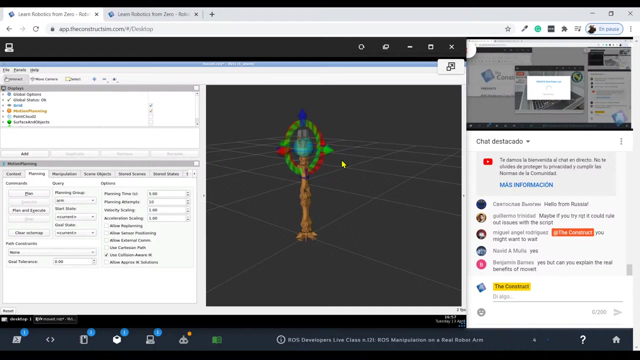 graphical tools and it's very easy to use. and it's very easy to use. so let's go to the simulation. so we have the GUI and here we can see our robot. so we could set a random goal, for instance, see, I can change to a different. 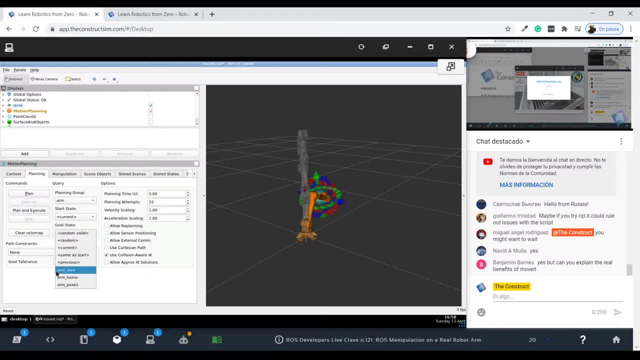 random goal. or also I have some predefined positions here at the end which are named arm zero, arm home and arm pose the end effector to a position or another. see: okay, in my case I'm going to select random valid. no, let me select this arm home. 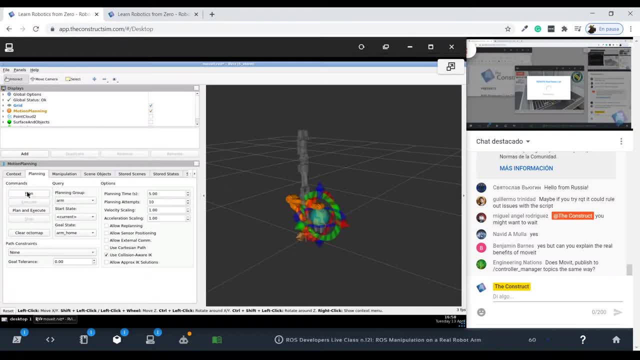 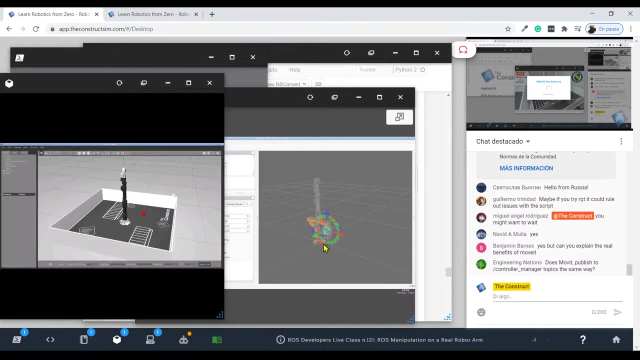 there we go. then, once you have selected a random goal, you can change the position of the joints. as you can see, it's also showing this path as a movie. it has computed a path in order to reach this goal position and the simulation you can click here. 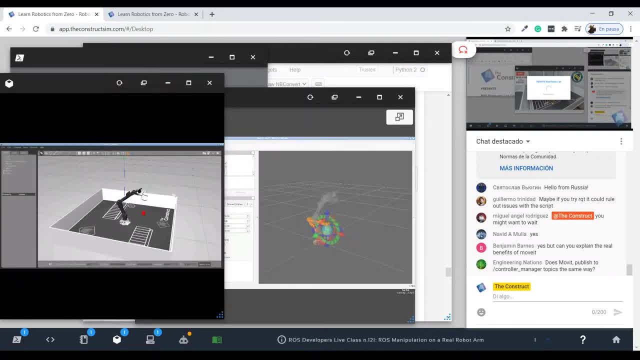 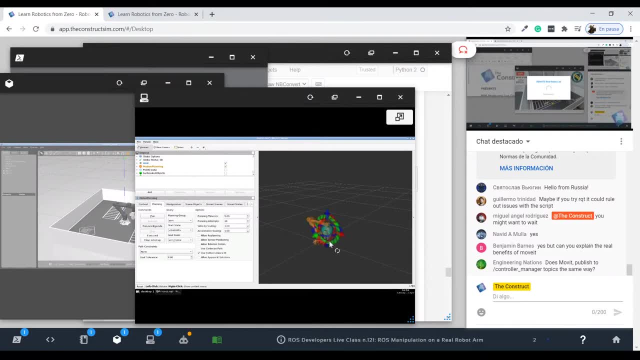 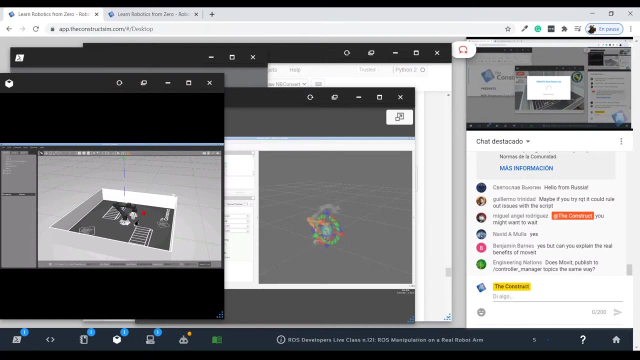 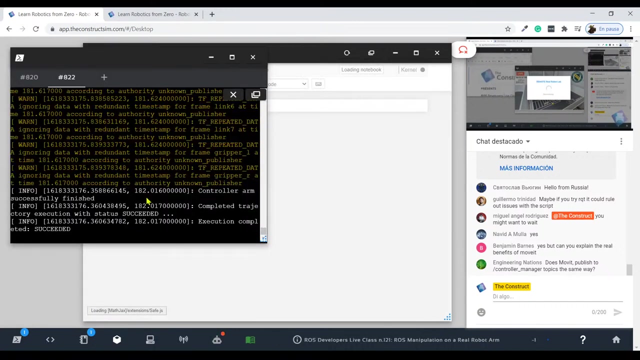 in the execute button and the motion is going to be executed, as you can see here. see the same motion that movie planet here is executed here in the simulated simulation. in the final minutes let me try to connect again to the real robot. so let's go for. 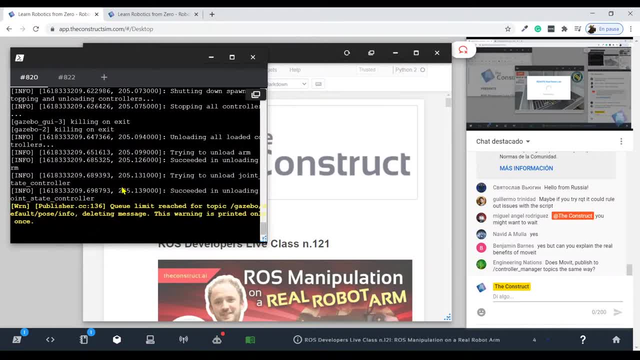 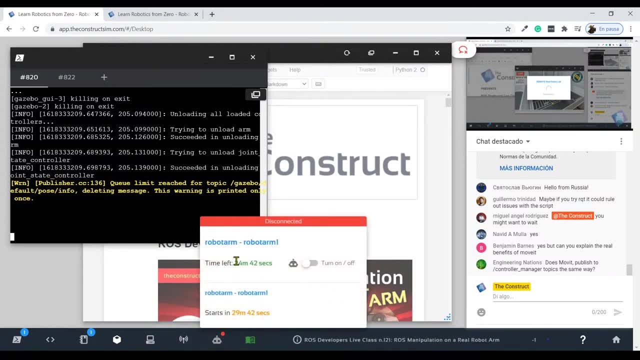 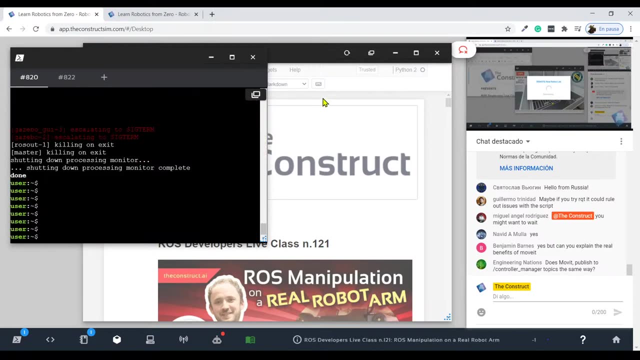 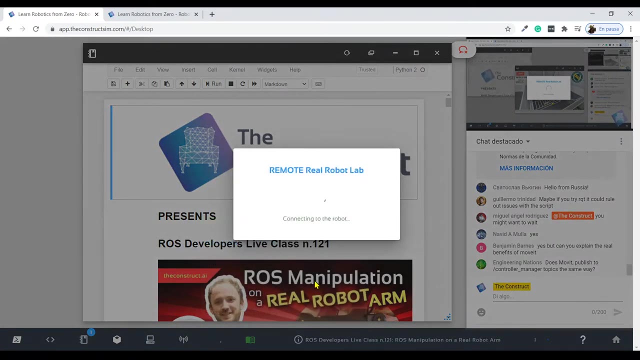 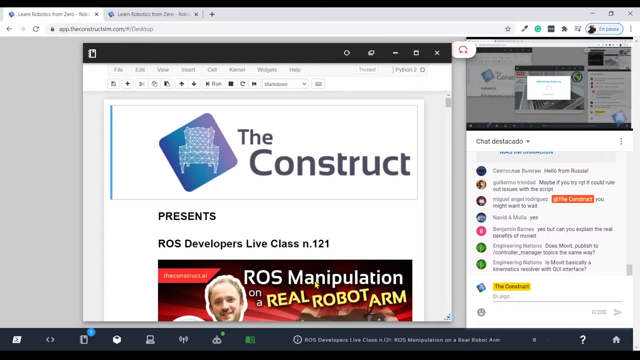 the second try. let me stop the simulation here. stop everything. my new session has started. yeah, I'm going to close the shell and let me again turn on the connection. there we go connecting to the robot. let's wait a few seconds. okay, this one has gone pretty. 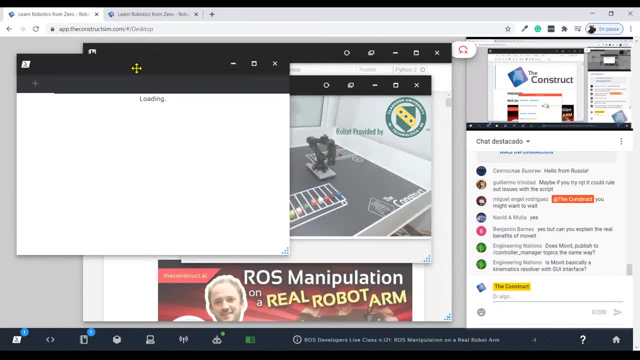 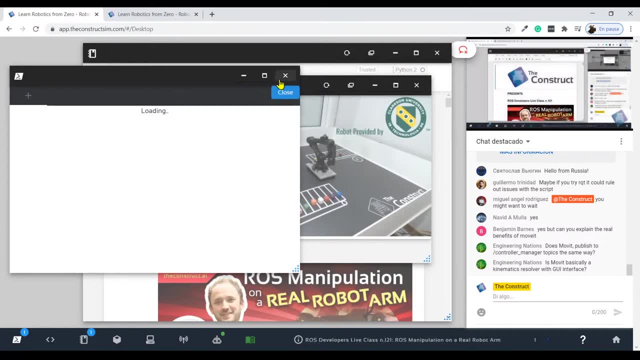 fast, so let's see how it works. not really okay, let me wait a bit. is movie basically a kinematics resolver with good interface? yes, that's it. that's it. engineering nations, that's basically, uh, kinematics over inside. you can switch from one to another, depending. 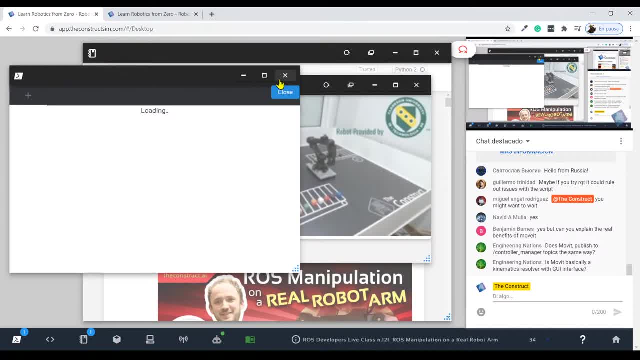 on your needs. you can even create your own kinematic solvers and compile them as a plugin and load them to move it. so it allows uh, working with kinematics and trying to solve kinematic tasks. it's a pretty hard task if you have tried to. 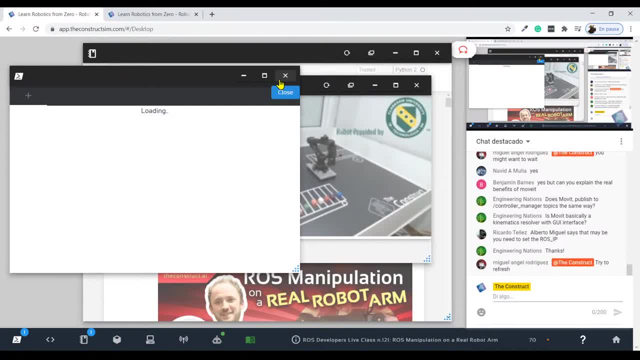 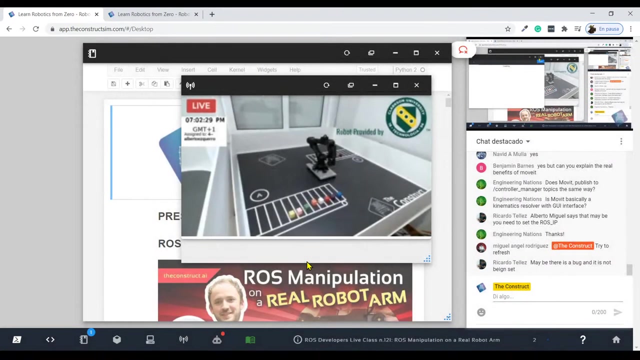 to calculate the kinematics of a of a motion. it's something that it's not easy. and movie: he can use movie. so that's the amazing thing. yeah, let me, let me stop this. i'm going to turn off and i'm going to try to connect. 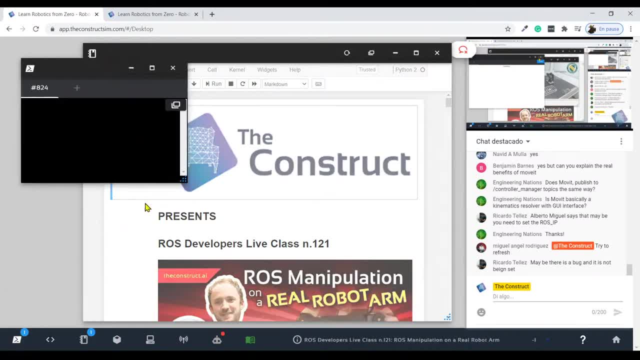 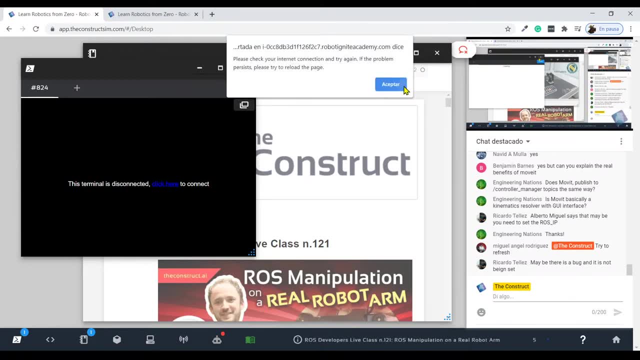 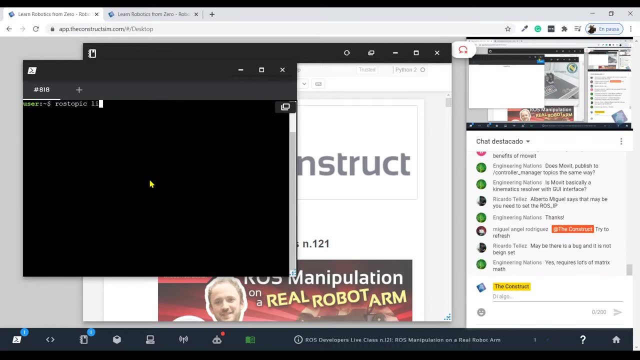 one more time and if it doesn't work, i will leave it. okay. now, in theory, i am not connected, right? so if i do, if i do raw stopping list, i shouldn't see nothing now. okay, right, because i don't have i, i don't have the 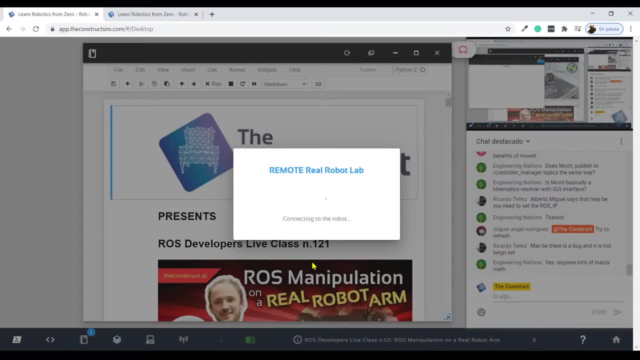 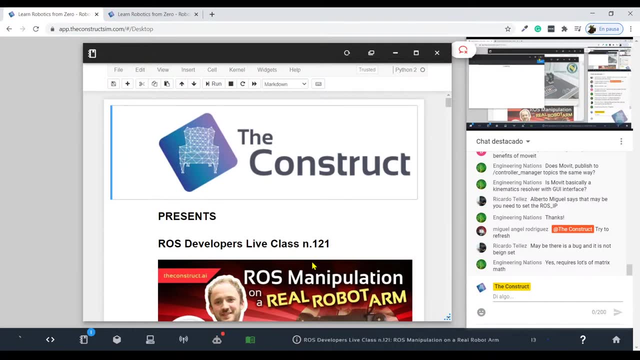 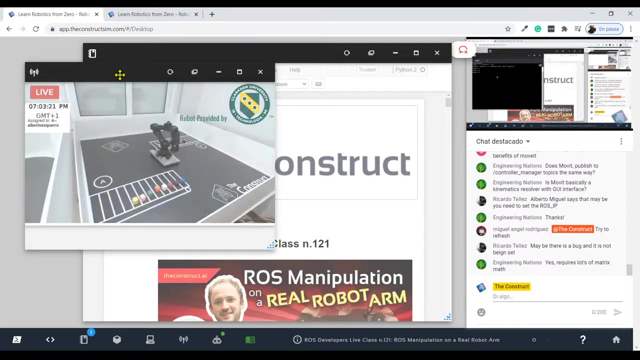 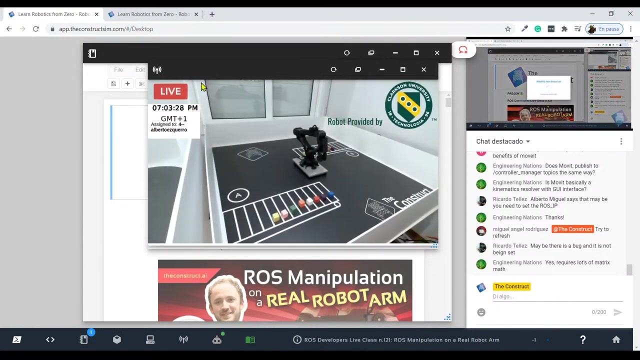 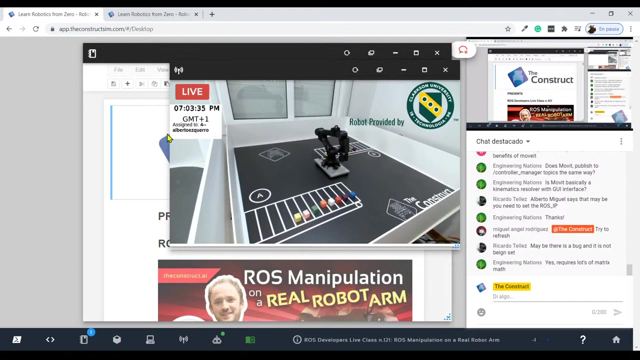 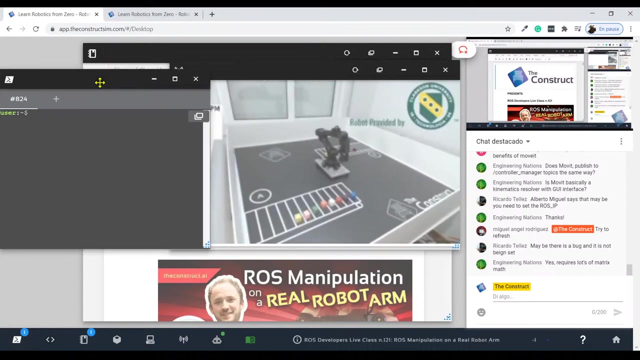 simulation and i am not connecting to the real robot, so it's normal that i don't see anything and i just wait for two seconds and and and providing a very nice good. all right, so apparently now i am connected, i can see here the robot, the, the. 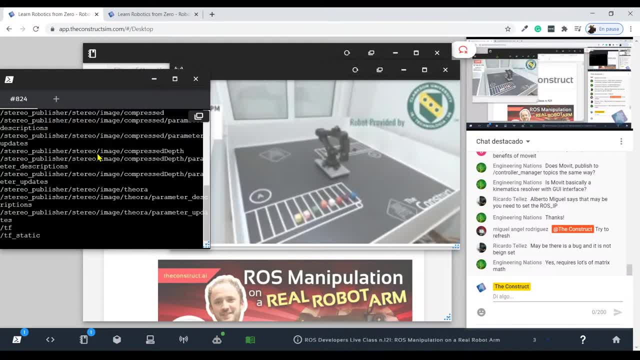 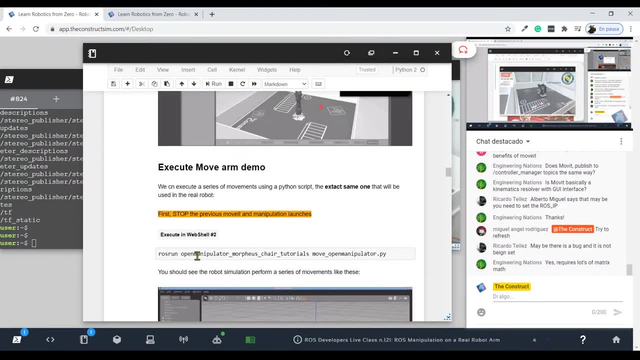 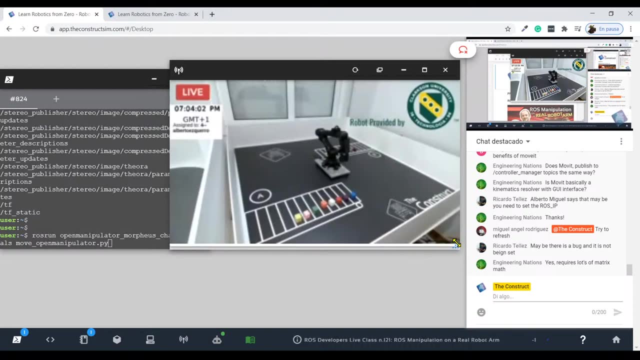 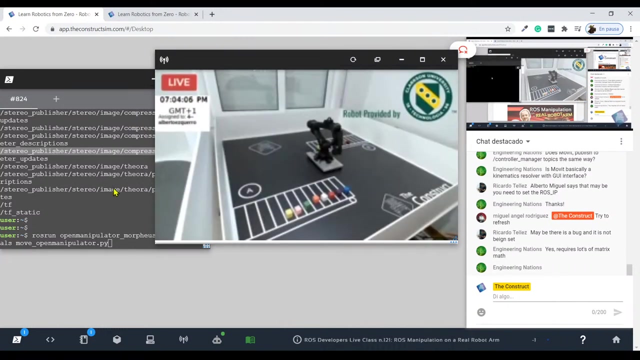 stream seems to be okay. yeah, we can see the topics, so let's try one more time to run the demo. there we go. here i have the command, here i have the robot. i have lost a little bit the quality here, but no big deal. okay, so let. 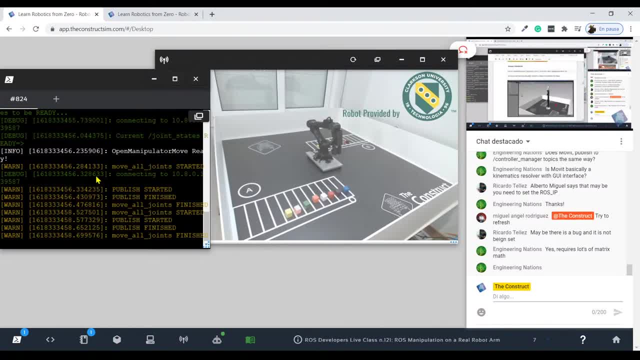 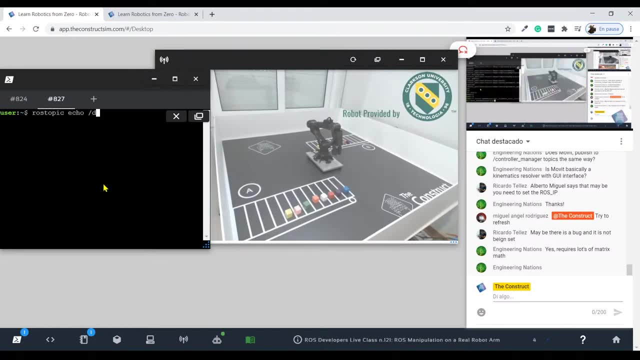 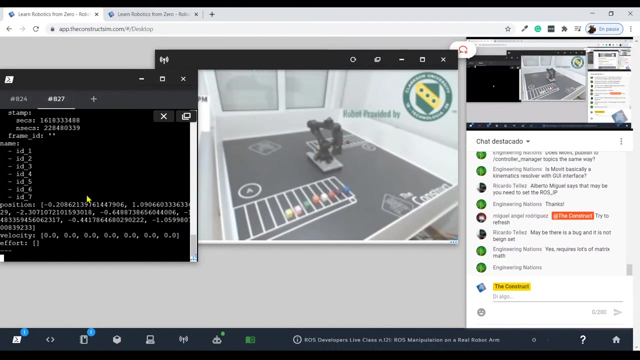 me run my script one more time. let's see: the messages are being published. yes, the messages are being published, but the robot is not moving. okay, so some try to refresh. is suggesting, miguel, the messages are being published. okay, let me try to refresh one time and see. 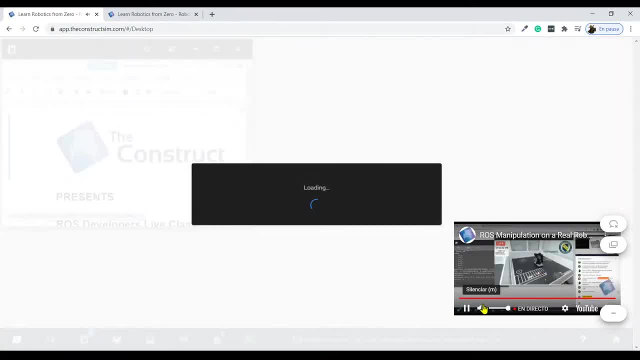 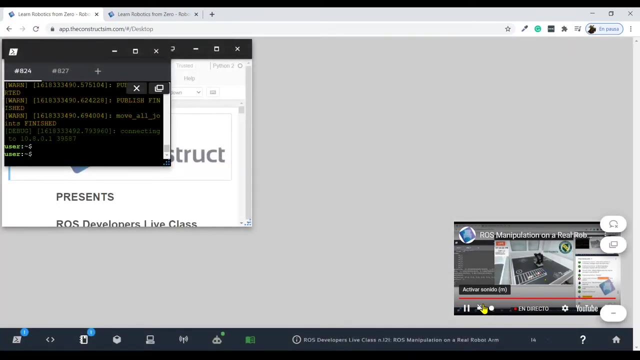 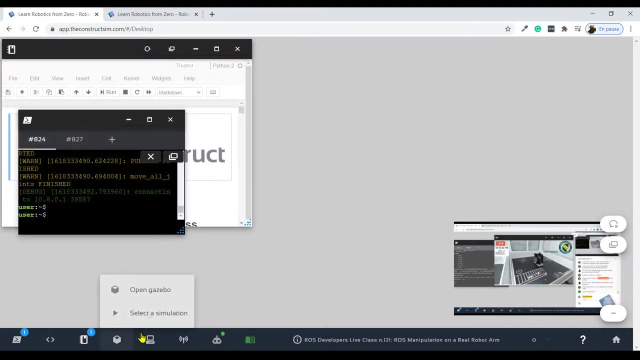 if it works and if not, unfortunately, we will leave it here without being able to test the real robot part. however, let me tell you that, even if, okay, i cannot see the chat now, however, let me tell you that, even if i don't manage to do it, okay. 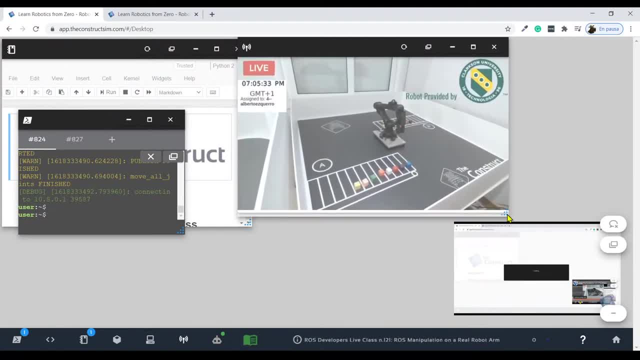 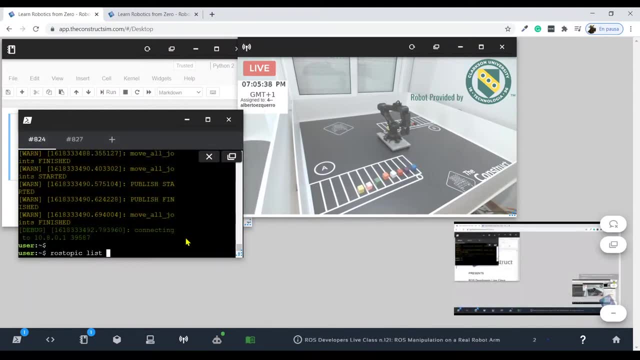 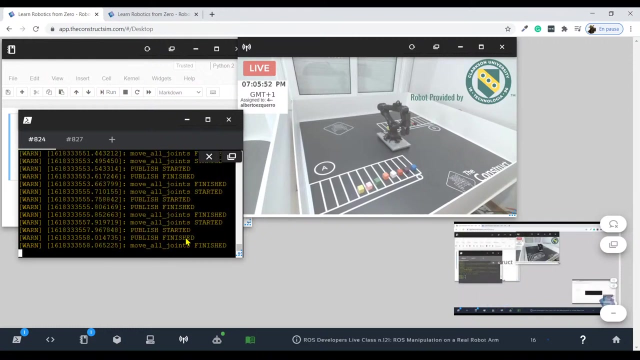 let me open the streaming here. refresh- okay, here we have the robot. let me make sure that the connection is there, okay, yeah, i can see the connection one final time and see if it works. yes, so all the all, the, the ross connections and everything seem to. 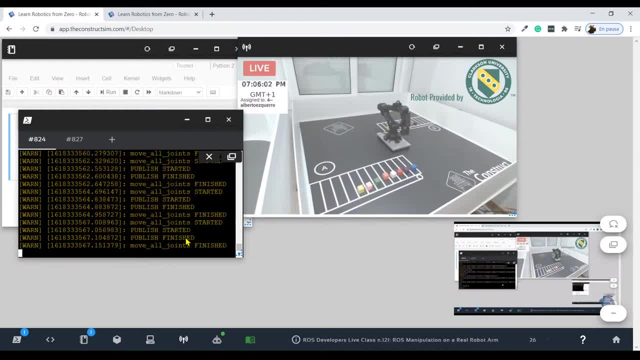 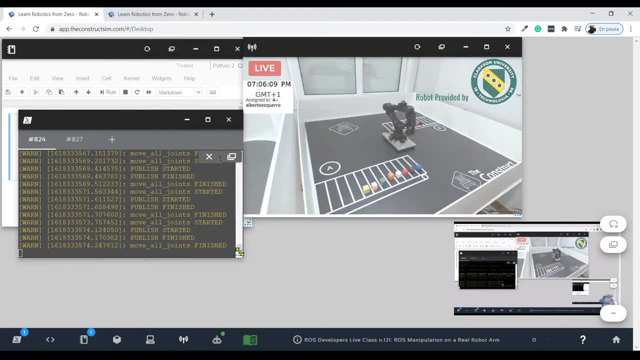 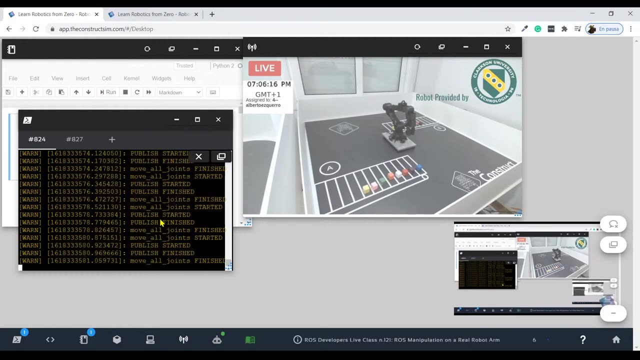 be fine, the pro the pro. the program is running fine. it is connecting to the topic, it's publishing the joint state messages, probably some kind of. let me tell you that i have just tested this 20 minutes before the live class and it was working, so something. 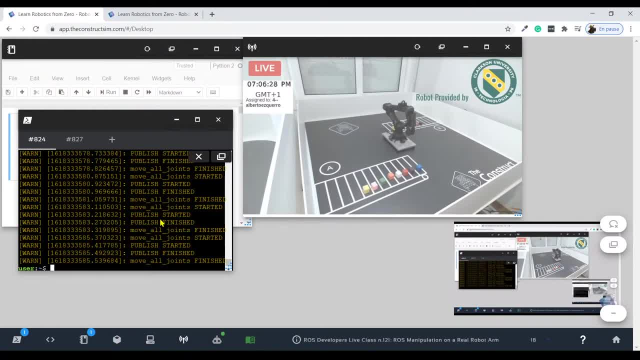 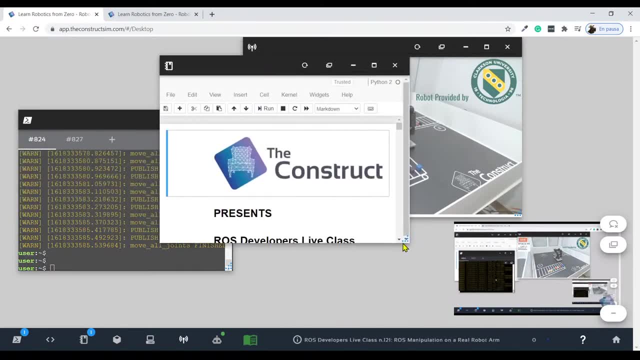 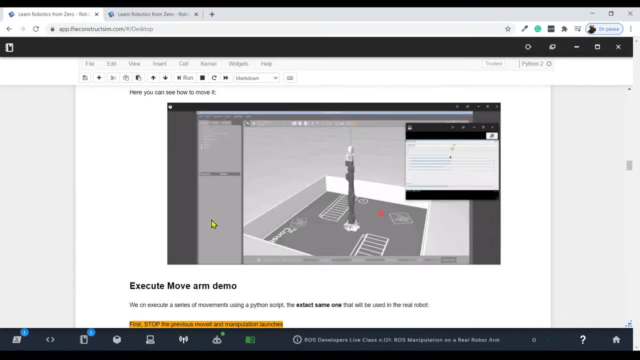 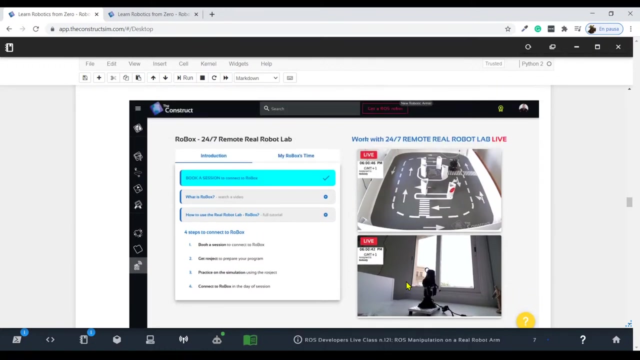 must have happened some strange book or the very well-known live course, live demo course. okay, um, okay, so let me close it here then. yeah, so let me tell you that, even though it has not worked in this live class for some reason, i don't know exactly- 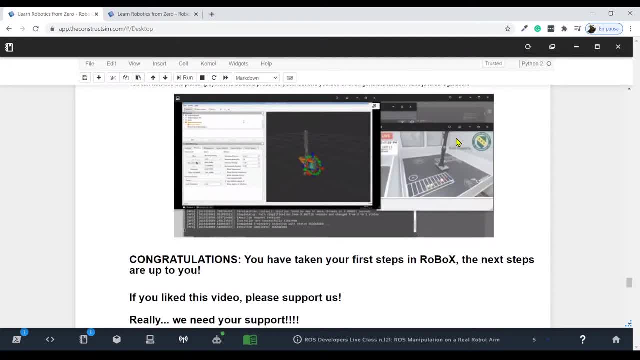 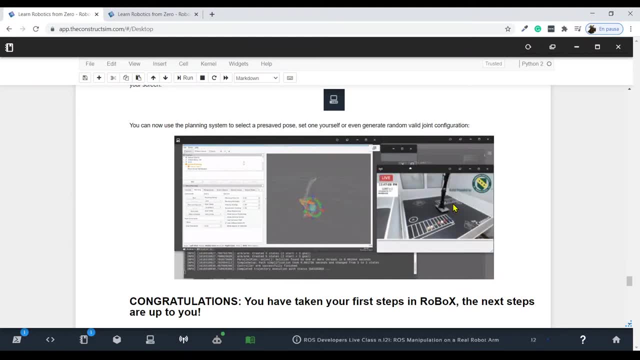 how it works. but let me tell you that, even though it has not worked in this live class for some reason, it is going to be working for sure tomorrow. okay, so everything i i have said is i have said at the beginning is still up. so tomorrow we 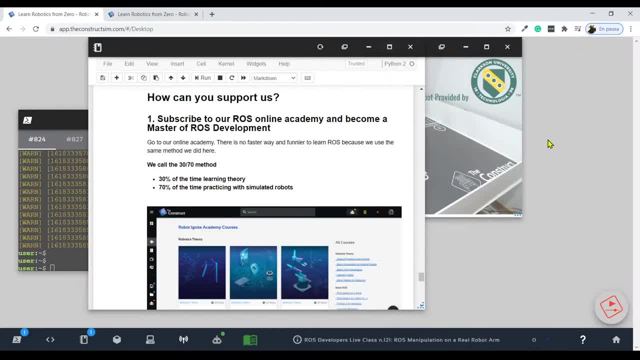 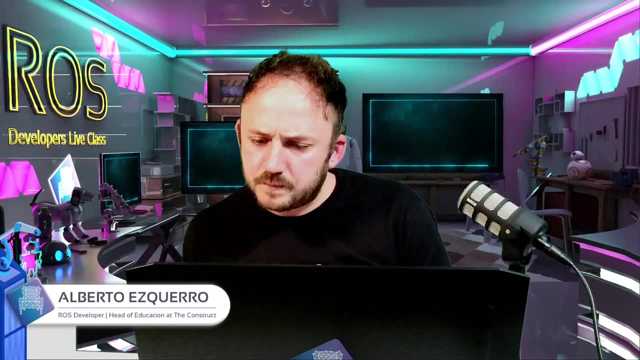 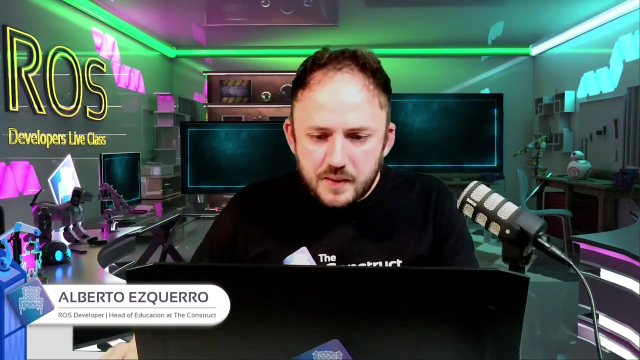 are going to activate this and you are going to be able to connect and test the connection and everything yourselves. okay, let me. let me, by the way, check the ros ip. okay, there we go, here, i am okay. check the ros ip. okay, let me do this, ros ip. 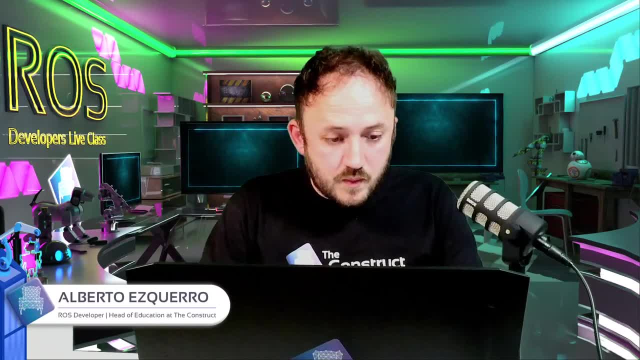 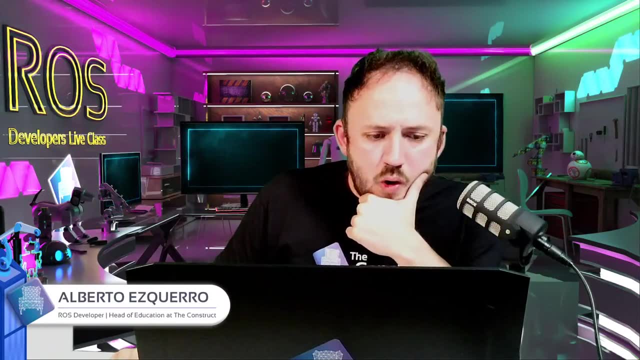 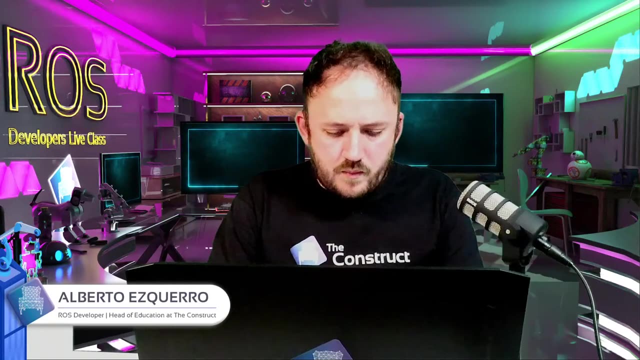 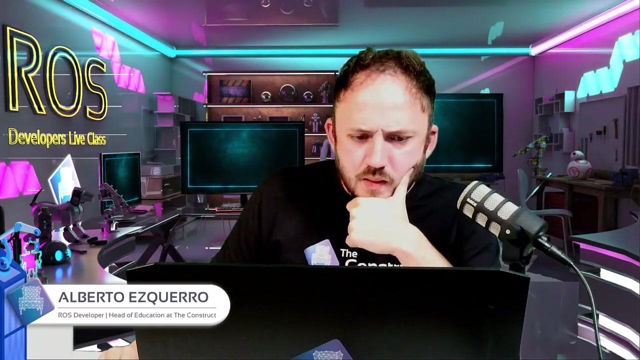 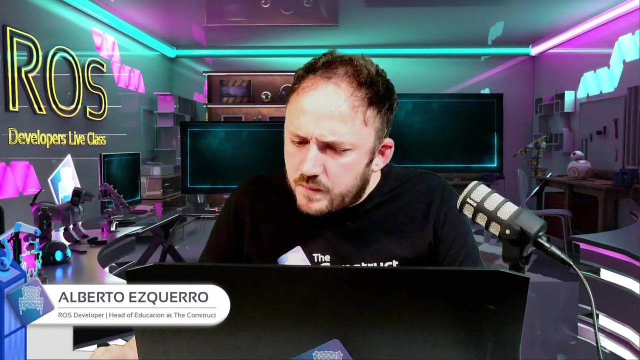 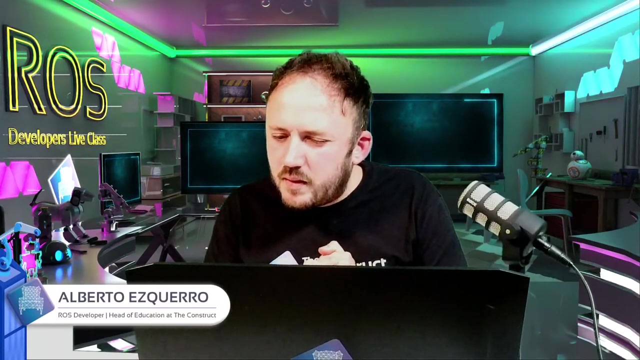 10803 and i am going to be going to the ros ip 10, 8. I think it is right, or I think it is right the ROS-IP. right guys? Miguel maybe can tell me, but I think it's right, the ROS-IP, if I don't remember wrong. 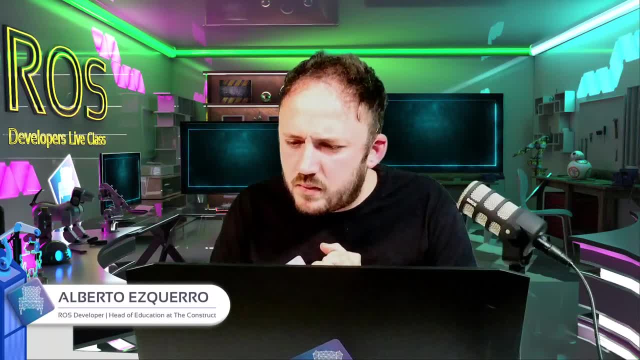 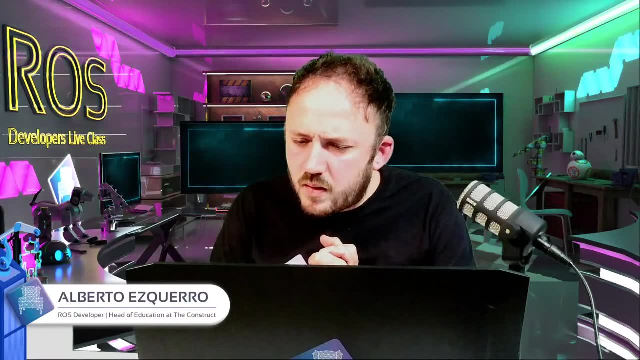 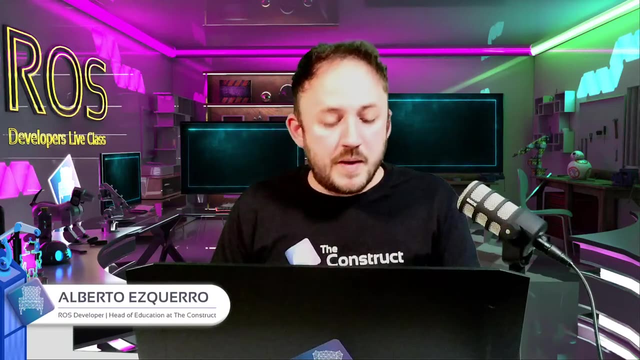 it was this one. yes, no, Miguel or Ricardo. can you confirm me Then? it's okay, okay, it's okay, Yeah, okay, don't worry, Yeah, let me. oh, yeah, I'm not sharing the screen. yeah, sorry, 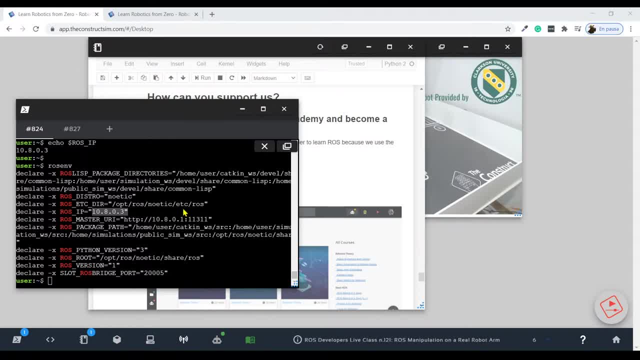 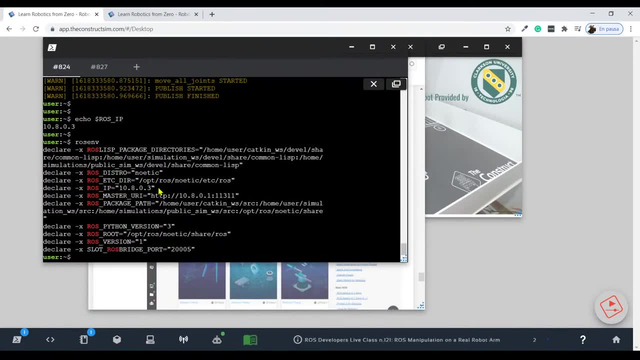 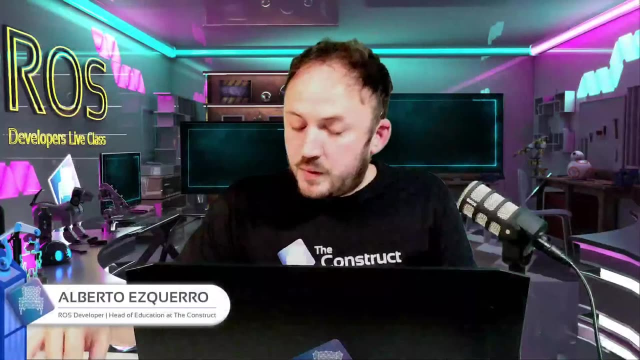 Yeah, I was checking here. let me show it. I was checking here the IP and it. It seems to be okay. yeah, We have the ROS-IP here set to 10803, so apparently it's okay. Well, don't worry. so yeah, everything I have said is still up. 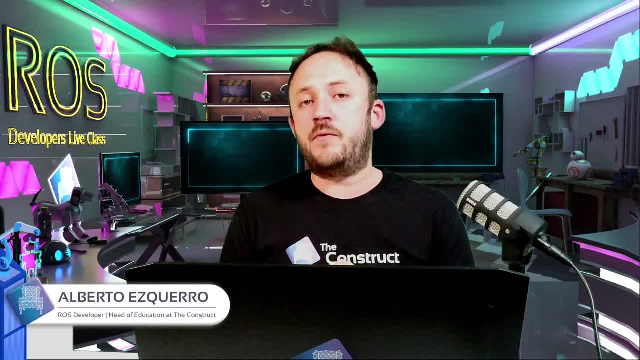 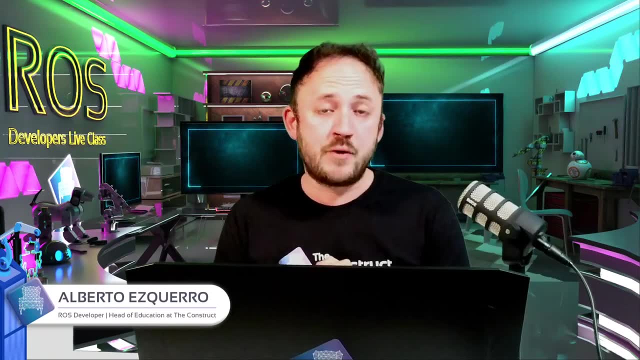 So tomorrow we are going to activate this option for all of you. so from tomorrow until the end of the week, you are going to be able to connect to the real robot and you are going to be able to use the manipulator robot. okay, 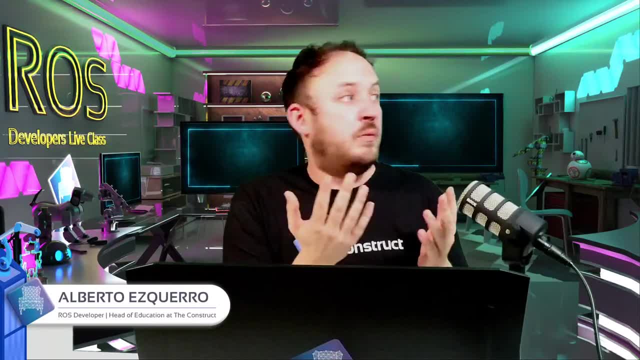 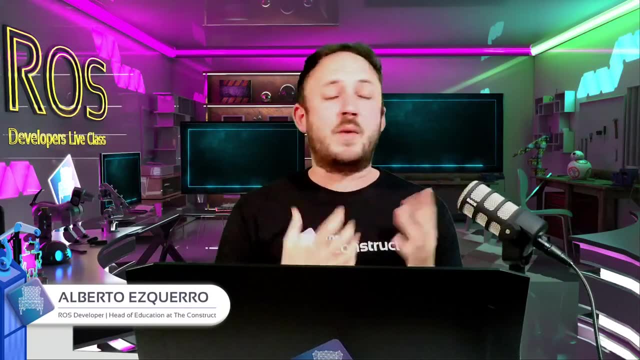 And it's going to work. Yeah, we are going to fix it and now we are going to check what was happening, but I can tell you that 10 minutes before starting the live class it was working. So we are going to see what happened and fix it so that it's going to work for tomorrow. 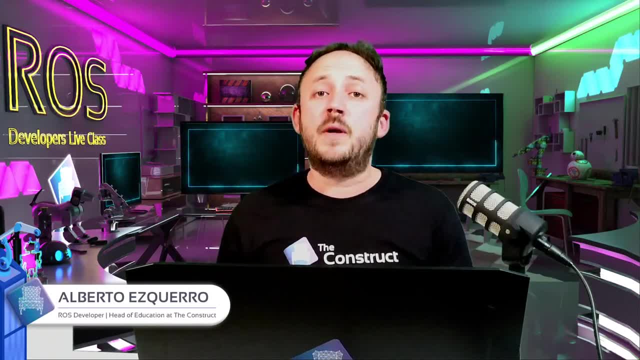 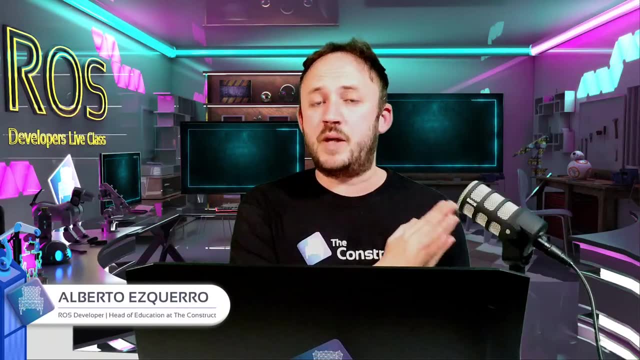 and until the end of the week, you are going to be able to book two sessions completely for free. okay, You can choose between the manipulator robot, the Clarkson manipulator robot or the Tattable 3.. So, yeah, that's all for this live class. 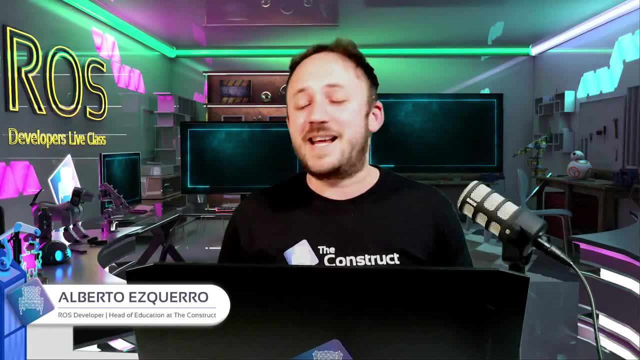 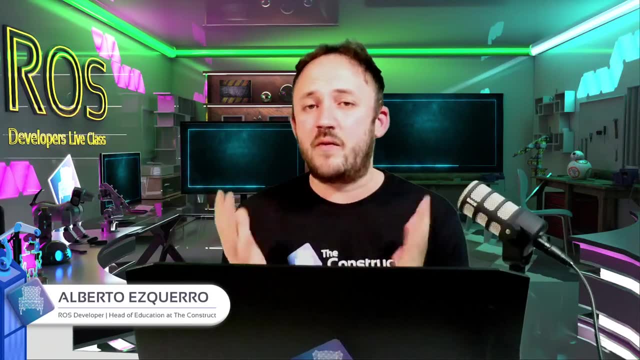 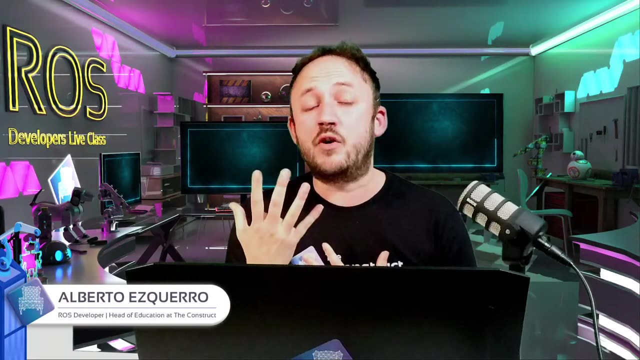 Thank you very much for being, Thank you very much for being here with me. Unfortunately, the last part, which is the real robot connection, didn't work, but I hope you got an idea of everything and I hope, I really hope- that you are. I have encouraged. 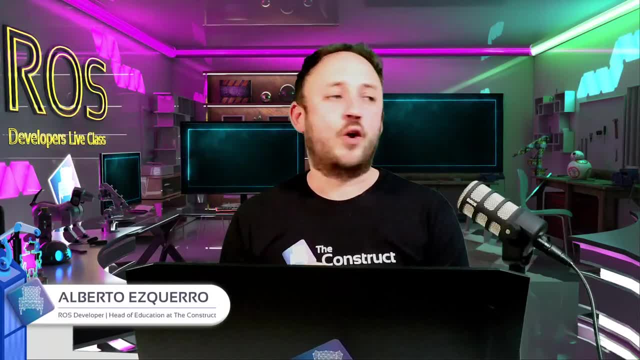 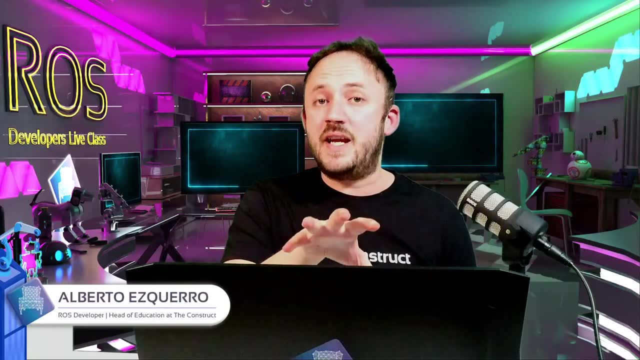 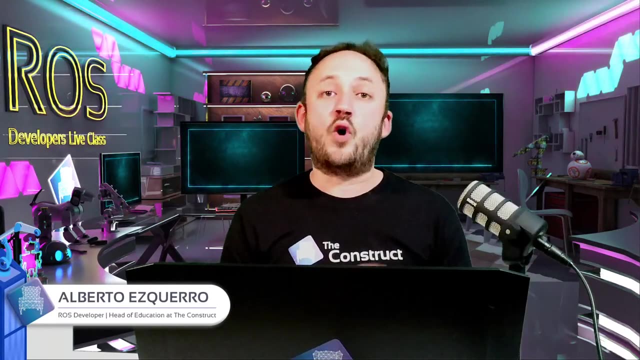 you to try it yourselves, so that tomorrow all of you go there and book a session to test all of this and to test these algorithms that we have seen today in the live class. You can test them in the real robot, Check and verify that they are properly executed also in the real robot, not only in the simulation. 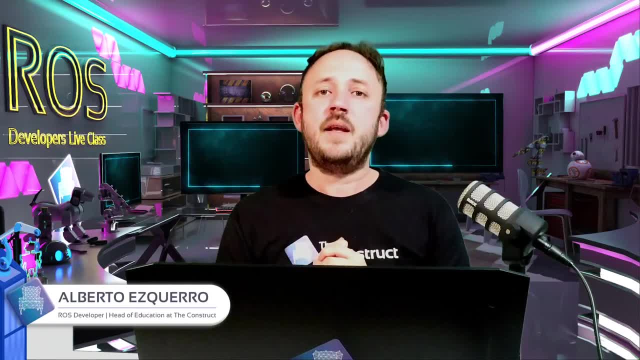 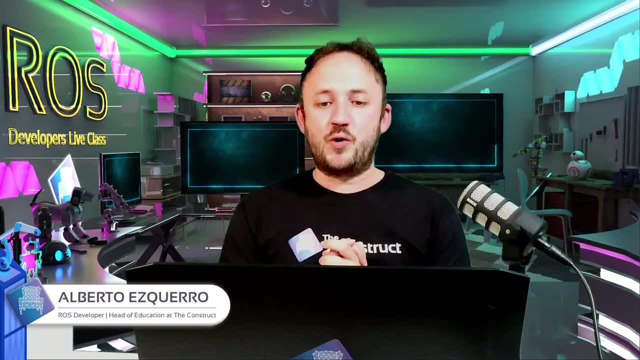 You can also test MoveIt, of course, and see how MoveIt works, test different motion plannings, et cetera, et cetera. So, yeah, guys, thank you very much for being here with me and I will see you, not next week. 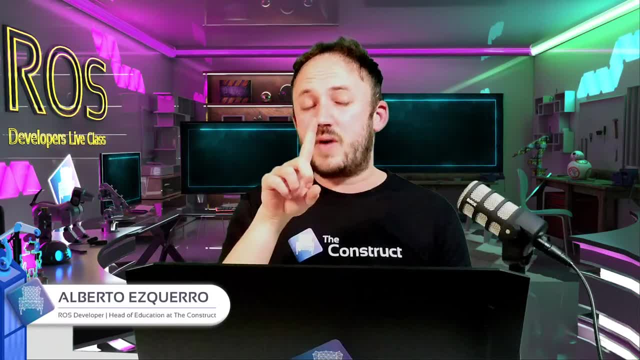 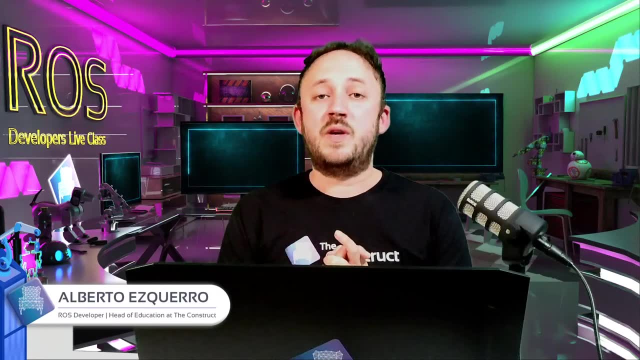 So let me tell you that the next week We are not going to have a live class, but the next one, all right. So next week, and we are not going to have a live class, so I will see you in two Tuesdays. 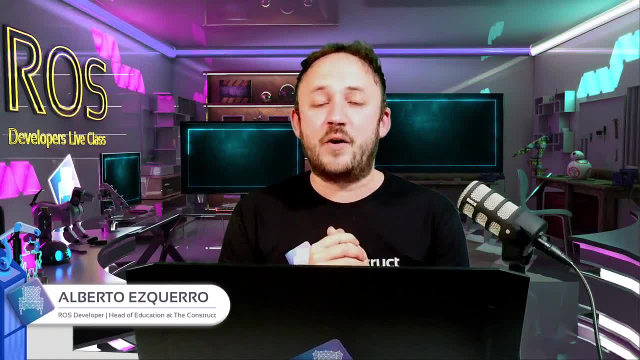 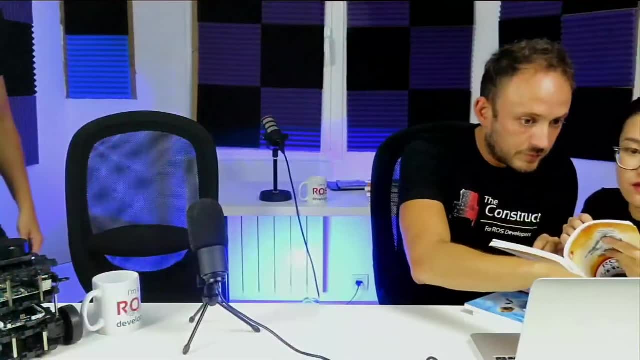 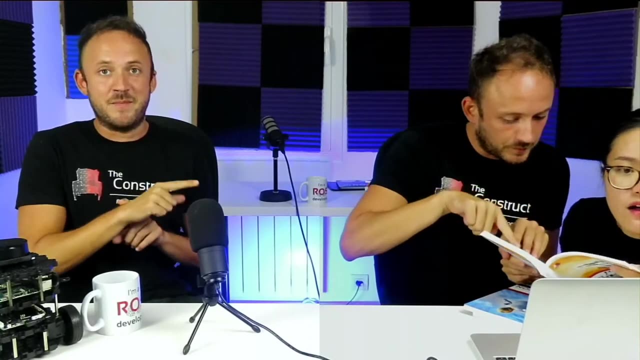 and until then, as always, take care of yourselves and keep pushing your ROS learning Bye-bye. What are you doing, Alberto? I'm training this intern with ROS. Did you have the same experience, Spending too much time Equipping your team with ROS skills? 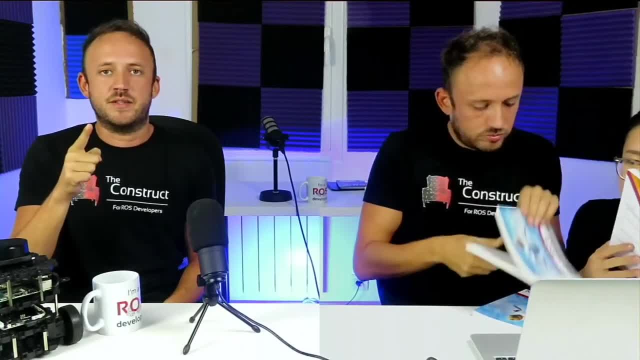 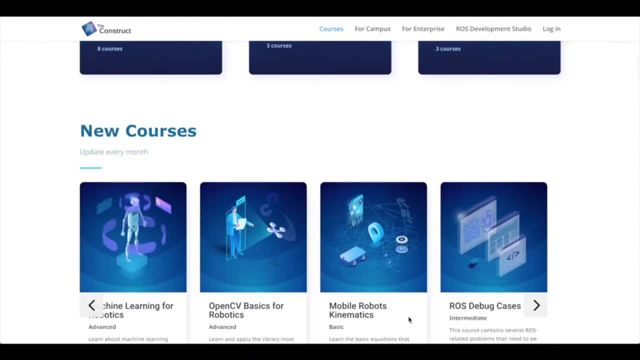 Check out our ROS online training solution for enterprises- a fast and easy way to empower your team with ROS. From ROS basics to manipulation perception, AI, ROS2,- everything your team needs to learn is here. Practice with real and simulated robots.